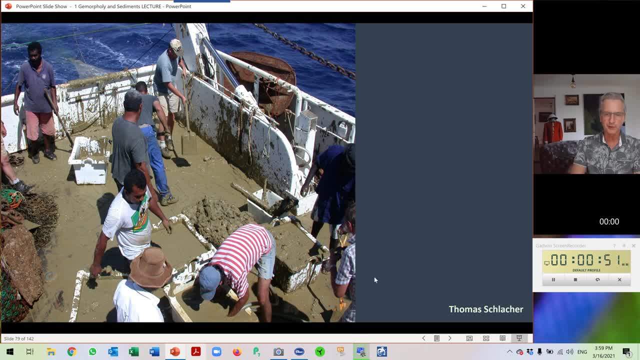 Well, the reality is- I hate to disappoint- This was my very first exposure on the very first day of taking a deep sea sample. You can see there was a bit of a rock slip up here, But we towed a big beam drill and it just filled itself completely up with mud. 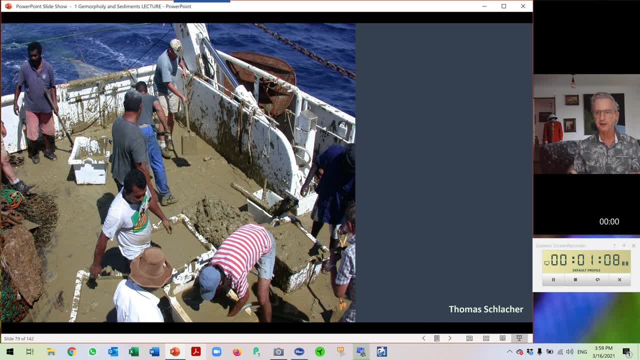 And this is something which repeated itself day after day after day after day In the middle of the Pacific. that was between Fiji and Tonga, Never mind, That is the reality. And So you might say, oh, this is not so much for me. Well, let me show you two videos from our friends on the Monterey Bay Aquarium, which very nicely illustrate how exciting life on mud in the deep sea can be. 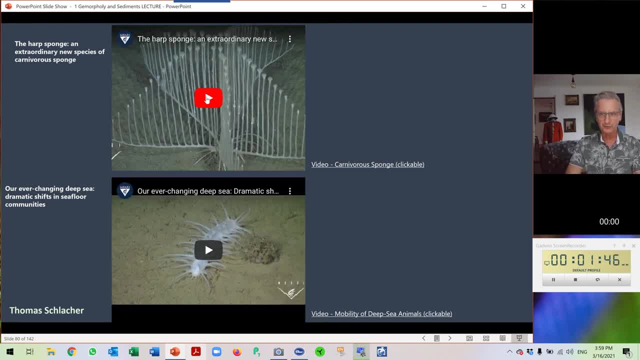 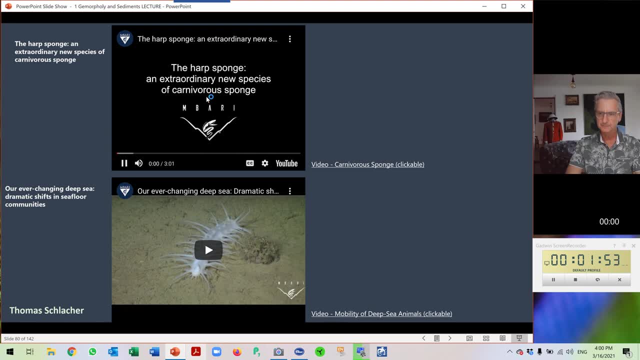 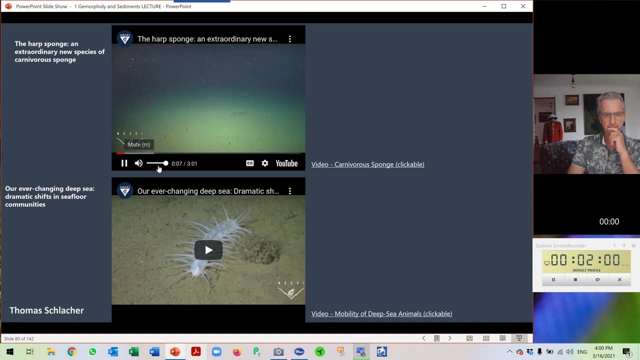 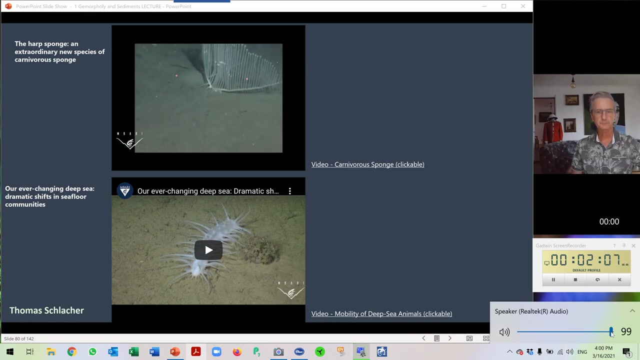 The first one actually deals with a sponge which eats other animals. It's a carnivorous sponge on the deep sea. The second one is a deep sea turtle. Scientists from the California Academy of Sciences, the University of Victoria, the Koyotan Marine Laboratory and the Monterey Bay Aquarium Research Institute recently described an extraordinary new species of carnivorous sponge named Chondrocladia lyra, or the harp sponge. 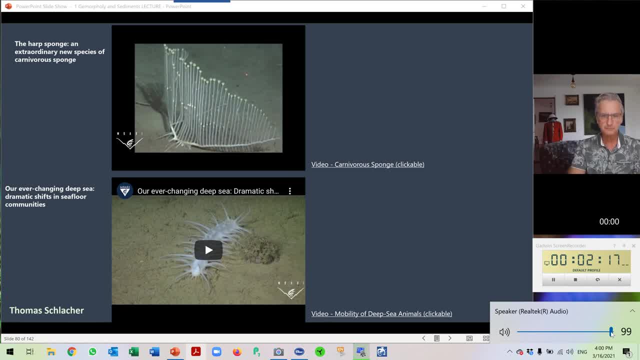 Rather than filtering water for food, as most sponges do. carnivorous sponges ensnare animals. The sponges then envelop and digest their prey. The enclosed and partially digested crustacean prey were observed and embedded in the tissues of the sponges we collected for this study. 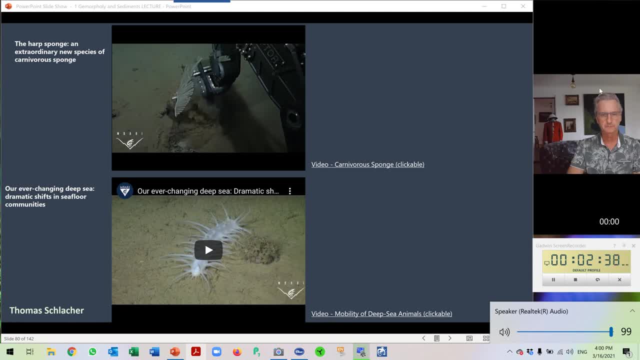 Ambari's remotely operated vehicles, Hibiron and Doc Ricketts were used to collect two specimens of the new sponge. We used these specimens, along with video observations of 10 other individuals, to describe the unique morphology of this sponge and how these individuals were linked together and how they were related to each other. 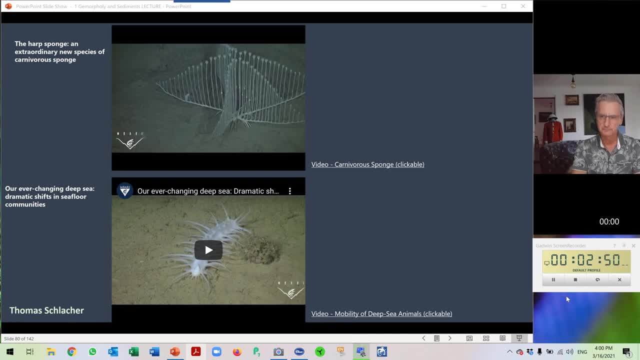 The first one is called the Chondrocladia lyra. The second one is called the Chondrocladia lyra. The third one is called the Chondrocladia lyra. and to characterize the habitat and environment where it lives. 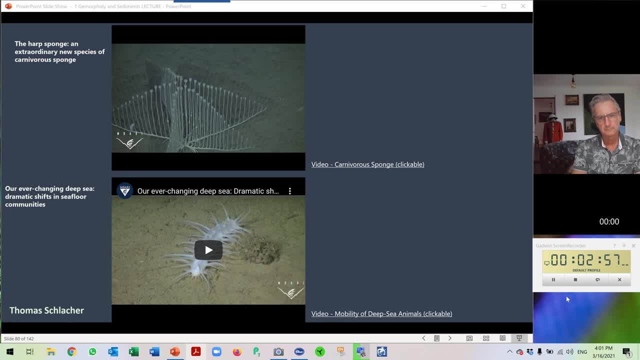 These sponges were observed on the deep sea floor off the coast of California. They live on soft muddy sediment at depths of 3,300 to 3,500 meters, where environmental conditions, including food sources, are extremely stable. The harp sponge anchors itself into this soft sediment with a root-like structure called a rhizoid. 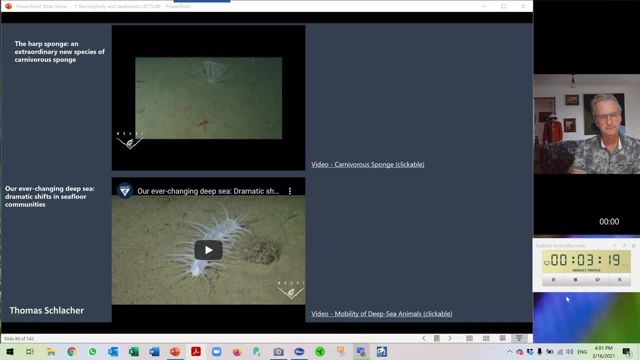 Other organisms, including anemones and sea cucumbers, were observed near the harp sponges. We named this unique animal a harp sponge because the shape of the vein and the vertically aligned branches resembles a harp, Like sea fan corals. we think the harp sponge evolved into this shape to maximize the surface area that is exposed to prevailing currents. 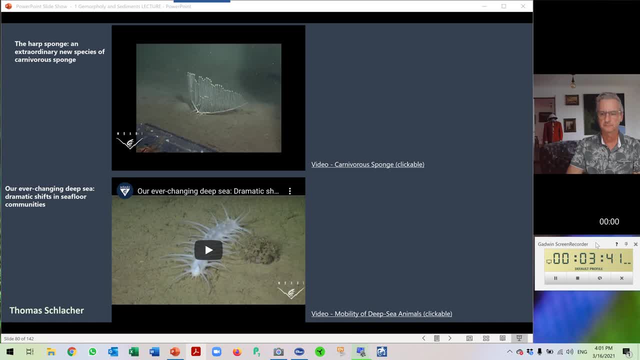 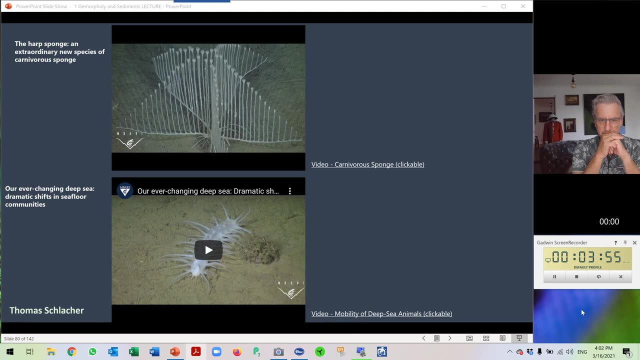 This increased surface area probably helps the sponge capture prey and release its eggs and sperm into passing ocean currents. The first specimens we encountered showed only two veins. However, additional observations revealed that the harp sponge often has multiple veins. Up to six have been observed, and these all radiate from the center of the organism. 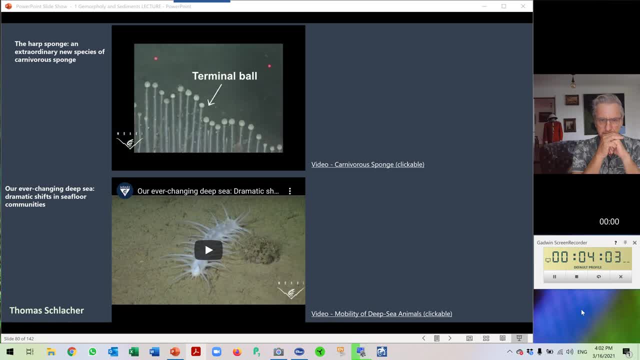 The upright branches of each vein typically end in a swollen ball, which is where packets of sperm are produced and released. When sperm packets released from other nearby sponges are captured on egg development sites of the vertical branches, the area becomes smaller. 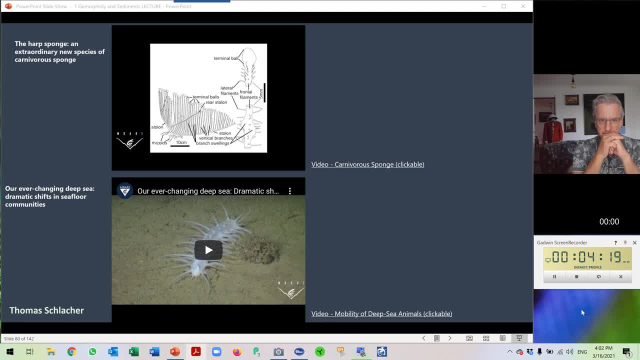 In addition to studying the new sponges' morphological characters and ecology, we used powerful microscopes to describe the shape and size of species-specific structural elements called spicules. Close examination and description of spicules is essential to species identification in sponges. 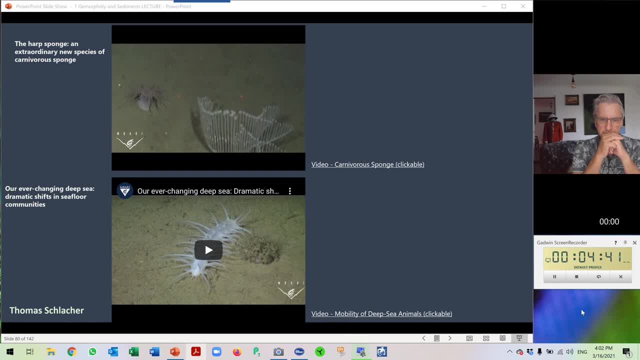 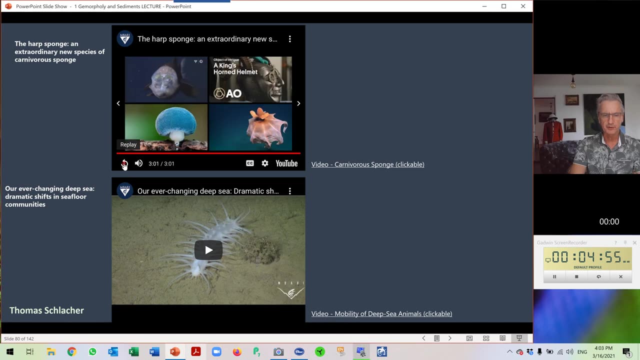 Our observations suggest that a related species of sponge may occur in deep waters of the South Atlantic. This unique discovery aids in our understanding of carnivorous sponge biology. So here you go. this is what is unique: a carnivorous sponge on a deep sea sediment plain. 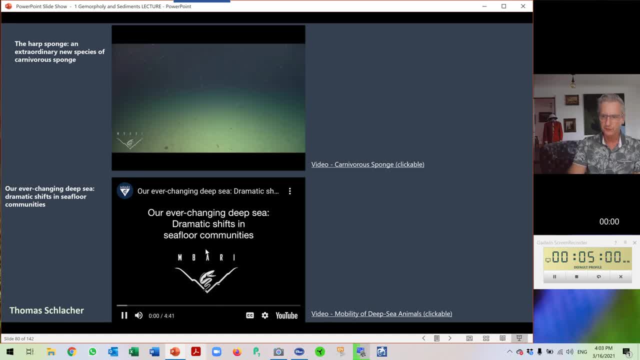 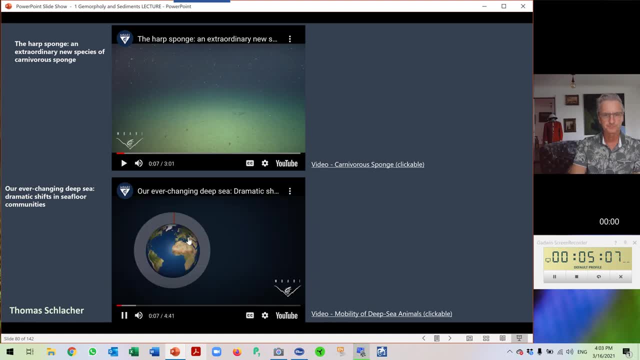 And if you think life in the deep sea is constant, scientists from the California Academy of Sciences are here to help you. Covering more than 70% of the planet's surface, the ocean surrounds us and is essential to life. However, it also contains the most remote and least understood habitats on Earth. 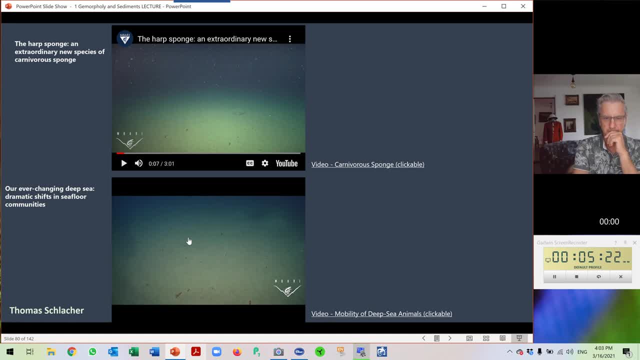 The majority of the ocean is very deep and remains largely unexplored. This is because of the difficulties working in such a harsh environment. In the mid-17th century, some researchers concluded that the deep sea was azoic, showing no traces of life. 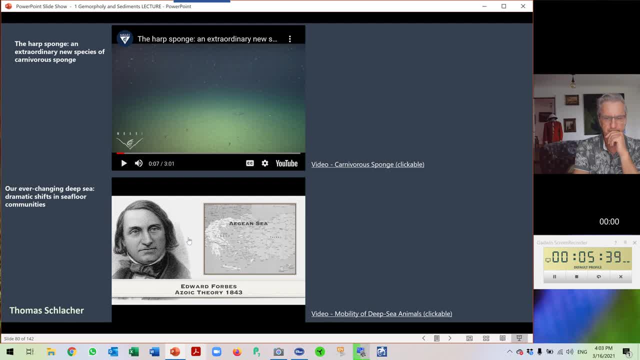 Part of this assumption was based on the lack of a food supply. With no light available down deep food can't be produced through photosynthesis, as it is in shallow water. Perhaps because it was so unimaginable, the idea of a life in the deep sea persisted. 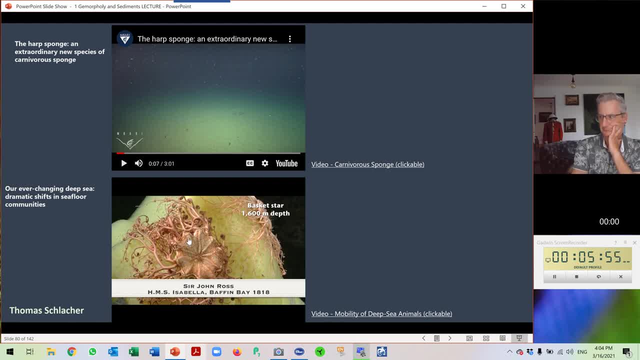 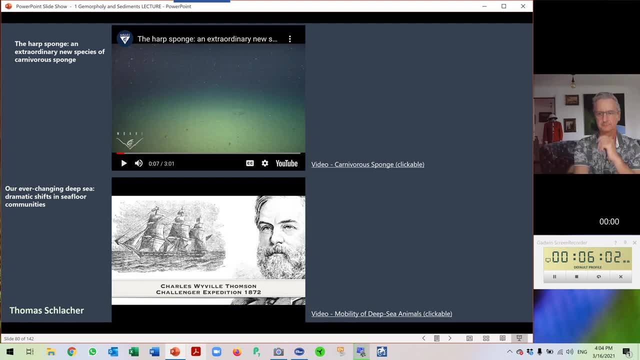 even in the face of evidence provided by earlier explorers who recovered remarkable animals like the spousal shark from deep water. With the advent of major research voyages such as the four-year-long Challenger expedition, our understanding of life in the deep sea increased tremendously. 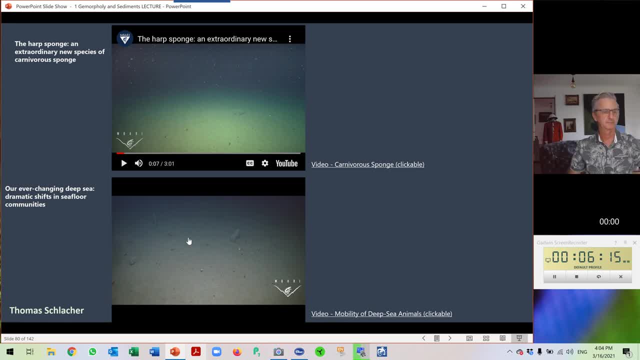 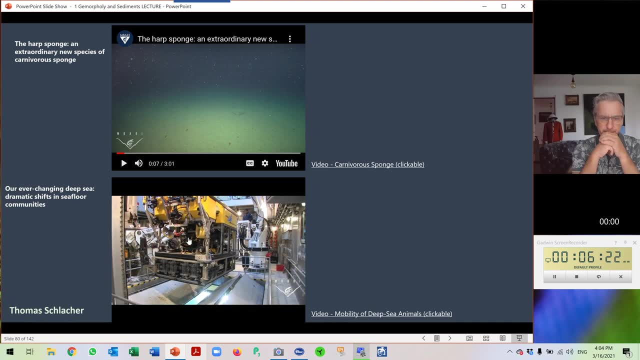 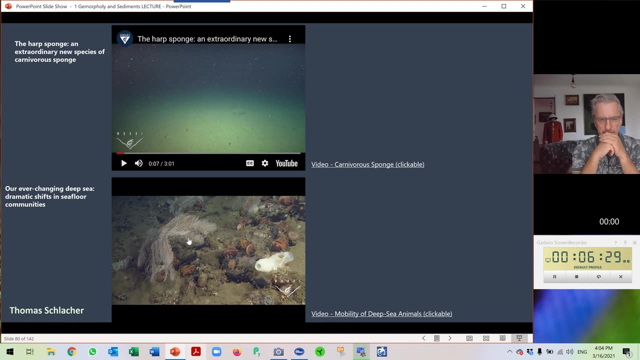 Yet it would be nearly another century before technology allowed us to begin to visualize these remote ecosystems. Newer technologies, such as remotely operated submarines, reveal what was previously hidden. The deep sea actually contains a variety of remarkable habitats that support rich biological communities. 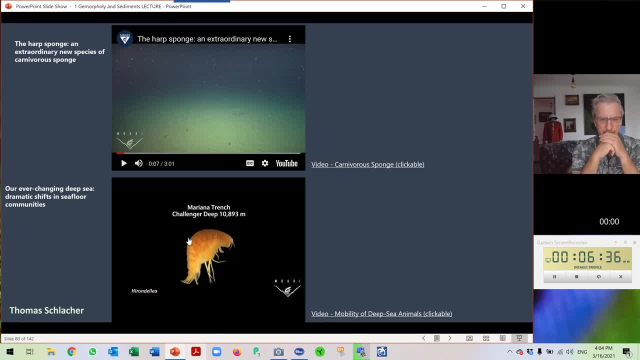 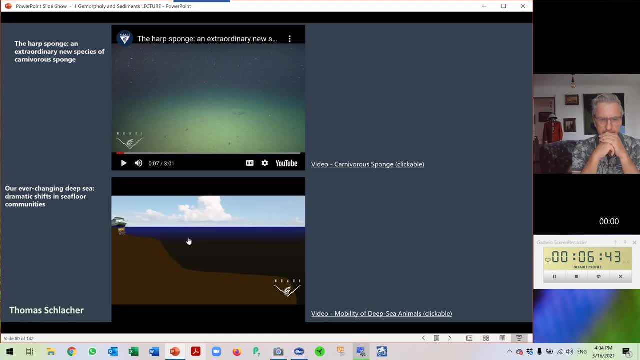 We now know that even in the Mariana Trench, the deepest part of the ocean, there is life. Crustaceans and other species live nearly seven miles down. As our vehicles descend into the ocean, light fades quickly. Temperatures drop to just above freezing. 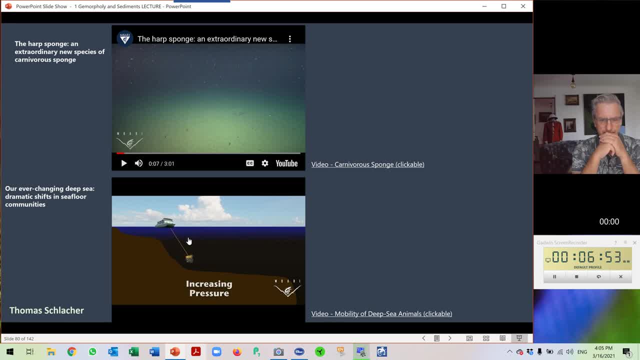 and the weight of the water above results in immense pressure. The vast abyssal area spans depths of 3,000 to 6,000 meters and comprises 76% of the entire ocean floor Off the coast of California. researchers have studied an abyssal area for the past 24 years. 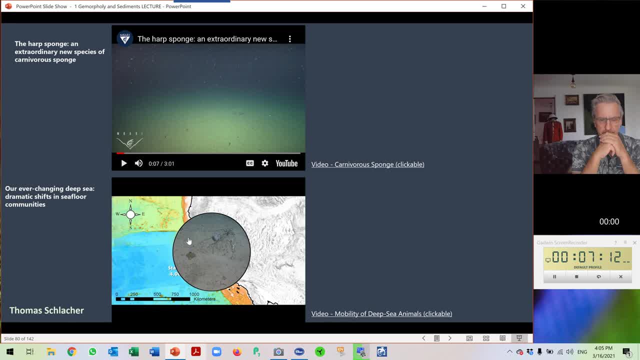 long thought to be a constant, unchanging environment, well isolated from changes taking place in the upper ocean. We now know that these areas can be dynamic and that the ecological changes there are linked to what is happening at the ocean's surface and, in fact, our whole global biosphere. 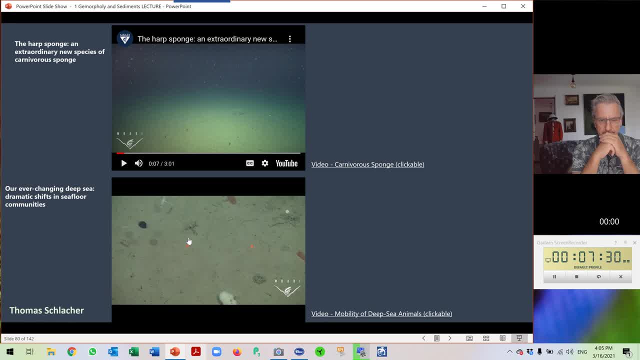 We've learned that animals living in the abyss survive on organic matter created in shallow water that floats downward. Small bits of dead animals and single-celled marine algae make their way to the sea floor, providing food for other organisms that filter it out of the water. 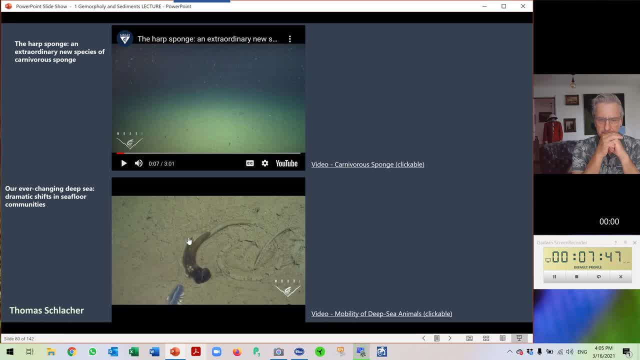 or extract it from mud on the bottom. Fluctuations in the number of animals on the sea floor are tied to the amount of organic matter falling from above. The changes we saw in the latter part of the study were quite dramatic. In 2006,, there was no obvious organic matter observed on the sea floor. 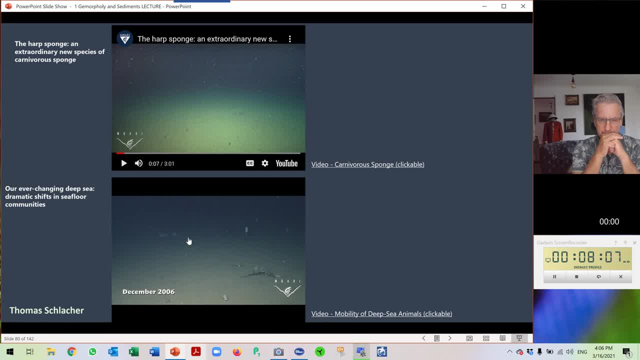 and there were mostly immobile filter-feeding animals living there. The number and types of animals stayed this way for some time, even during 2007,, when we saw an increasing amount of organic matter on the sea floor. By 2009,, the debris was no longer there. 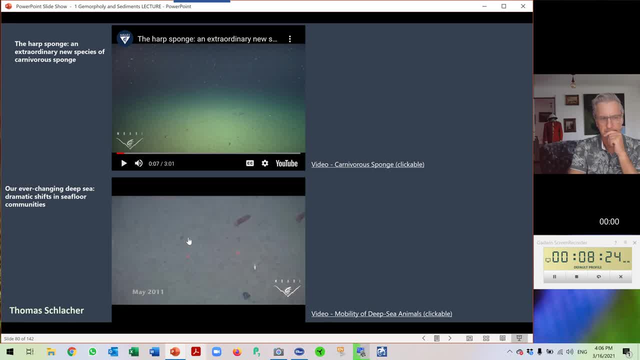 presumably having been eaten Within two years. the biological community changed dramatically. Now, large numbers of sea cucumbers dominated the sea floor. More dramatic changes took place in 2012.. In March, we saw salt bloom. Salts are gelatinous animals that are most abundant in surface waters. 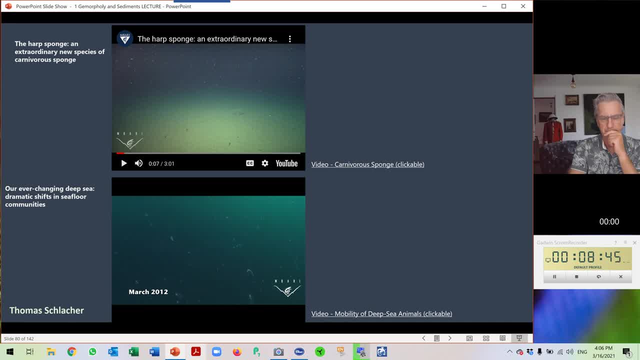 and whose numbers are known to increase rapidly Over the next two months. many of them drifted downward. Certain types of sea floor animals capable of taking advantage of this extra food thrived, becoming more abundant than at any other time in this 24-year study. 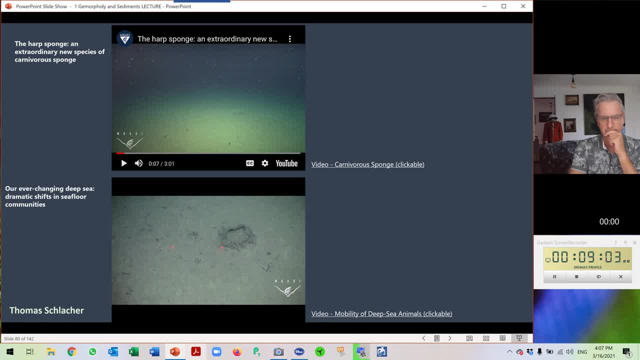 Other animals, such as sponges, became clogged and died. Our understanding of the deep sea is dependent on the development of technology. Autonomous vehicles like our Ventic rover can move along the seabed, measuring how much food is consumed and how much is stored in sediments for use by animals. 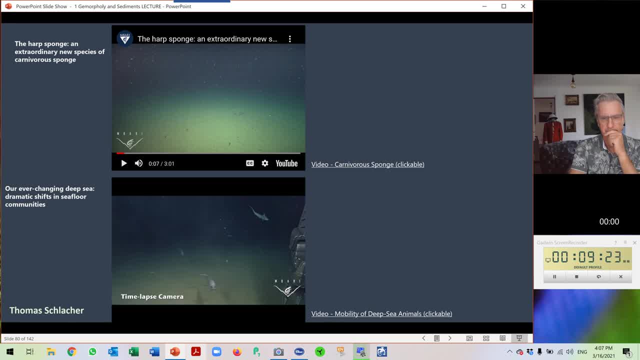 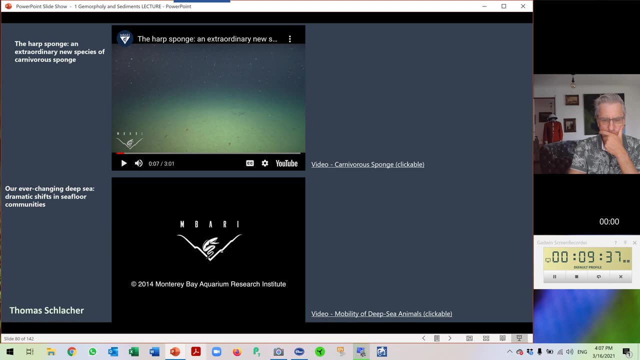 when less is raining down from above. Time-lapse cameras allow us to monitor the biological community and document food falls continuously for up to one year at a time. These types of long-term studies are essential for monitoring future ocean changes. This is Linda Coons for the Monterey Bay Aquarium Research Institute. 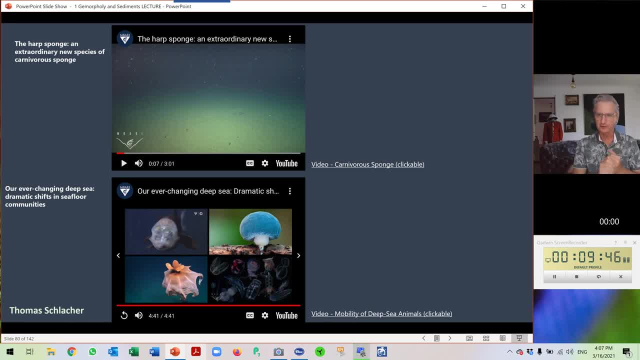 Right. So I think just this little glimpse into deep sea biology on a muddy sea floor should have convinced most of you that life is quite wondrous and often unknown. So you don't have to necessarily be on a rock, As a matter of fact. 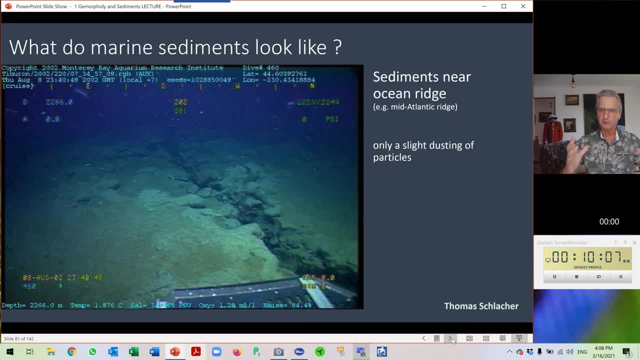 if you take a big view of the ocean, only very few areas look like this. This is actually at the spreading center, where new rock is being created at a mid-Atlantic ridge And, yes, there's only a slight dusting of sediment here. 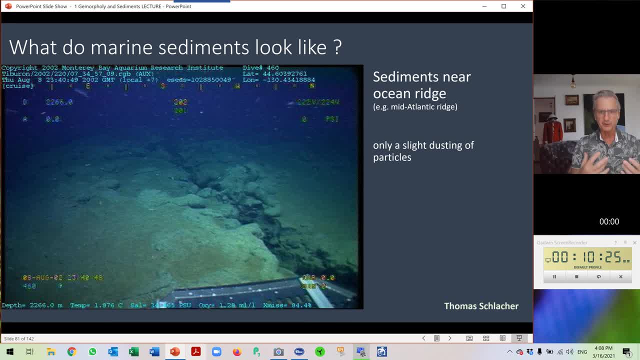 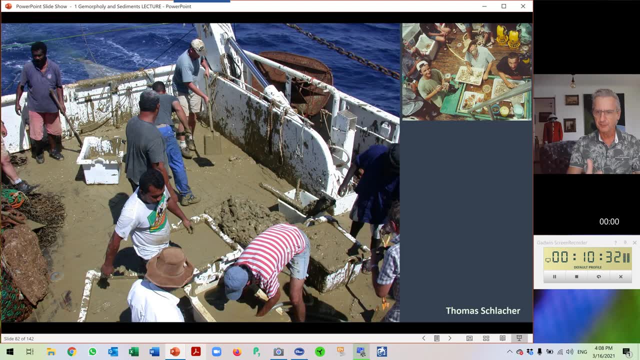 essentially because it's very young, So sediment didn't have time to accumulate there yet. However, in many other parts of the world it looks like this: This is in the middle of the Pacific And lots of biologically produced mud. Those are basically the skeletons of organisms. 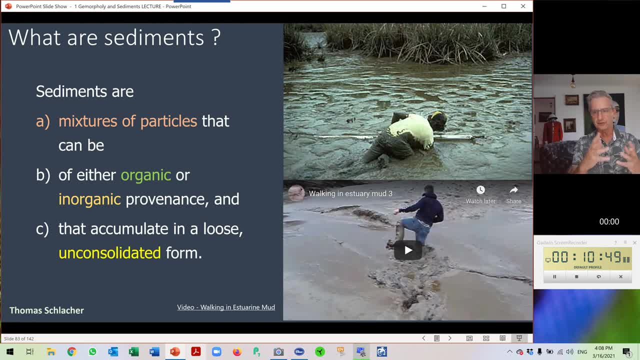 Now sediments. you know people say like, ah, it's just mud, so it actually is of no use to anybody really. Well, the first thing you have to actually realize is it's different particles. They're usually more than one source. 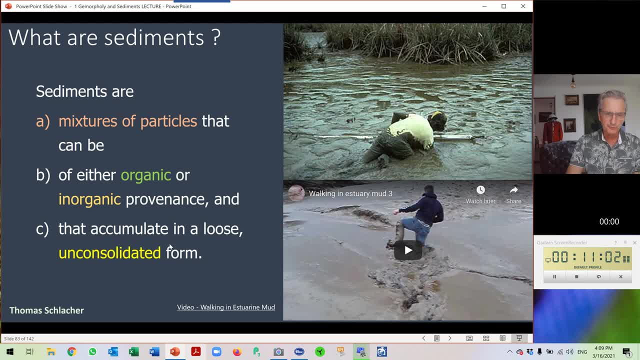 you know, contributing to it In terms of where it comes from. it can be either inorganic, like wetting of rocks from the land being washed in by rivers, or it can be organic, which basically means some of the fleshy remains of organisms. 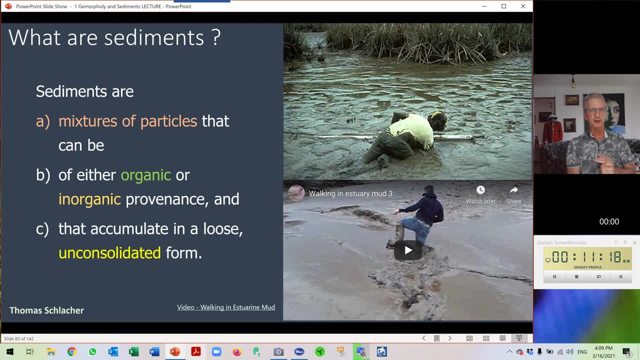 whose skeletons contribute to the sediments originally. But all sediments have one thing in common: they're malleable. they're pliable, they move. they change because they are loose. We call this unconsolidated right. So sediments are unconsolidated. 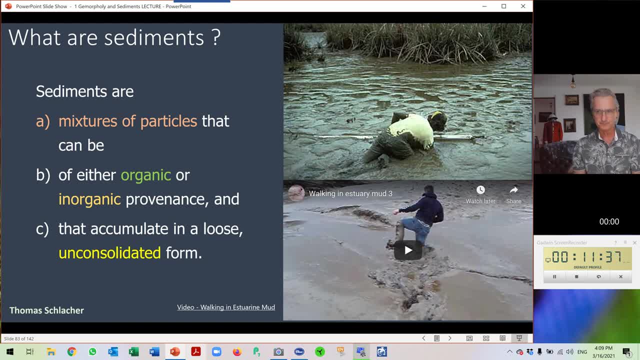 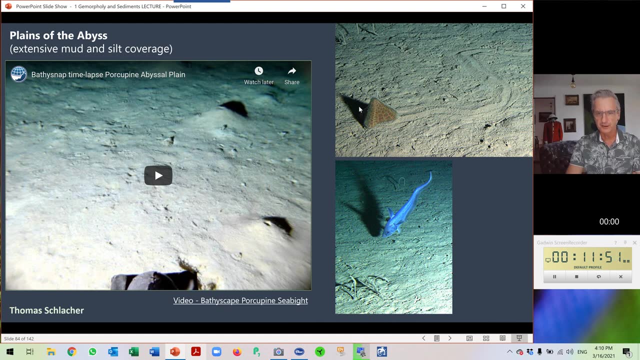 but they are so because they lack the long-term geological forces to combat them. Now we have already seen, you know, life on the deep sea floor. Here you can actually an urchin cruising around Here. we got a quantity of fish. 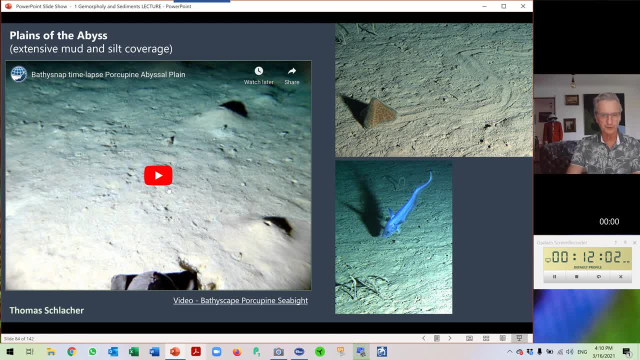 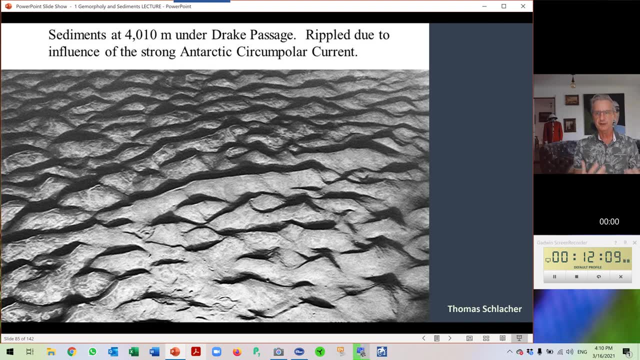 This is a time-snap camera. You can watch this in your own time. I've got the link at the bottom here. So one thing we also learned over the last 20, 30 years is: you know, image technology became more available. 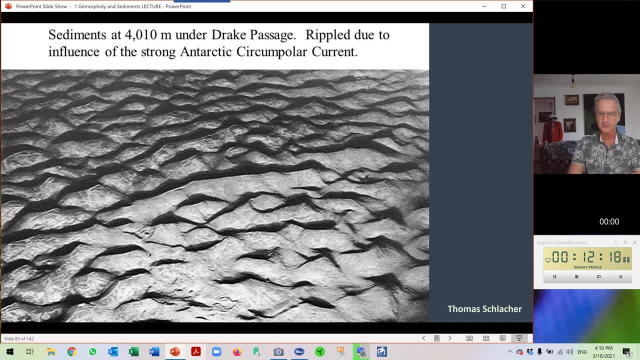 became better. We could use it in more locations. It is that the deep sea is not free of the forces which shape sediments somewhere else. ie here you got current ripples at about 4,000 meters near Antarctica, which is actually very. 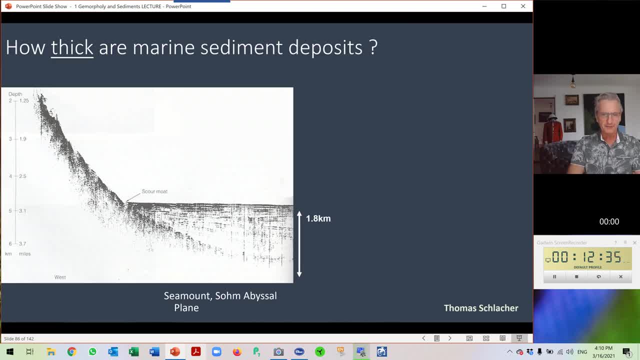 very remarkable. We will talk a little bit more like how much sediment we have, but I'll just give you this as a little pointer here, a teaser. This is a basically undersea mountain, a seamount, The flank coming down here. 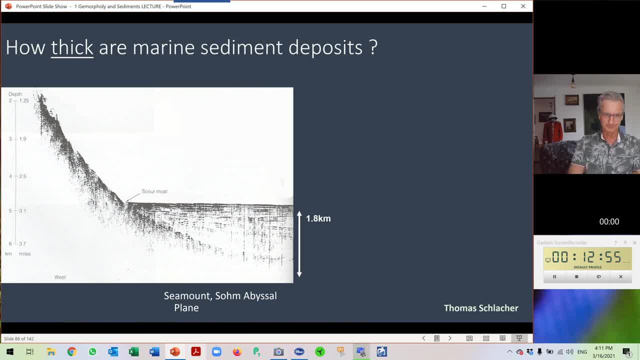 you got a little bit of a oops, a little bit of a scar here, And then we have this massive wedge of sediment covering about the first 1.8 kilometers of that mountain. Now let's just think about it. 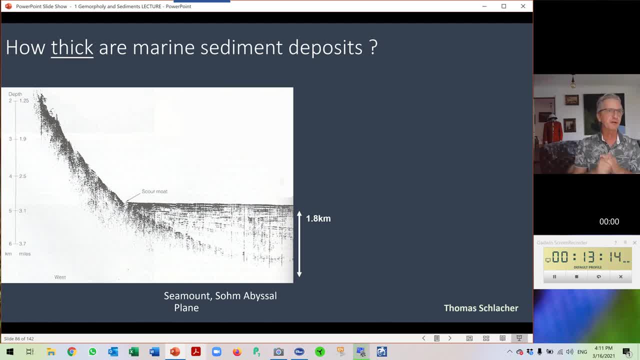 You know, we kind of get a little bit excited here on the Sunshine Coast If you have a mountain of a few hundred meters right like Mount Coulomb, which is hardly a hill in deep sea science, Pardon me- And here we got about 1.8 kilometers of mud. 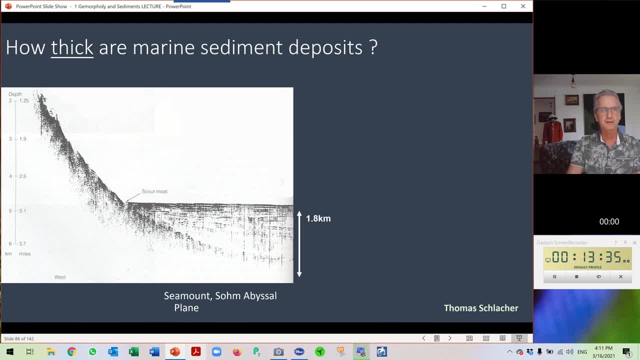 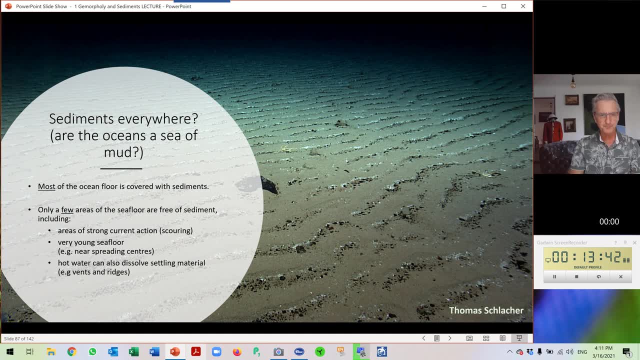 And this is actually a fairly tiny deposit, because in many parts of the world we actually get up to nine kilometers of mud. So, yes, our sediment is everywhere. Most of the ocean floor consists of muddy, sandy, salty particles, And the only areas which are free is. 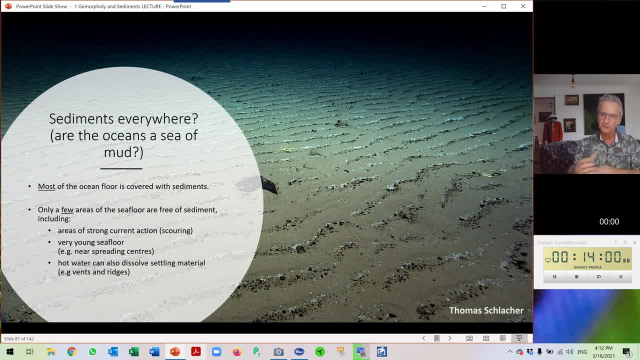 you know, the top of undersea mountains, like seamounts where the strong currents sweep the sediment off, or very young seafloor near spreading centers or when hot water dissolves some of the settled material. But those are really exceptions. 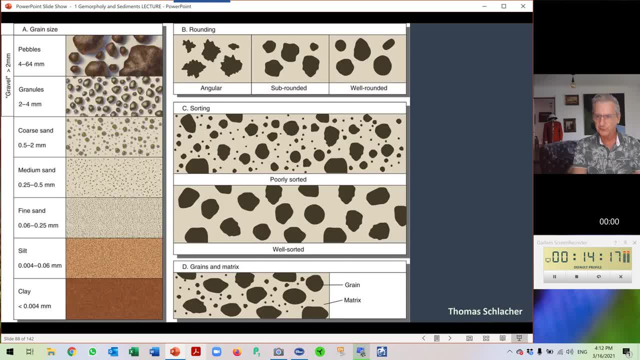 you know by and large Now, because sediments are so prominent, this is what might look a very boring classification, But if your first job is in environmental consultancy- and for many of you that will be the bread and butter- I can almost guarantee that it will have something to do with sedimentary features. 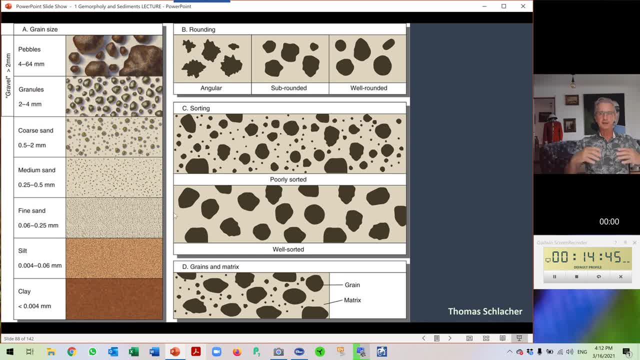 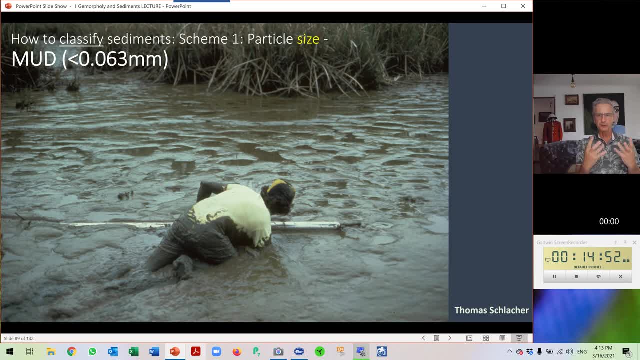 And we quite often actually use this kind of classification. We're talking about pebbles, we're talking about granules and so forth. So the official name for anything smaller than 63 micrometers is mud. Here we got. 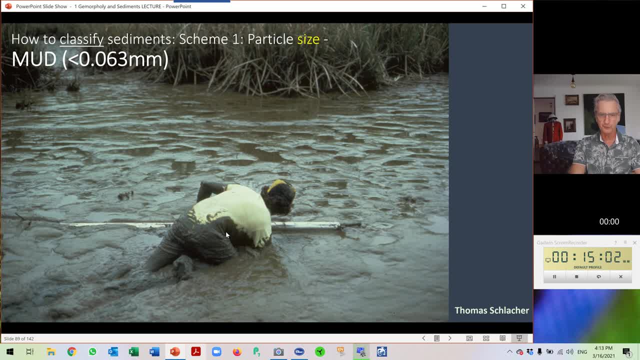 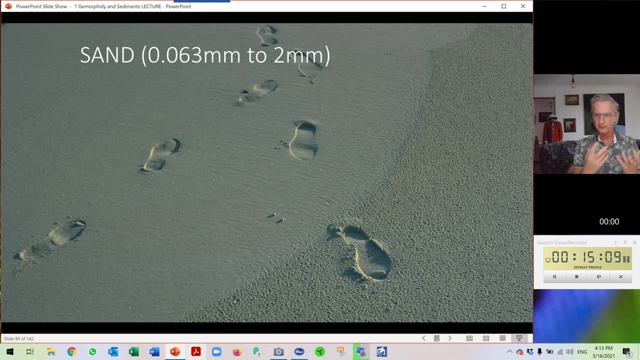 you know a thing called a consumable item- I think it's called a student, you know disappearing in the mud. Then we move on. anything up to two millimeters is sand. Two millimeters is actually really the upper, you know. 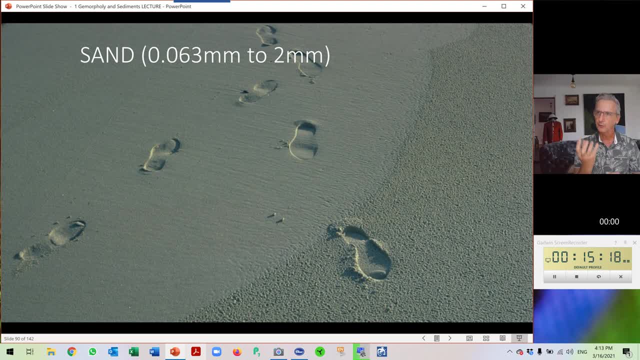 size class boundary, because it's quite coarse. You might say, oh, two millimeters is not actually very much. Well, you know, on our beaches, our meaning the Sunshine Coast, the average diameter of a sand grain is roughly about. 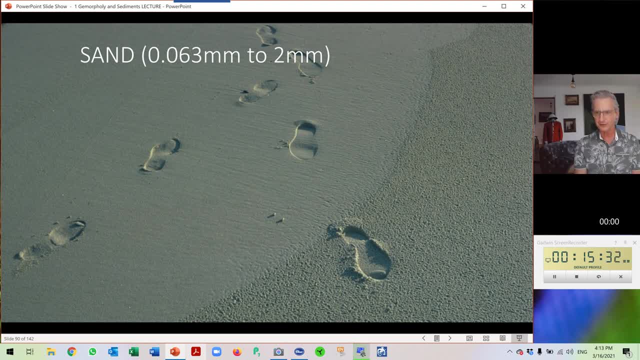 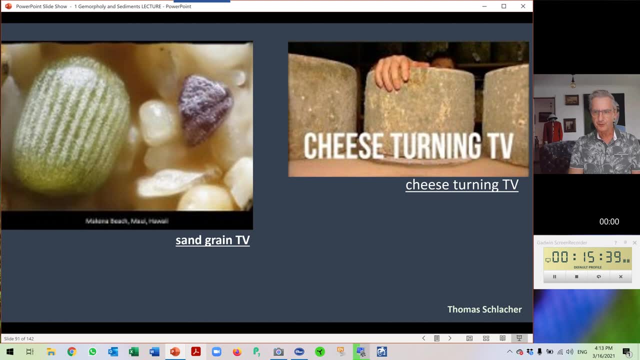 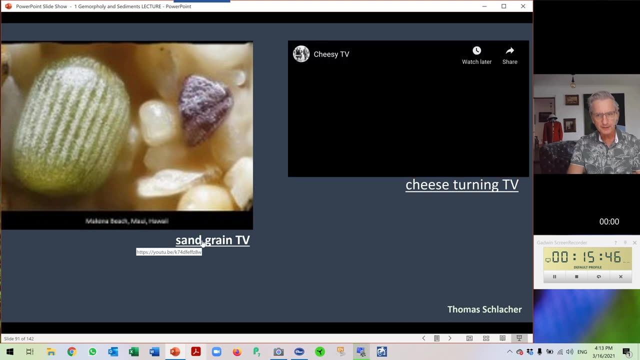 I don't know exactly. it's 353 micrometers out of many thousands of measurements. Now, I did some poking around on the internet. to you know, look for videos about sand. I came across this one, And this is some crazy guy who said: 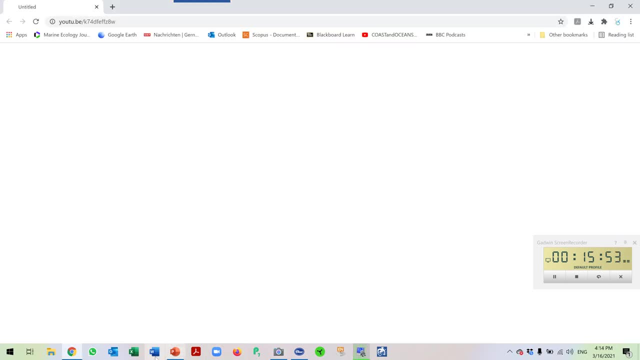 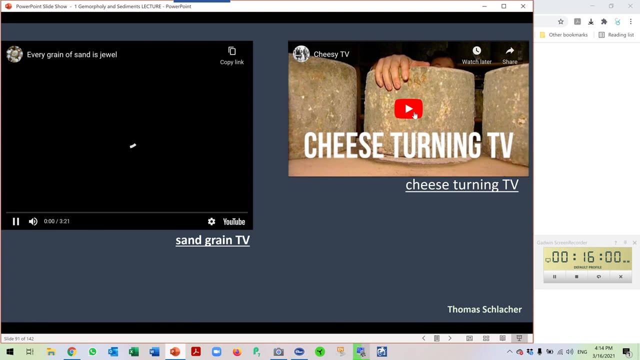 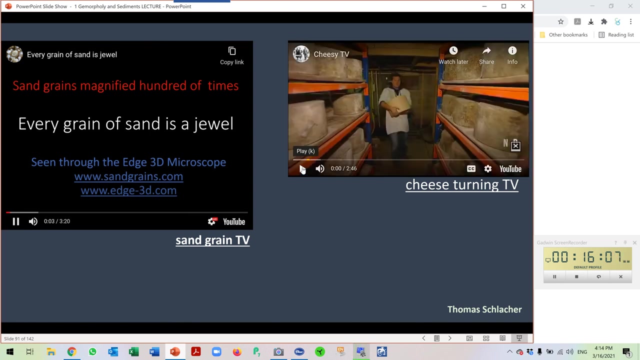 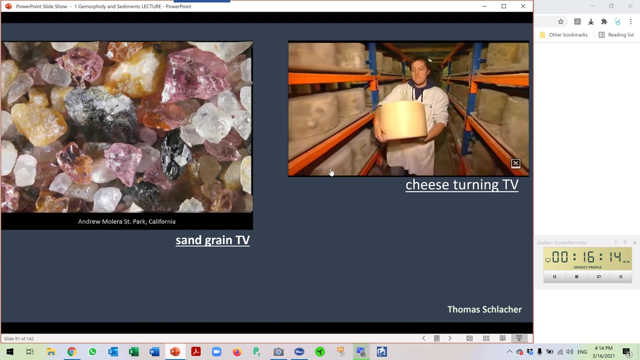 oh, I invented a 3D microscope And what I can do is actually show you some, um, uh, sand grains, And what is actually truly astonishing is is that, uh, that every beach seems to have a very unique composition in terms of what the sand grains. 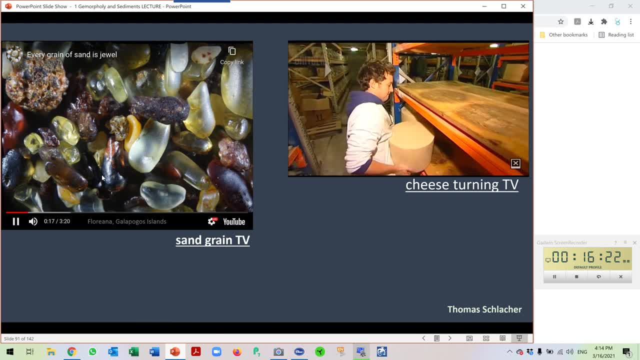 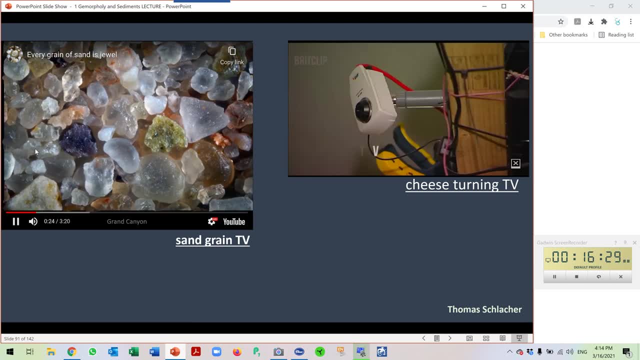 look like. Here's your classic quartz. This is quite red. Do you see how rounded it is? So it must have actually been swashing around for quite a long time. Yeah, I think so. Much fresher than the Grand Canyon. 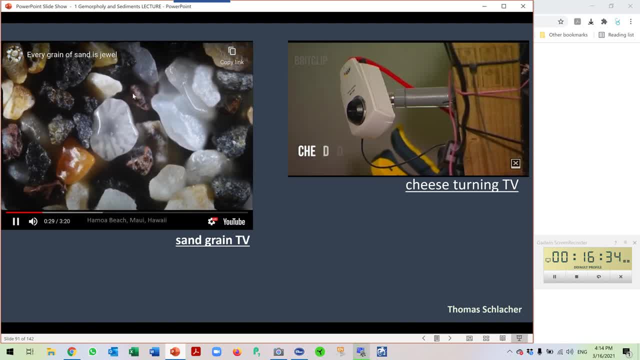 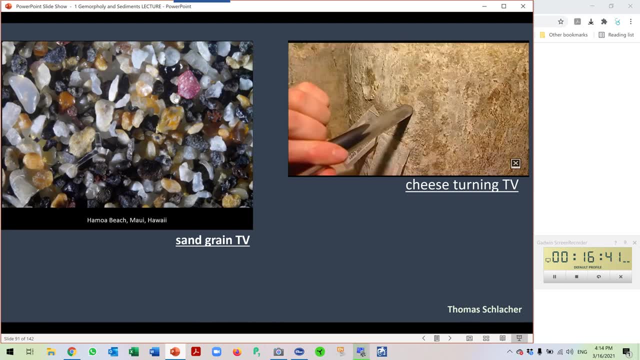 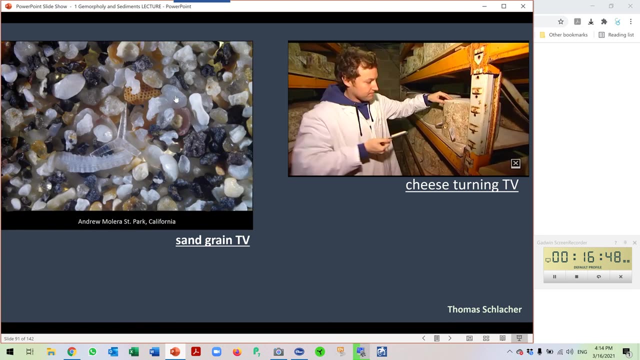 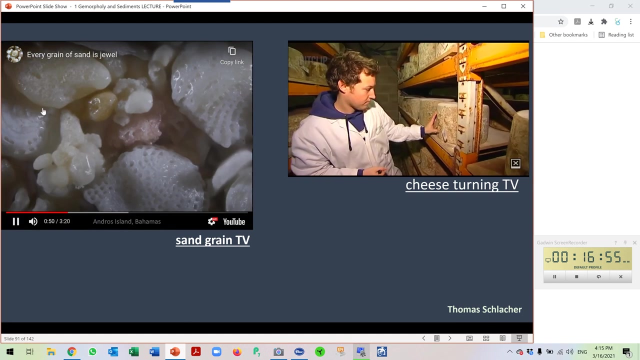 No surprise, there Another beach sand. here is a ferrominifer, Here's a basaltic rock. So that is more to sand grains or to a collection of particles than just a basically collection of innate geological objects. Here we got a ferrominifer. 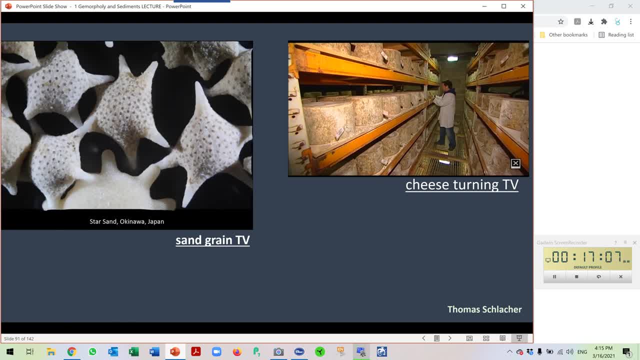 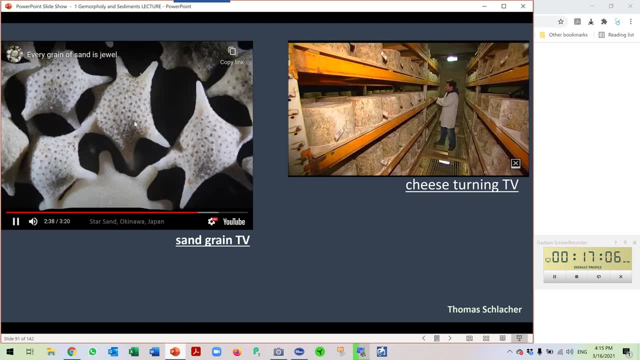 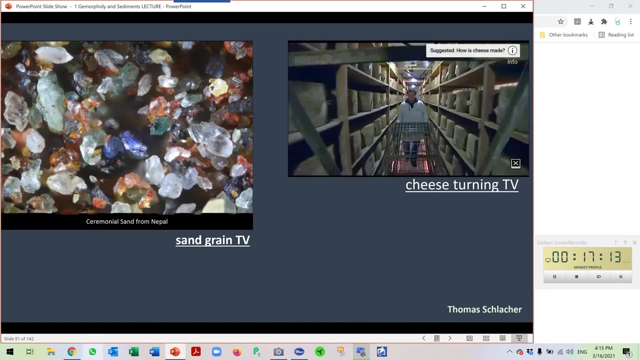 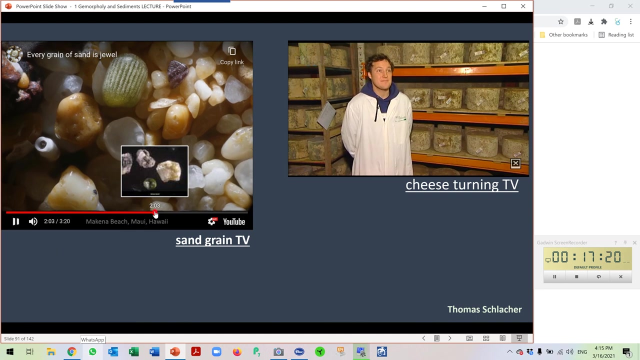 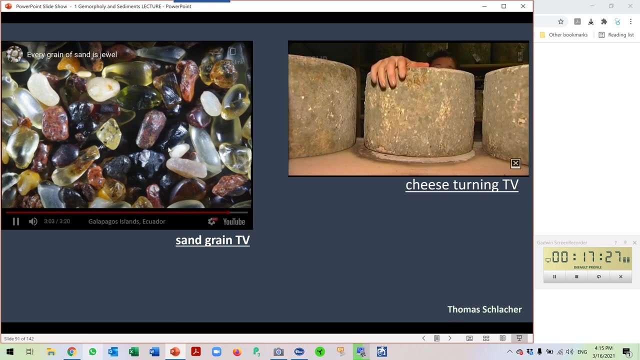 Now this is a bryozone, uh, probably skeleton and so forth and so forth. so if you really want to completely relax, oh, it does have four mini furs, isn't that kind of really cool? the star sand, i think it's very cool. so he likes to seem, he likes to be going to to hawaii. but if you're really bored and you want, 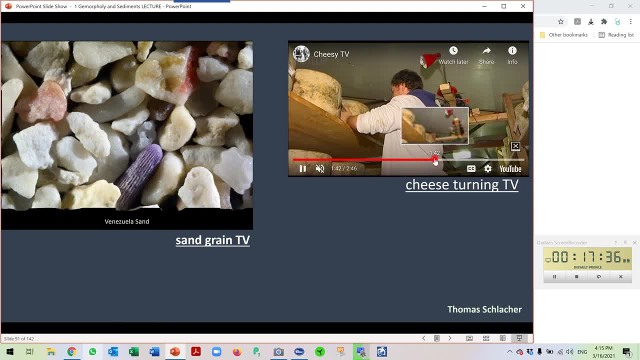 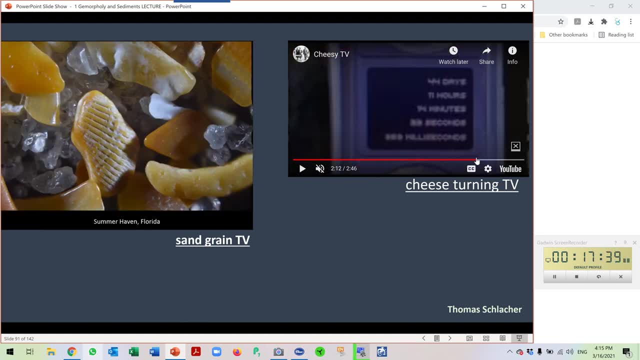 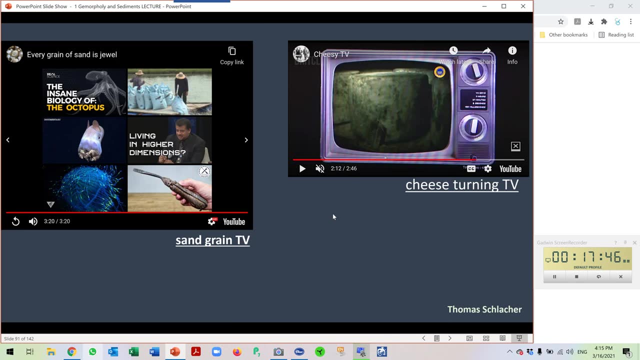 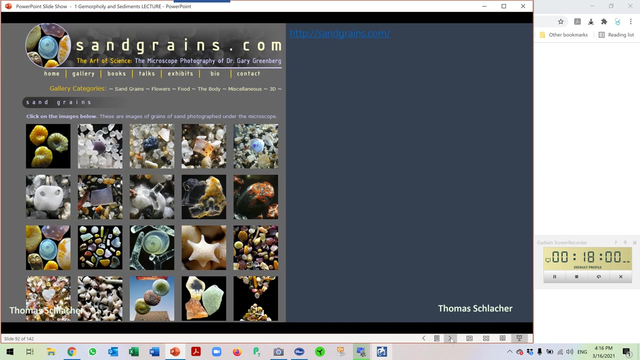 actually watch a lot of sand. you can also watch the cheddar cheese uh, basically, uh, maturing facility that's. you know they're also extremely cheddar cheesy tv. you know it's kind of interesting stuff, but you know it's just about in the same league of being kind of very esoteric. now here is the web link to it. you can also hire. 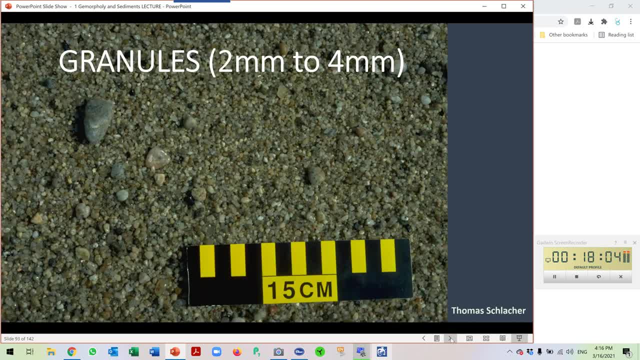 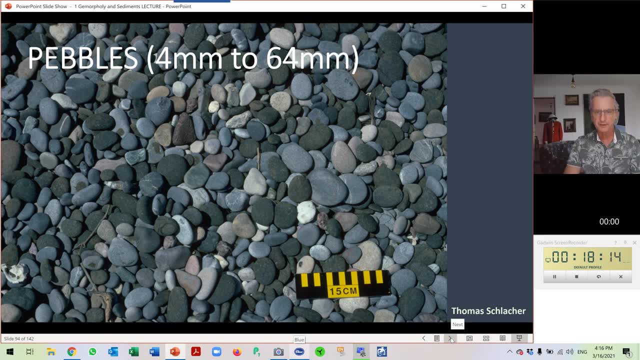 this guy for talks the flowers through the body and so forth. very uh, as we actually move up, we get into kernels up to four millimeters, then pebbles. they go up to about 64 millimeters and then everything, uh, up to about that much is called cobblers and everything. 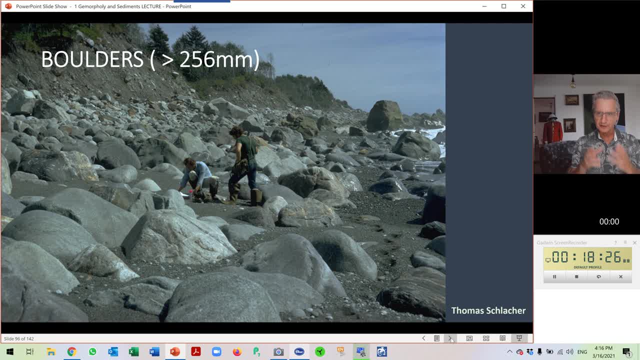 larger than about a quarter of a meter is bolder. so there are official classifications and you have to use the correct term. you know it takes a little bit of experience, particularly when it comes to things like cobblers, which we actually think are, in normandy usage, a little bit bigger. 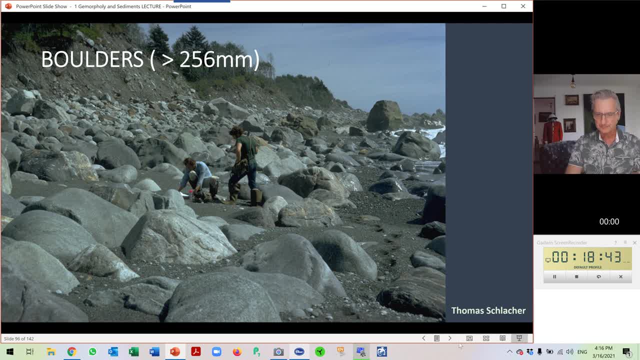 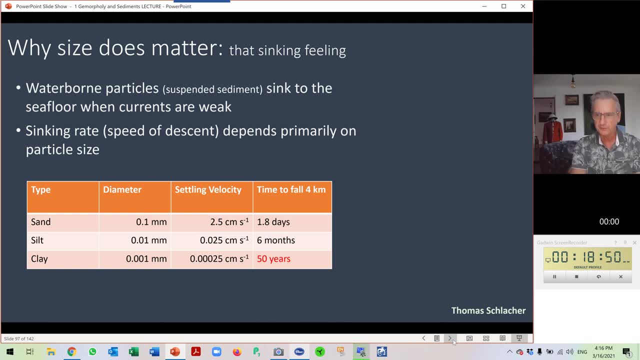 terms for each of those right now. why are we so obsessed when we talk about sediment, about particle size? the reason for that is actually quite simple and that has to do with the settling velocity. settling velocity is crucially important because it connects the shallow parts of the oceans. 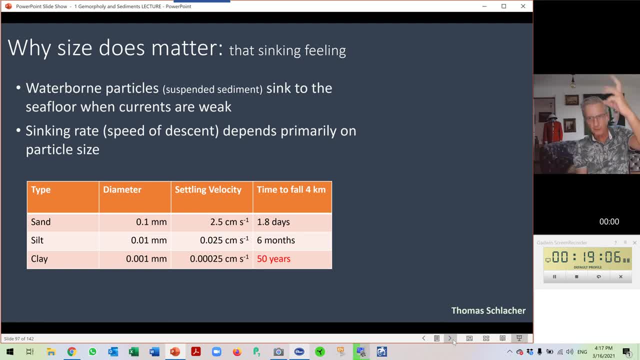 with the big ones through the setting of particles. so the rain of particles going from shallow, sunlit to the deep ocean and ultimately forming the bottom of the deep ocean. now why do smaller particles sink so much? smaller than slower than bigger ones? it has to do with the ratio between 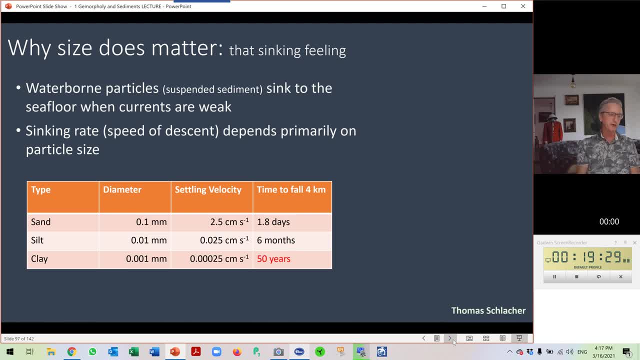 gravitational force and friction of a body. i've got my dive watch here, so think about. this is actually a particle, as it actually goes through the water, it actually bounces between the water molecules. it has to basically displace them. now that displacement means the molecule rubs against the water molecules, they might say: well, you know, gravitational attraction is actually. 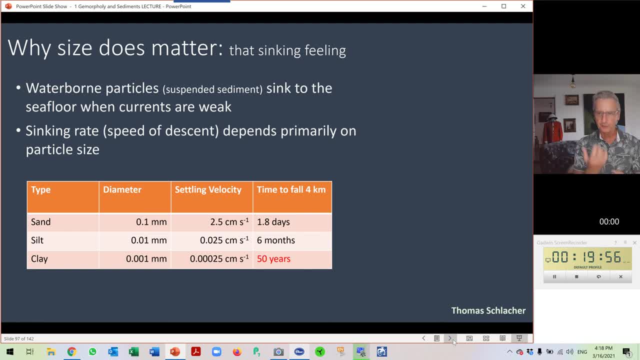 pulling it down. well, the gravitational attraction depends on the weight, which means are, which depends on the volume of the organism. now, let's suppose you have a very small particle, like a large particle, like a little round one. you might actually take up to about 50 years, if nothing. 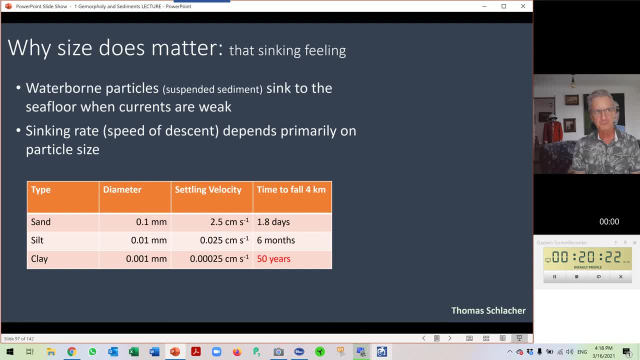 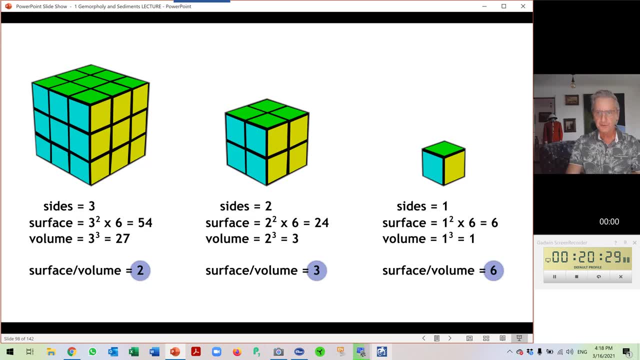 happens to you to basically sink from seven meters to four thousand meters, which is the average depth of the ocean. now, why is that? it's quite simple, really: because as you actually have a smaller body volume, the ratio of your body volume increases by the time that you have a smaller body volume. 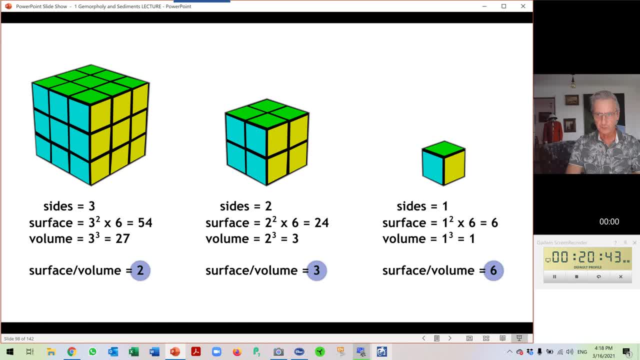 disproportionately to the surface area. So a smaller particle has a much larger surface area, which basically means surface area is friction, whereas volume means gravitational force pulling you down. In other words, you are at a disadvantage the smaller you get as a particle, because you're missing out on weight. 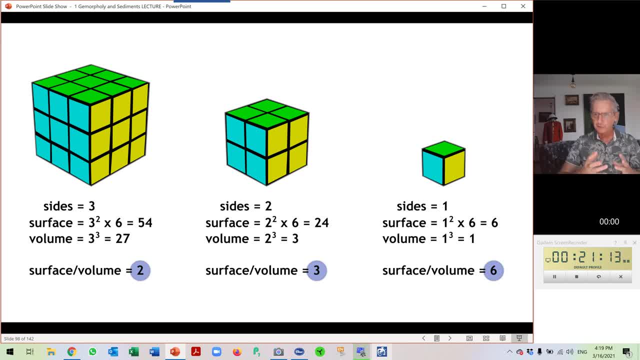 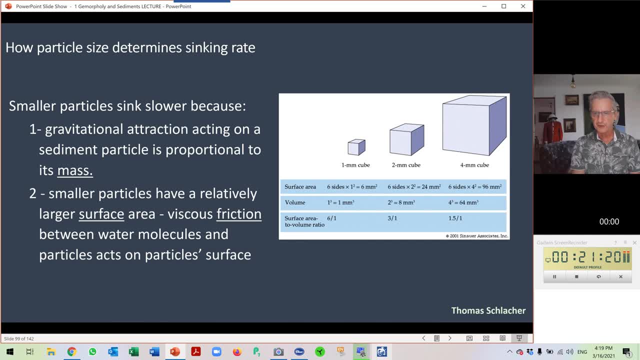 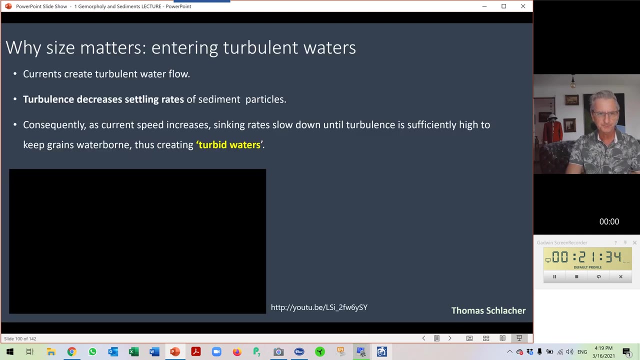 but you're actually increasing your surface area in relation to the little bit of weight you still have. The upshot of it is that, essentially, small particles sink very slowly, extremely slowly, because their surface area, ie their frictional potential, is actually so large. 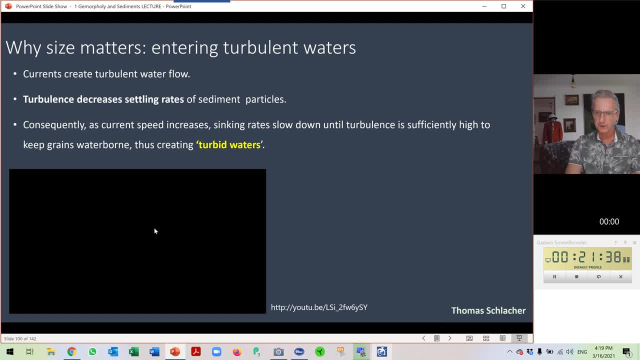 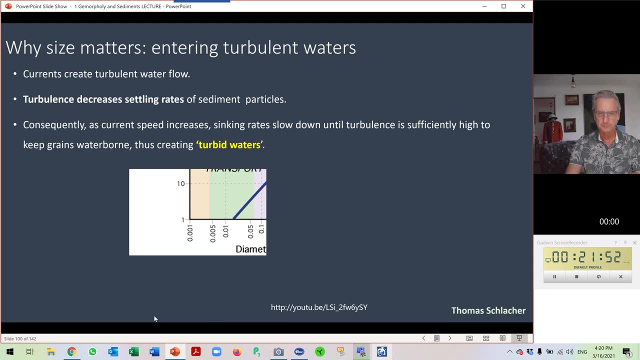 Now, this is quite funny. I was like: hmm, how can I, you know, illustrate? Oh, it doesn't really come. Where is it? Come on, Can we poke it out? No, No, Never mind, That is actually just supposed to actually show you a turbulent water flow. 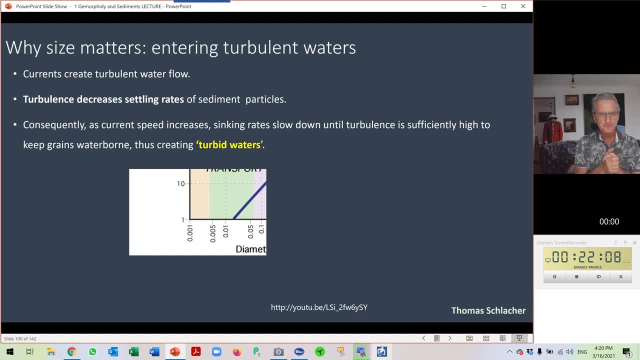 but it doesn't. It doesn't really want to play. What actually happens is when you have a very turbulent water flow, particles stay in suspension, They never have a chance to settle out and basically we have an expression for that, and it is turbid waters. 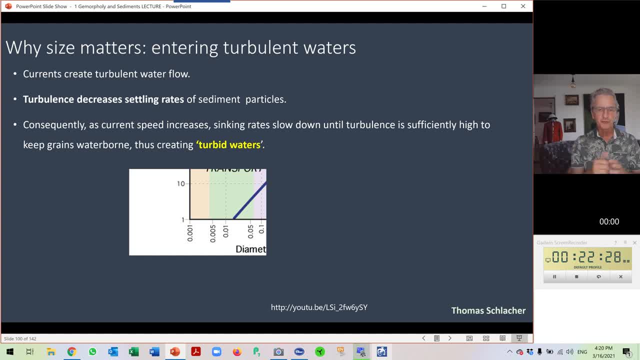 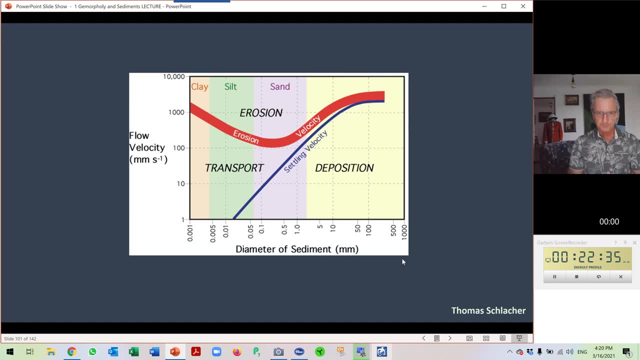 Turbid waters is basically any solution of very fine particles where turbulence keeps them from settling out. Now this is a very famous- or should I say infamous- diagram, because if you're an environmental consultant or any other marine biologist having to do with particles, 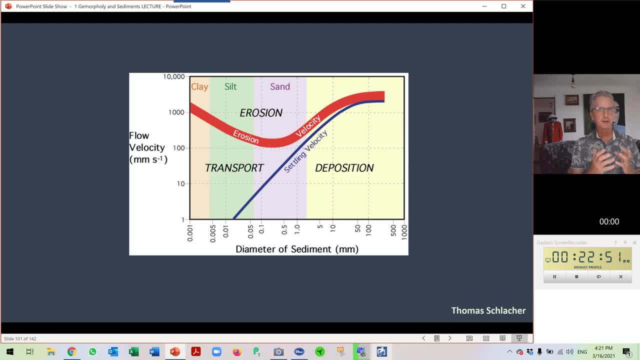 you come back to that a lot. Why do you come back to that a lot? Because it is for you the relationship between whether a particle remains in suspension, whether it settles out and hence the water becomes clearer, or whether it's actually transported in a large or a small distance. 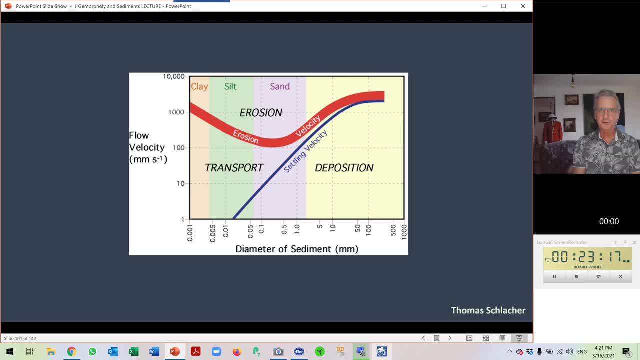 Now, all of those are very, very important considerations when it comes to environmental protection, safeguards for building projects, civil engineering and so forth and so forth. Now you can actually read that thing in two ways. You can say: okay. 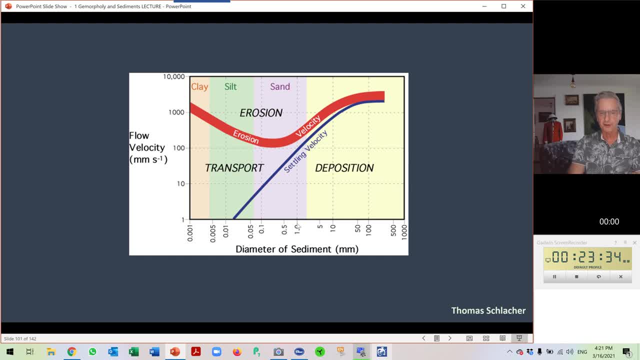 I have, let's say, very coarse sand of one millimeter, and you then actually can say, ooh, as long as my current stays under 100 millimeters per second, that sediment will actually settle out. It will become, you know. 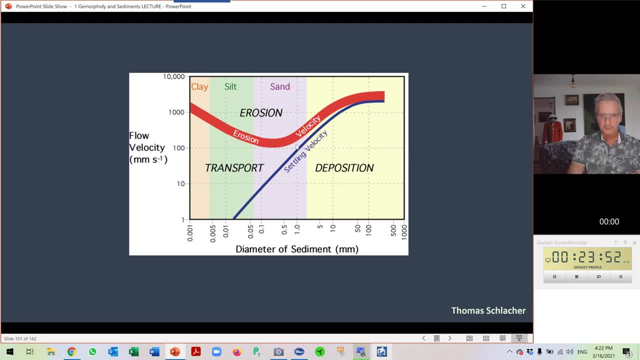 a deposit on the sea floor. If it's slightly higher, it will actually be transported, and if it's even slightly higher the flow velocity, it will actually remove it, It will erode it away. You can actually also say then. 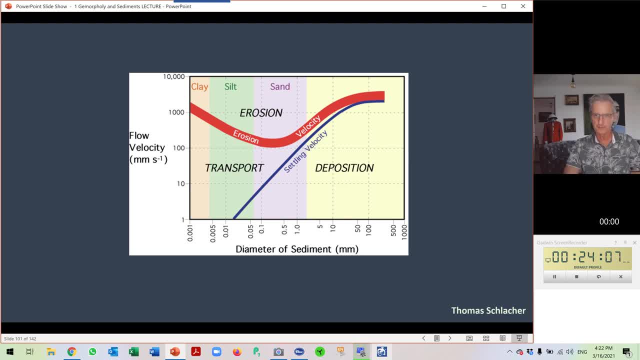 well, if I want to avoid right any increase in turbidity, given my sediment, I should really have flow velocities well below that blue line. Very practical measure you can actually adopt, let's say on a building project. So this is enormously useful. 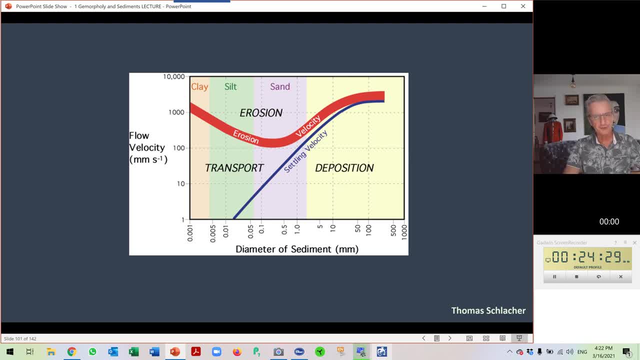 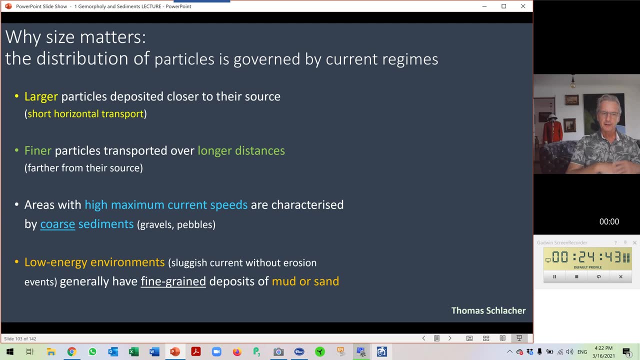 If you don't really like reading diagrams- and I think you need to get into the habit of actually doing it- I can actually cut it down to a few very, very basic observations, And they are essentially. large particles will usually be deposited closer to their source. 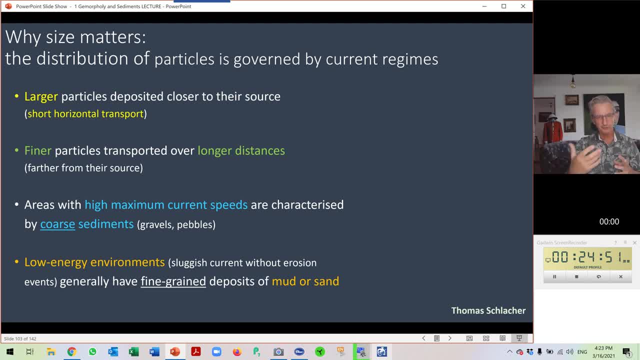 ie they don't actually travel very far for a given current speed. Fine particles, on the other hand, are transported over longer distances, ie they move far out into the sea. once they get released from the land, You can also go and look at a particular habitat. 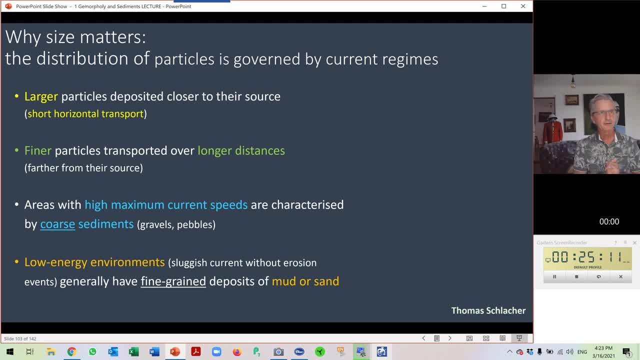 and can basically tell, from the type of sediment you find there, what the current situation or the current conditions in terms of maximum current speeds usually are. If you go, let's say, to a beach with very coarse sediment, you can be fairly sure or fairly certain. 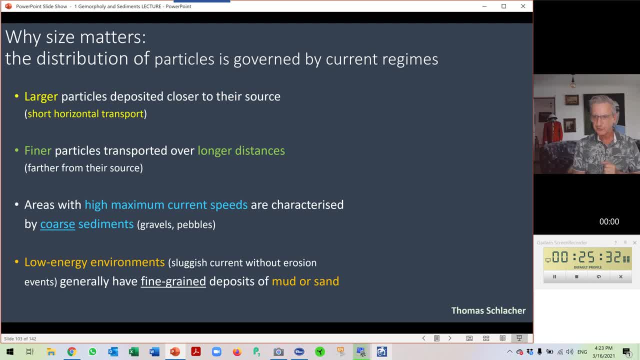 that sediment is caused for the simple reason because all the fine particles have been removed, meaning currents are strong. If you go to a low energy environment, you can tell, if the sediment is very fine, that currents are sluggish, because even fine particles can actually settle out there. 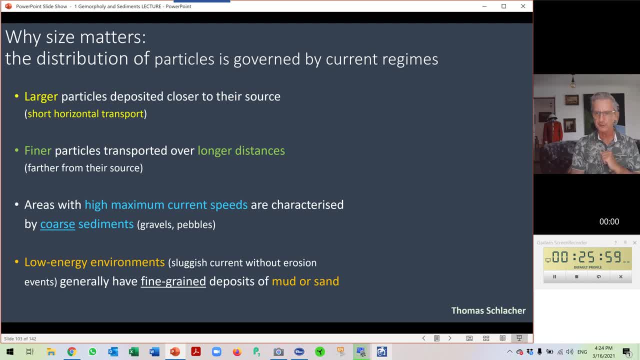 and will not, on average, be removed, eroded away from the area. So sediment coarseness or fineness or particle size, whatever you want to actually call it- gives you a very, very good time-integrated measure of the energy conditions impacting. 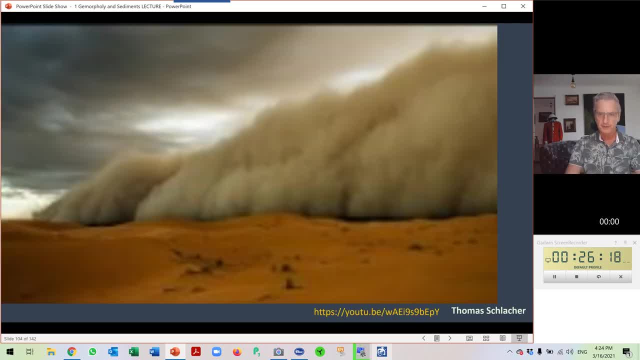 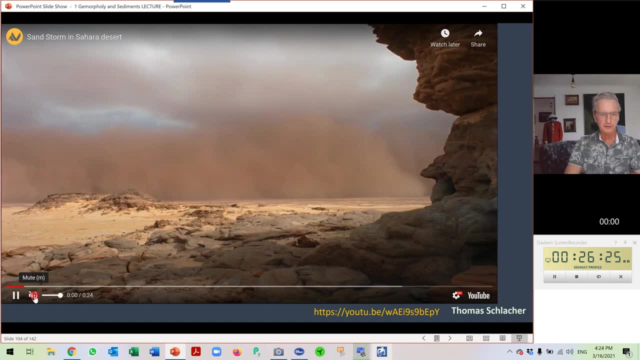 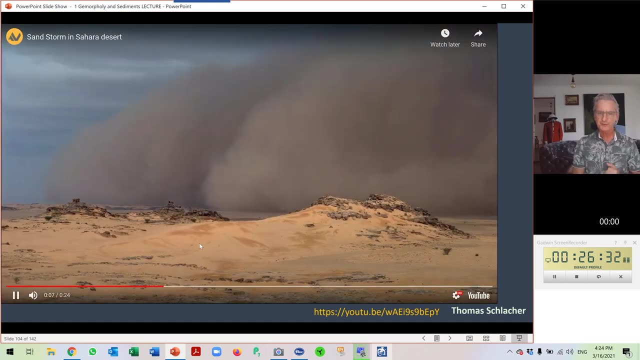 on the sea floor. Now here is a video of a sandstorm and you might say, ooh, Schlacher, now completely lost it. Why do I show you a video of a sandstorm? The reason is this is: believe it or not? 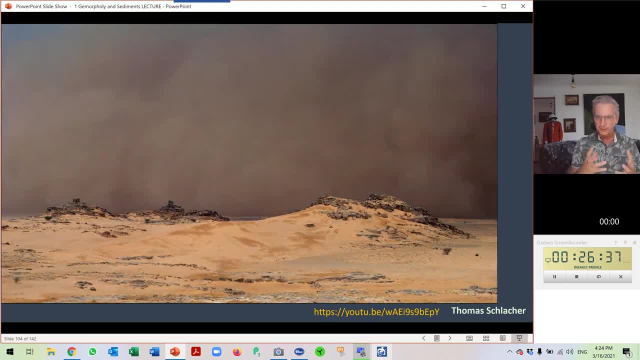 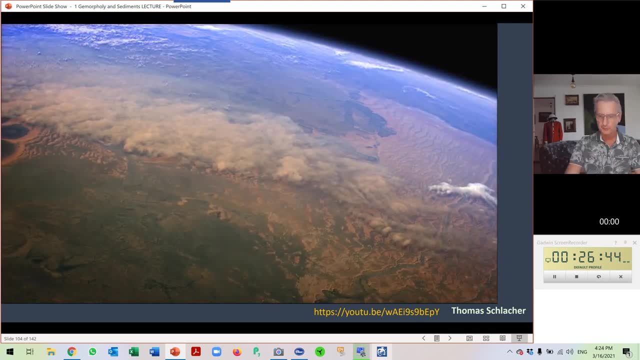 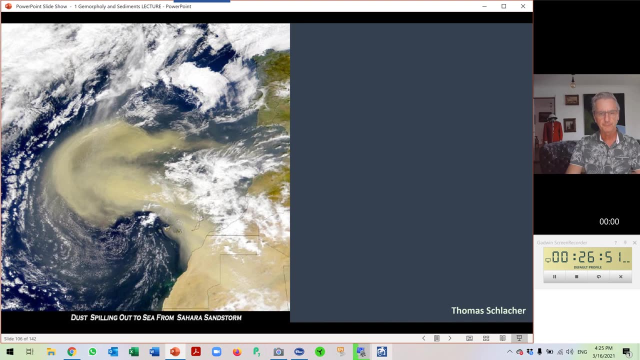 one of the significant sources of sediment being supplied to the oceans. It's a mechanism of transport from the land to the sea. How does that work? Well, look at a satellite picture. Here we go. This is the Iberian Peninsula. 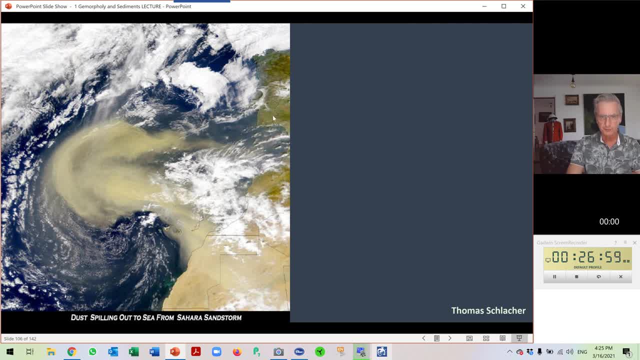 Well, you know, cut off really just in the extra material here. This is Portugal, This is Galicia, Then we go down here to the Straits of Gibraltar. This is Morocco, Mauritania, Senegal and so forth. 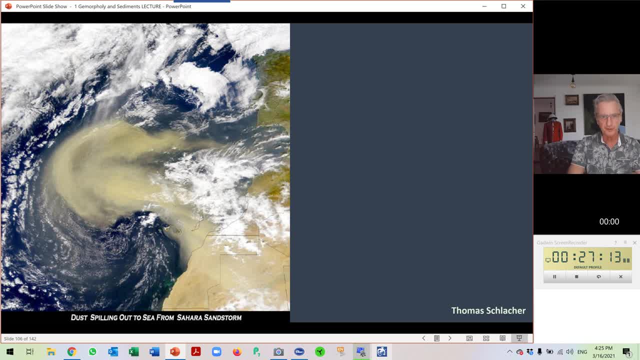 And you can see this massive dust storm moving off from the Sahara into the North Atlantic. Look at this size of the sediment plume. Those are millions of tons of sand being transported from the land to the sea. So this is one of the transport processes. 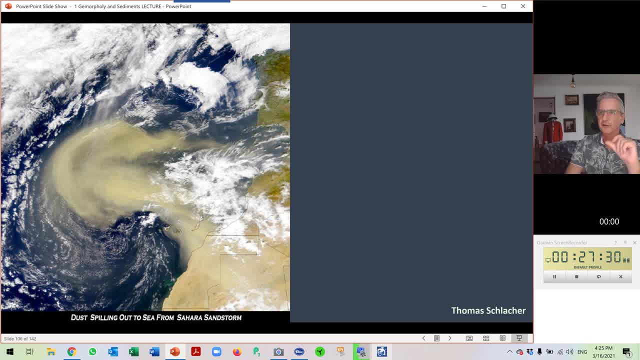 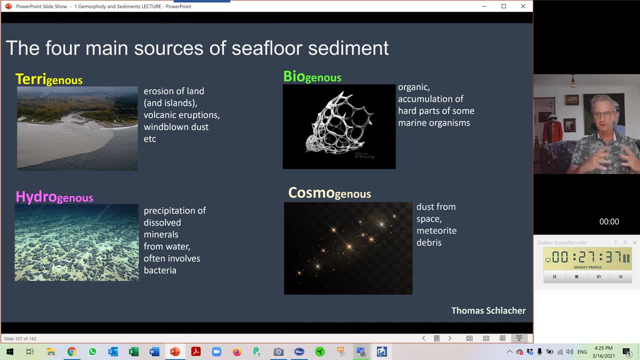 and it gives you an indication of where the main sources of sediment might lie. Broadly speaking, we differentiate or we distinguish four different types of sediments. You can say: well, we do know that, even the Himalayan peaks, you know. 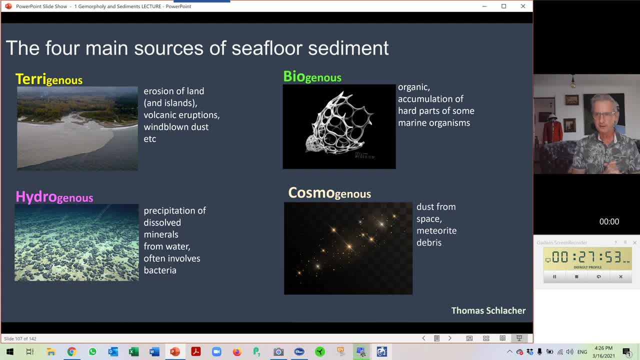 will not stand forever. In 2 billion years of time, there will actually be fairly hilly, insignificant things, because they will have just wetted away And that erosion of the land, supplying rivers with sand and then ultimately, as the sand becomes, melted down. 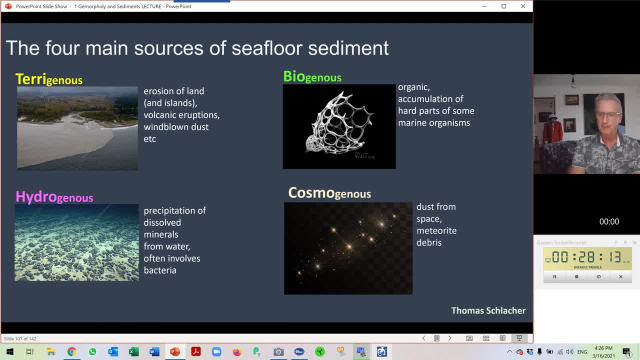 into smaller particles of silt and clay. that is one of the big, big sources of sediment to the ocean. So basically, the land is crumbling away. That's why you shouldn't actually study terrestrial ecology And making, and making the oceans. 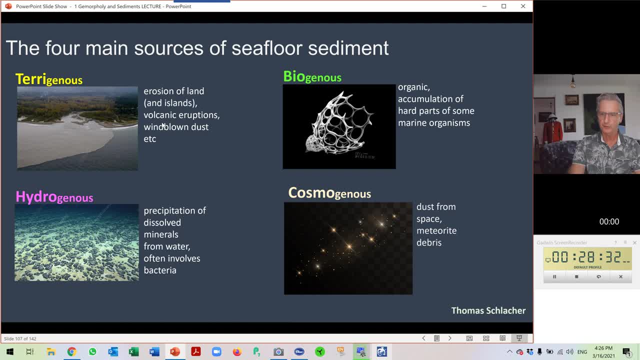 richer in sediment. A little bit comes from volcanic eruptions or from windblown dust, as I have just shown you. The other major source of sediment are biogenous sediments, And basically every cubic metre of seawater will contain thousands and thousands and thousands. 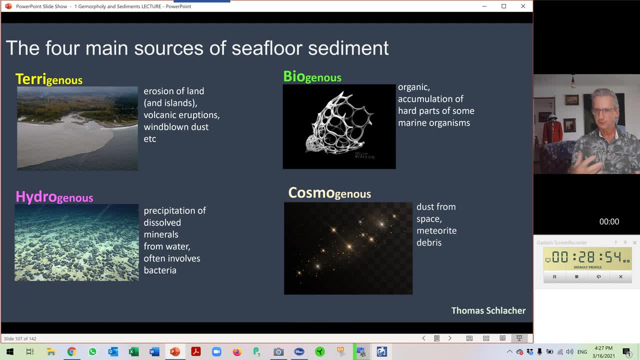 of unicellular little organisms called phytoplankton. Some of them are zooplankton, but never mind about that distinction right here now. But essentially they build unseen to the naked eye. you need a microscope to actually have a look at it. 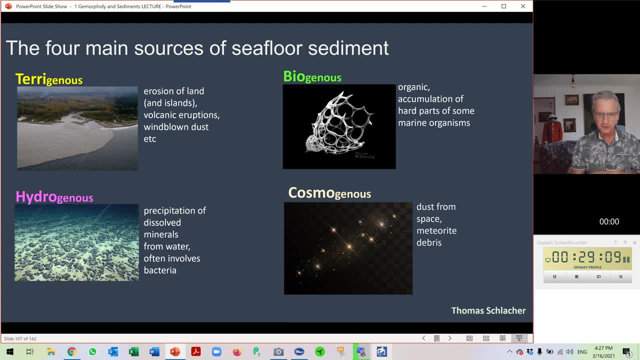 quite exquisite skeletons, And those skeletons come in all different shapes, forms, sizes and so forth. And when the organism dies or gets eaten by a zooplanktonic organism, such as a copepod coming along or a little fish, 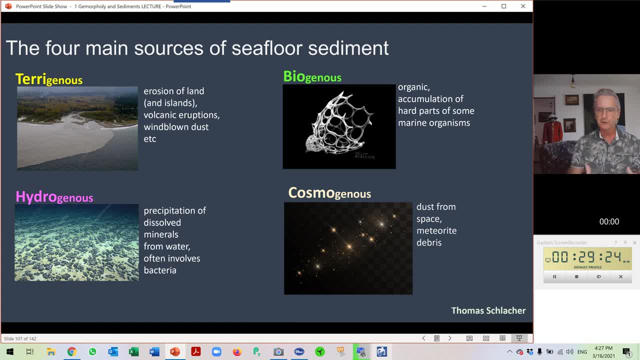 essentially, they sink to the bottom of the sea And the skeletons form sediment. They are particles. Now, it just happens to be the case for us. we are a very curious species because, engineering-wise, we power ourselves forward through controlled explosions. 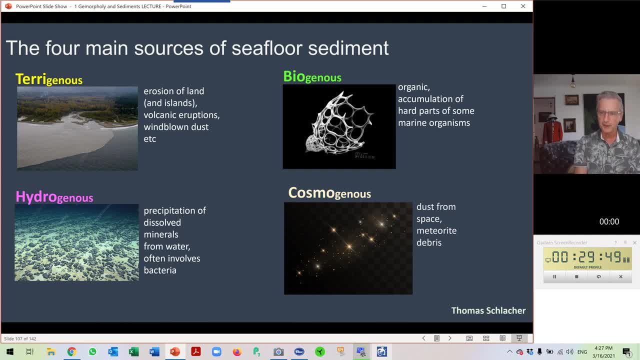 which are fuelled by the organic remains of those organisms. What do I mean? If large quantities of those biogenous sediments settle out to the bottom of the ocean, their organic remains can be so large that they form oil and gas reserves under the right conditions. 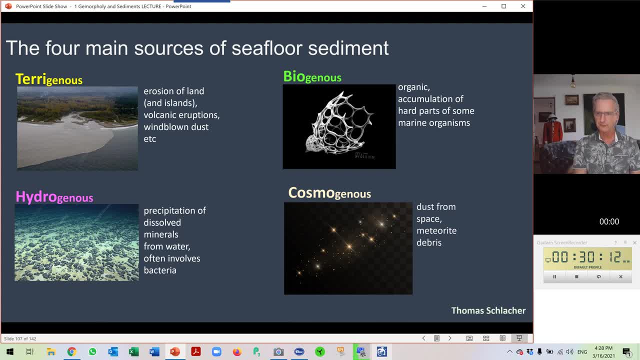 And we basically pump them up and voila, we use them in internal combustion engines, which is basically just burning dinosaurs or thousands and thousands per minute of the organic remains of those organisms. We have a very special class of sediments called the hydrogenous ones. 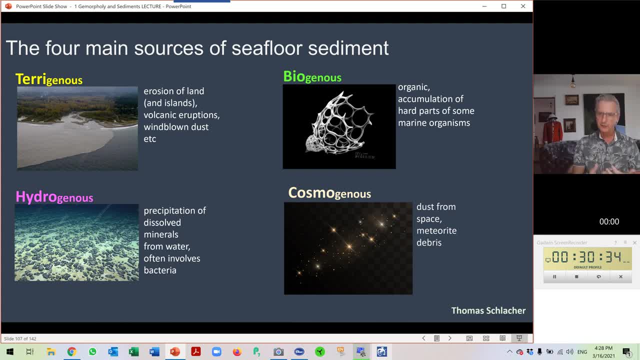 And that is basically chemicals forming crystals or other curious bodies. and we get to that in a second And that actually happens as a direct chemical reaction from seawater, sometimes under evaporative conditions, such as in a very shallow lagoon in a hot climate. 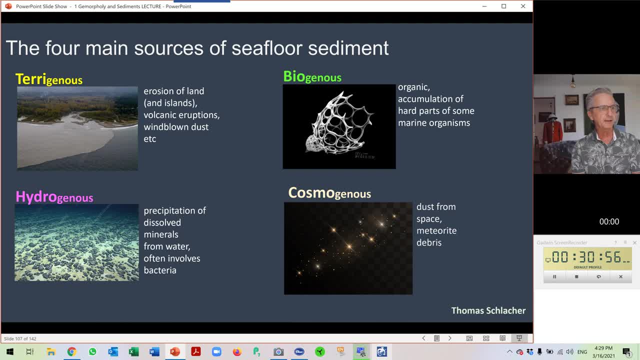 Or we use them basically to make salt. And, last but not least, you know we all have to be a little bit mad to be a scientist, so I often blame it on cosmogenous sediments, And that is basically as we sit here. 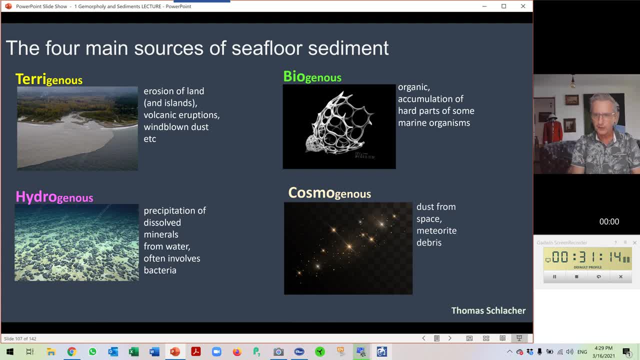 we are continually being rained upon by a steady supply of fairy dust from stellar space. We've got micrometeorites, but it's basically all sort of debris from space falling onto the Earth. Now the volumes, of course, of cosmogenous sediments. 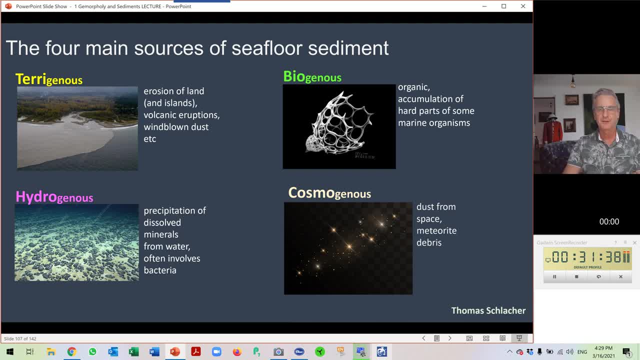 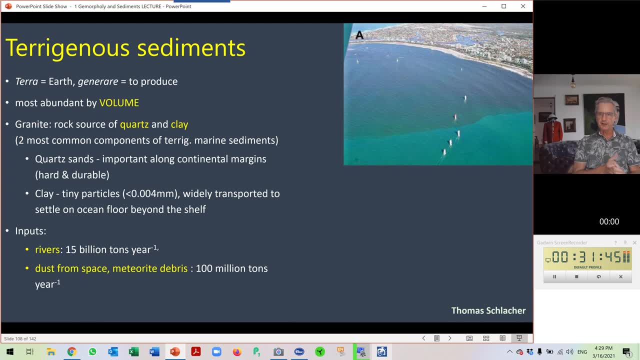 are not very large, So it's good for that, But they are there, so we can't really ignore them. Now, when it comes to land-born sediments, the hydrogenous ones, we don't have to look very, very far. 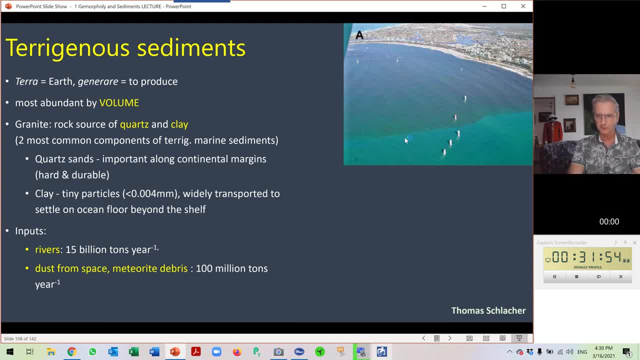 You basically spot how the process works. This is Mooloolaba here. This is a photo I took from a little plane. Here's the boats coming back on a Sunday afternoon And you see this huge sediment plume coming out of the Moolooloa River. 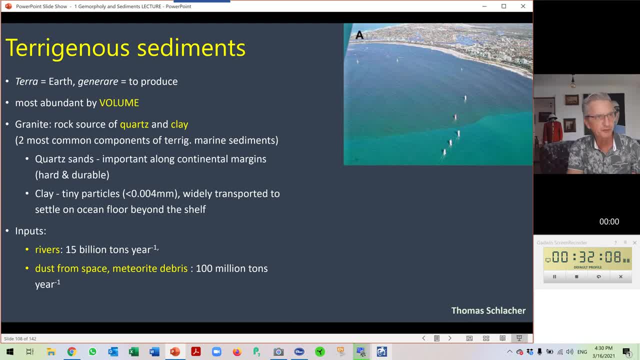 Now that sediment would have come from somewhere up from Mullaney-Kennelworth, probably up that way, or the catchments further down to the coast where all the suburbs are being built. But you know we can't really say that. 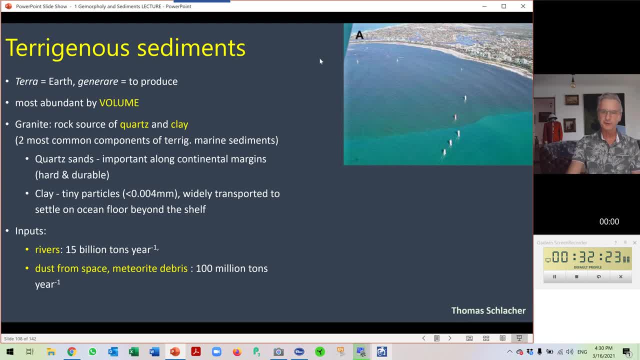 And essentially it gets washed out to sea. Most of it actually settles out on a continental shelf here, But some of it will actually be transported further offshore, mostly to fall off into the abyssal plains located about 20 kilometers offshore from the coast here. 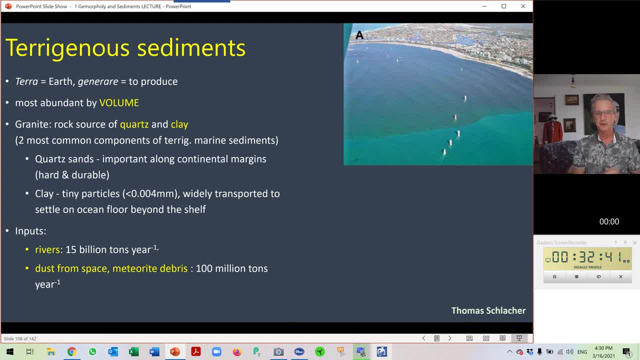 Rivers transport large volumes of quartz sand into nearshore oceans, But also they transport fine, small clay particles. There are smaller than four micrometers, which basically means they can travel hundreds to thousands of kilometers right into the middle of the Pacific Ocean. 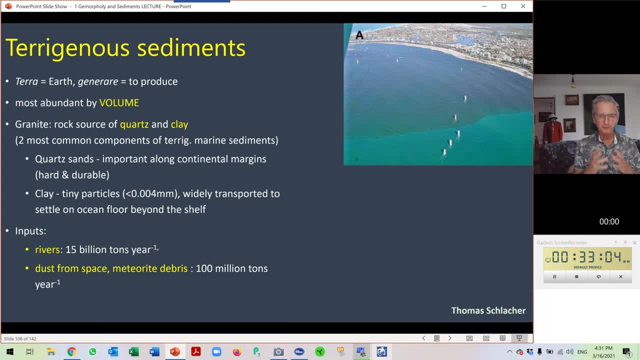 And the amount of sediment reaching the global ocean every year is staggering. Think about the figure now: 1,515 billion tons per year. It's incredible. If you think about that, you know the Earth has existed for you know. 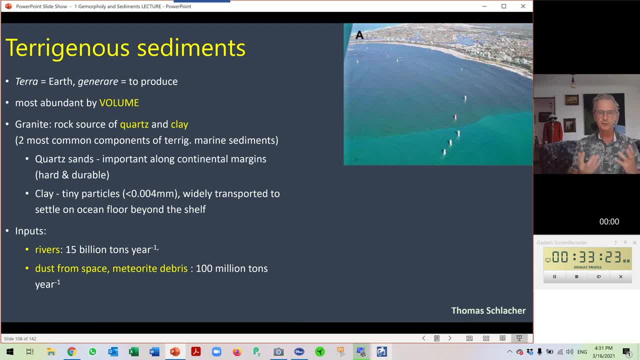 four billion years or something around there. To have that massive amount of particles coming from the land delivered to the ocean every single year is mind-blowing, flamboyantly mind-blowing. Now you can also, you know. 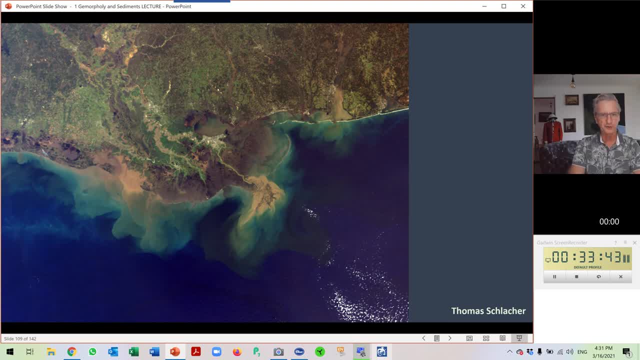 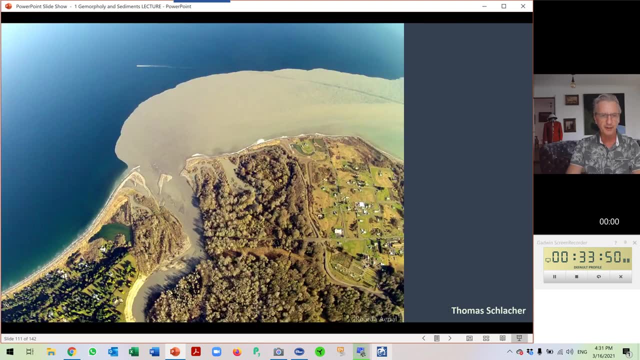 poke around the Internet, hunt for images of river blooms, and there is plenty of them. It doesn't really matter where you go. Here is one from southern Spain. Here is one from New Zealand. No sheep here. There must be some somewhere on the farmyard here. 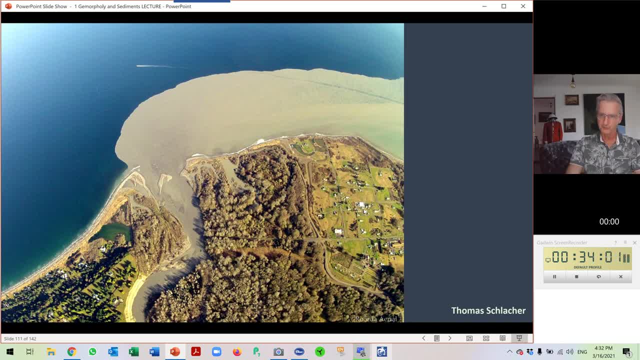 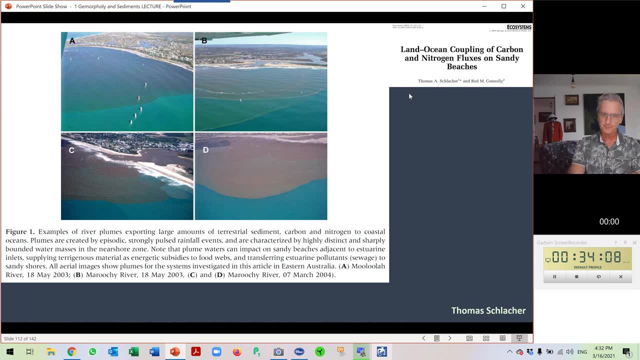 Transporting half of the island straight out into the ocean, And of course we know a little bit about that because a few years ago we ran quite a big project on the land-ocean coupling being achieved Here, one coming out from the Mooloola. 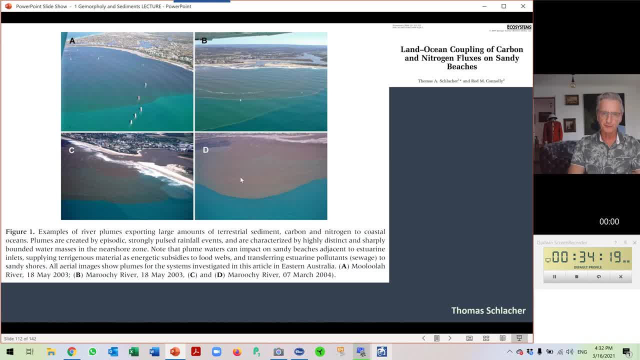 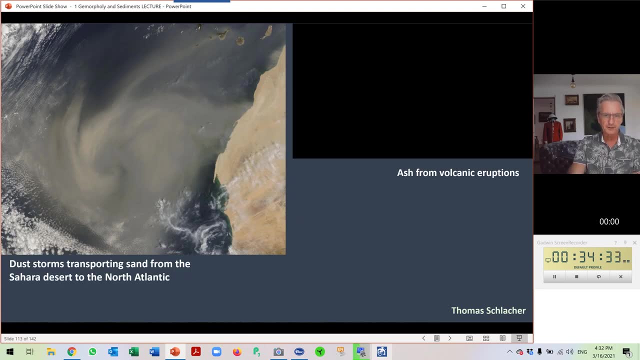 and those are all blooms coming out from the Mauritius River, And notice how incredibly distinct they are. They don't actually mix very readily, and that is actually a consequence of density differences, mostly as a result of lower salinity. Now, we already talked about 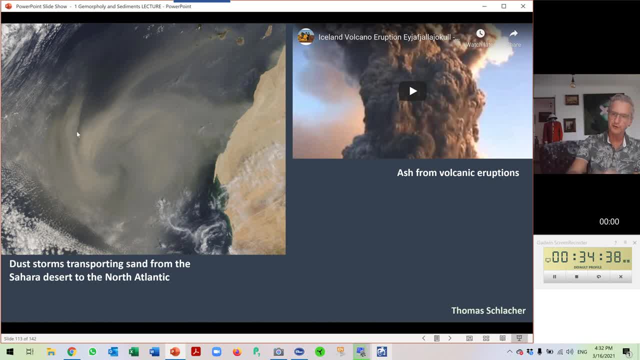 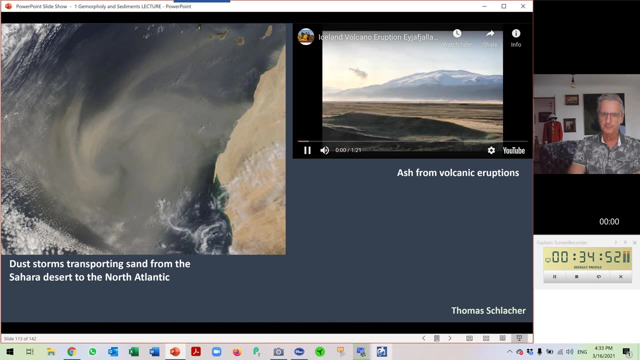 the sand being transported by sandstorms from deserts. Here is another example of one of those massive sandstorms. Here is the Canary Island. This is West Africa going off into the North Atlantic. Now a few years ago, we had a very large 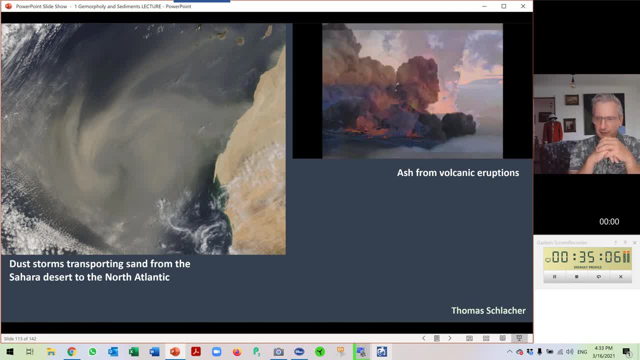 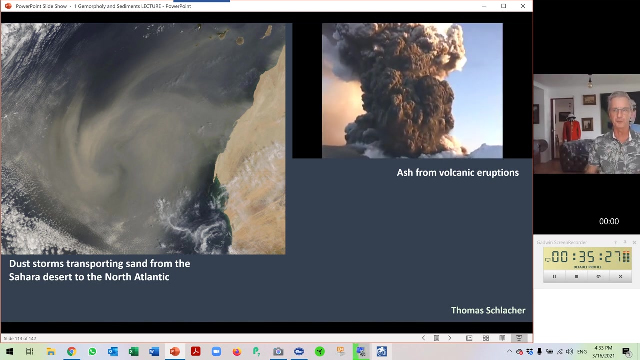 volcanic eruption in Iceland and that delivered massive amounts of particles into the atmosphere to the extent that it basically led to long-term- I think it lasted for half a year- disruptions of the European, North European flight segments. It also basically was the case in Bali when we had that. 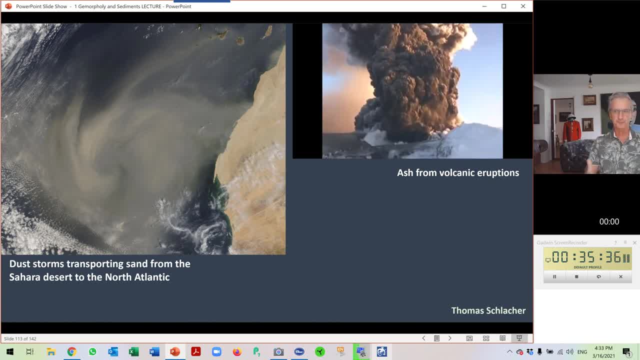 So over many, many, many months we actually saw that atmospheric loads of particles being too high for safe operation of aircraft, Eventually they cleared. of course the skies cleared and they cleared because the particles set it out and many of them would have. 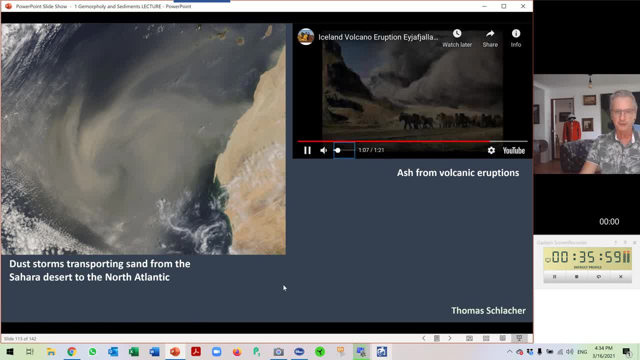 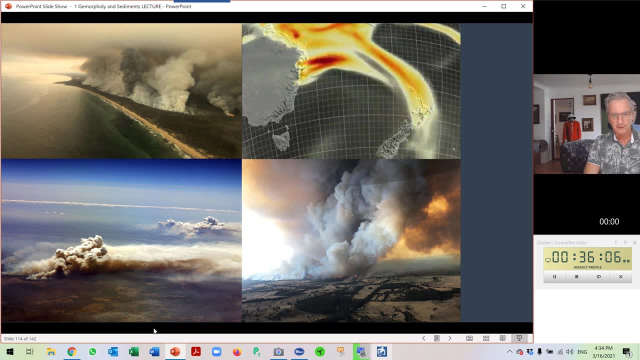 landed up in the oceans. Aha, there we go Now. a few years ago, when I did this lecture, until I should say, literally about two days ago- let me adjust the camera, sorry. It was a case where I said: 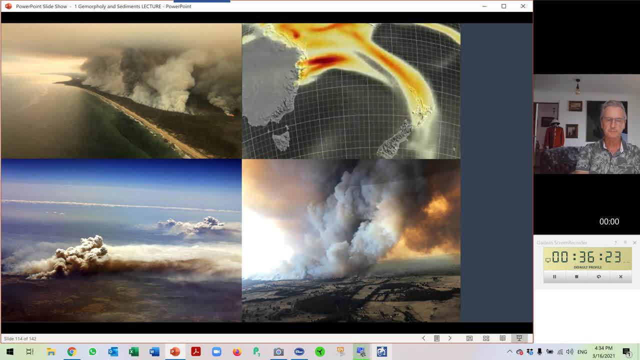 look, you know it is kind of curious that we have little fires in Australia and you could see those streaks right of more or less dust, you know, wandering over to New Zealand. Now that actually has changed very dramatically since. 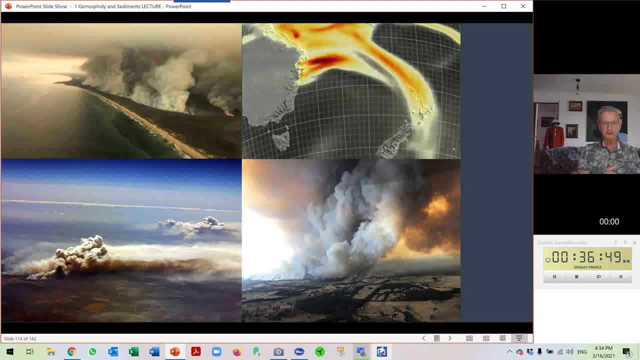 you know we had those massive bushfires in New South Wales and Victoria And you look at this imagery and it is literally frightening. And it is frightening not only displayed over how many thousands of kilometers one can actually feel an influence or an impact. 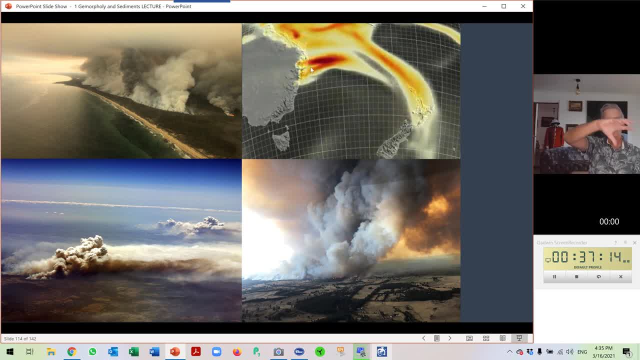 of those bushfires. Look at this top right image here where the bloom basically goes up And it is like a line that goes up and settles all the way over the northern part of the north island of New Zealand And also, you know. 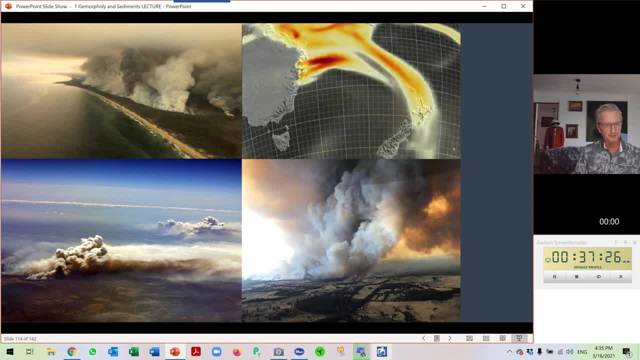 you can actually be a little bit of a- you know, maybe a liberal party supporter. You have to be quite careful with what I say now, like Thomas, I didn't say anything. I said you could be, And even if you would be. 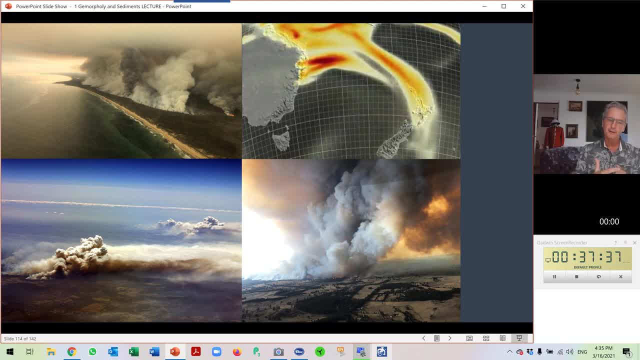 you know, sitting in Parliament holding a lump of coal. you know, and you might not actually read your dossiers. you know, and you may not be in a position where you could actually be a liberal party supporter dossiers. But just look at this imagery and I think if you still, then actually 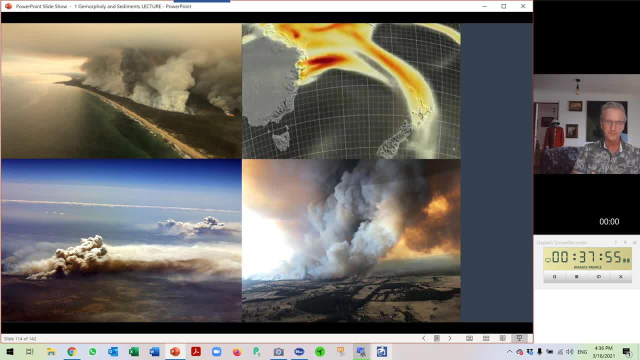 go on and deny our children's generation a safe and secure climate to live in. I think you must actually be a little bit blind even to powerful imagery like that, And it's quite odd that nowadays we find ourselves, you know, learning about ocean. 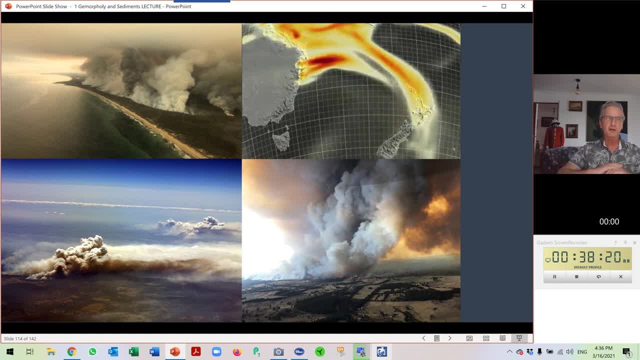 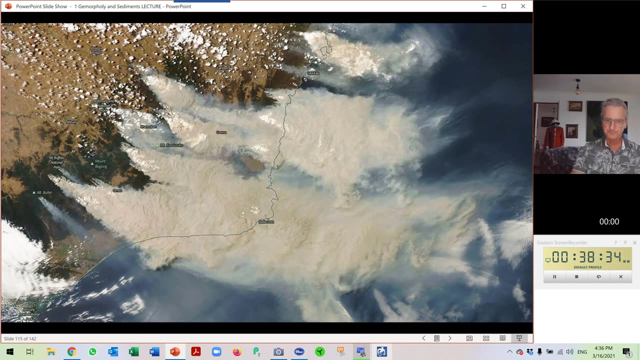 sediments and talking about bushfires. Who would have thought about that? I would have never thought about that, you know about 10, 20 years ago. But that actually illustrates how very, very acute the need for climate action is Right. And here's 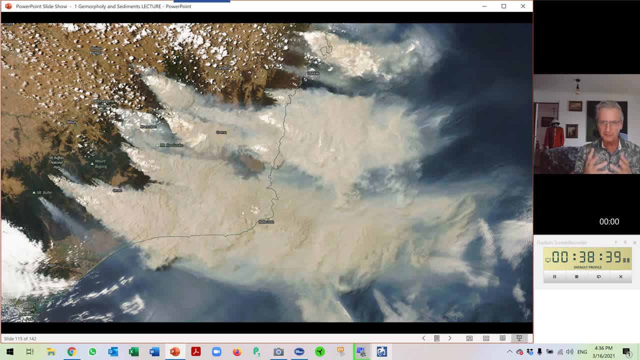 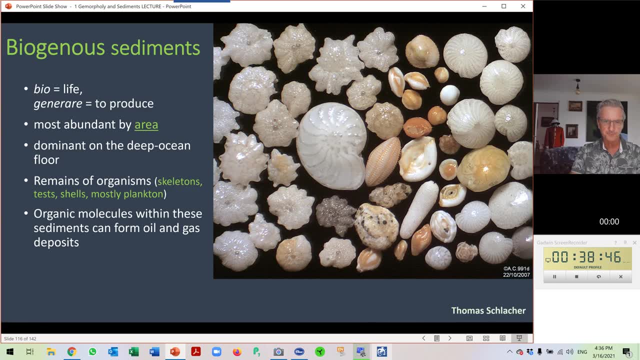 another you know image here. Look at this massive, you know smoke clouds And they're actually full of very, very fine particles going into the ocean. Now, some of the coolest sediments God come from the remains of organisms. 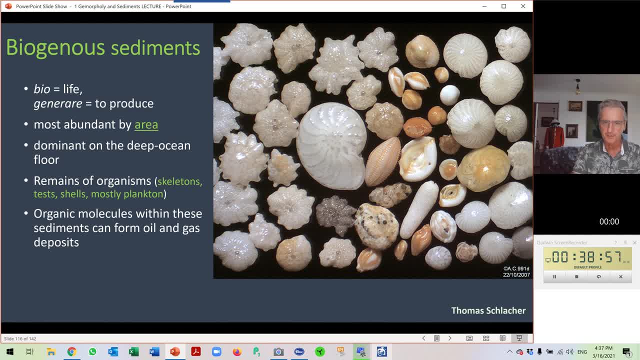 Now what you can do is you can literally scoop up you know a little timber of you know beach sand and then put it on the microscope and use a very, very fine needle and you can sort them out And you will find all those little remains. This: 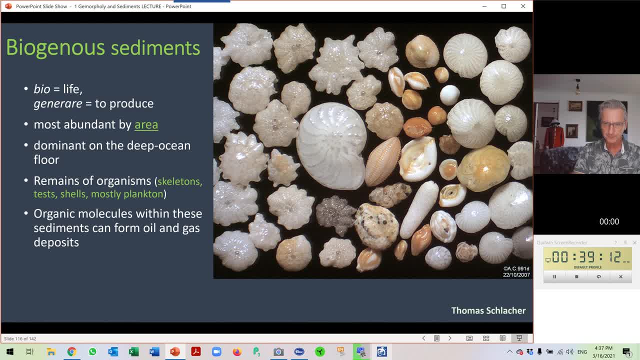 is mostly for minifera, in that case, making up the sand. Now, this is actually very, very cool. I mean, basically half our ocean is covered with skeletal remains in the cross-cilium. Now, what actually happens here on those ones is, as I explained already, each of those organisms. 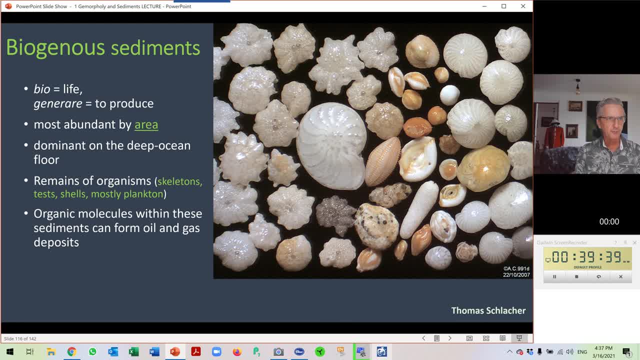 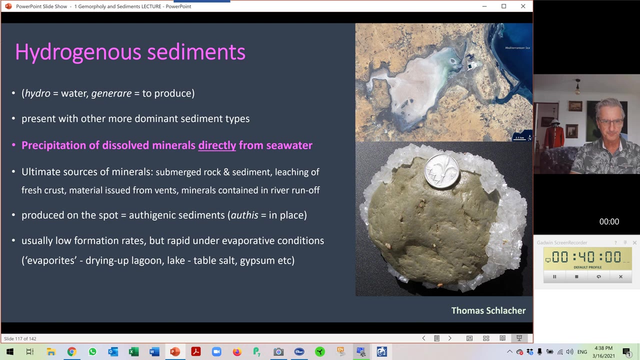 originally contained organic molecules, Each of them, you know, predominantly being some sort of carbon molecules or another, And, of course, under conditions where there is sustained pressure and then burial, they can form gas and oil deposits which we now extract from the deep ocean. 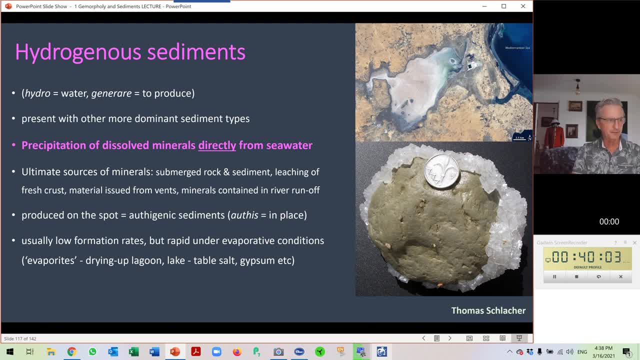 Right, Here's a curious one. I always wonder why people go off and buy very, very expensive Himalayan rock salt. Right, Here's a curious one. I always wonder why people go off and buy very, very expensive Himalayan rock salt. 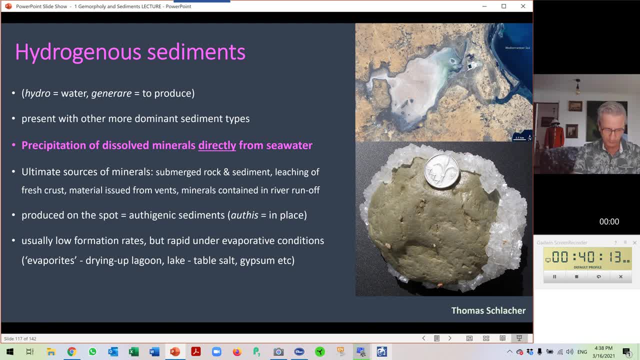 If you really really want to do a low-carbon footprint, go and make your own salt. Take a bucket of water and boil it down- preferably using some solar-powered system, of course- And you have then a perfect evaporite, And we use this in salt pans the world over. You basically have a shallow, you know swimming. 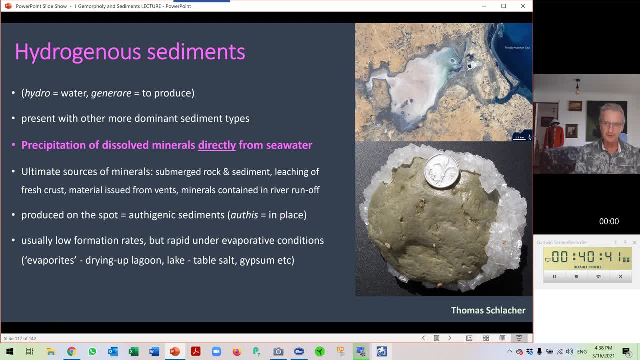 pool a meter deep. I actually made you know my very first celery came from working for half a year in a salt pan. Very, very curious. And the odd thing is, nobody would actually eat any of that bio-salt if they see what actually comes out from it, because lots of animals actually fall into. 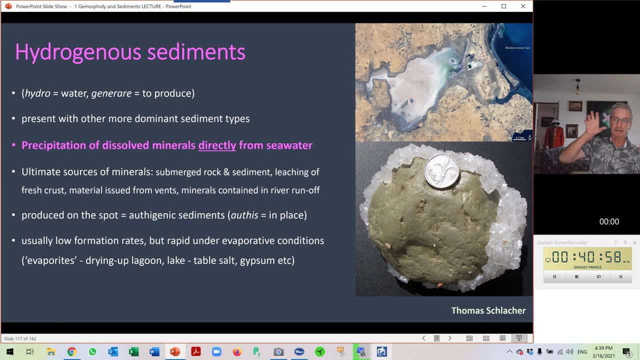 it and they just get mummified like baboons, antelopes, you know, kind of like that- Well, not quite like that, but you know you get the drift. And here we actually see some gypsum being crystallized out on a rock. 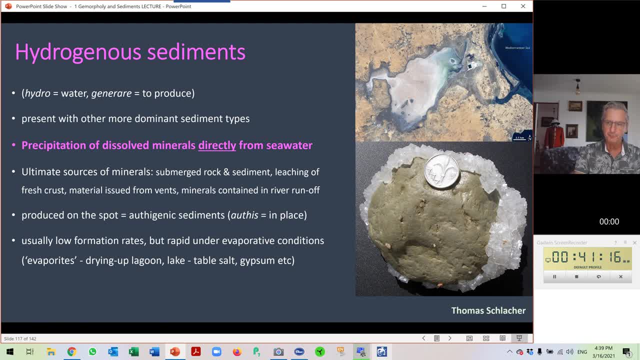 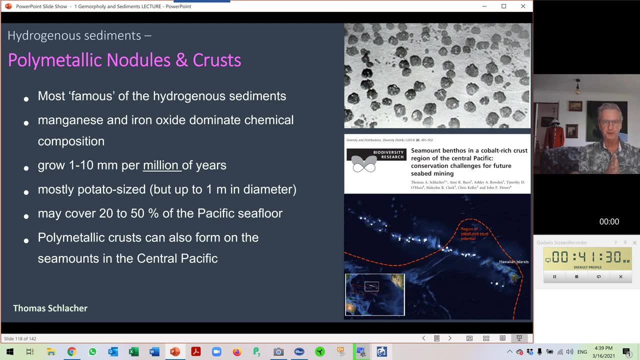 But- and that actually happens- in lagoons which dry up, Lots of the gypsum deposits in the world come, you know, from those kind of very, very hot areas. However, the coolest ones come from the Pacific. Now about 30 or 40 years ago, on the first dives in sort of the central Pacific between 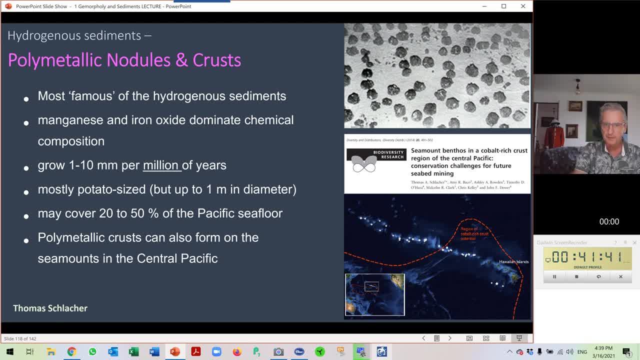 Hawaii and over towards, you know, Mexico. Wow, People stumbled across those weird potato looking things on the seafloor. Now, that was not an Irish ship which lost, you know, its cargo, all the black potatoes. They covered a size probably the size of Australia. Now, this is very, very odd. And what actually? 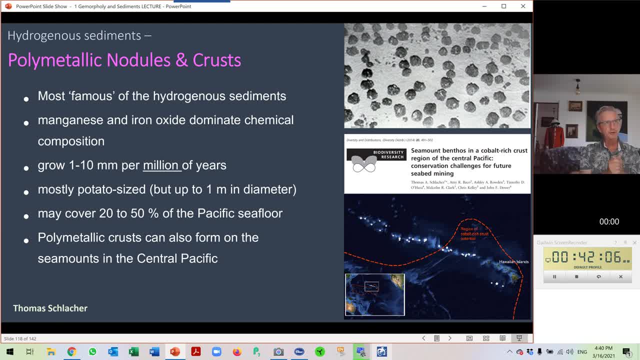 happens is under those particular chemical conditions in the central Pacific, central Pacific, Eastern Pacific. there we have precipitation of minerals in a very, very unique makeup. They come either in the form of those nodules or they come in the form of a crust forming. 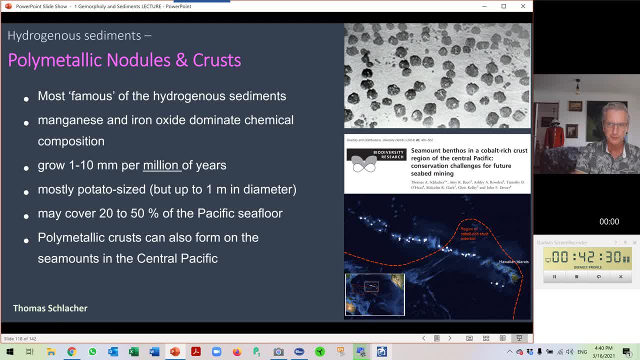 over the top of those sea mountains. those mountains And are called polymetallic nodules or polymetallic crusts, And the curious thing is- air how widespread they are and b how valuable they are Now, when I actually started to talk to geologists and we did some work there, as you can see, not terribly. 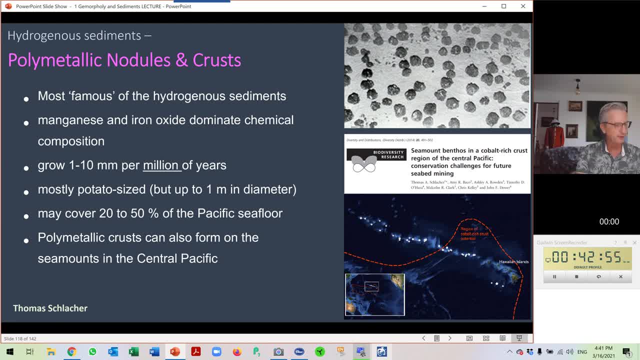 long ago, 2014,. feels much longer now, but basically they said this is a mining person's dream to come so that contain all the rare minerals particularly used in, you know, very advanced in a metal fabrication, which are usually very, very hard to find, so that process concentrates them in a deep sea. Here's: 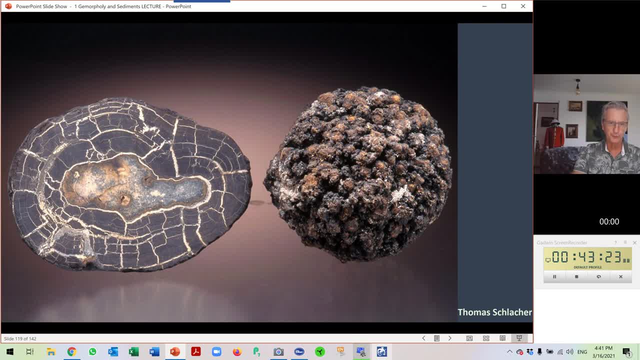 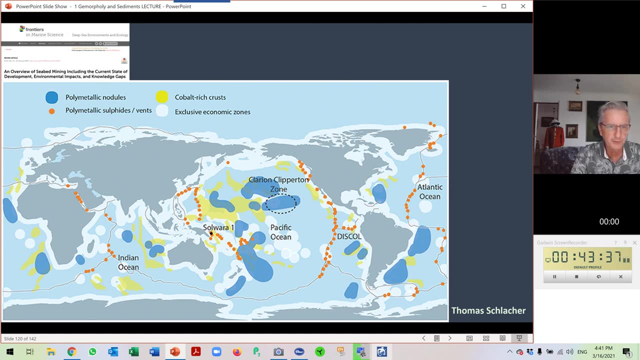 one of those polymetallic noddles they used to call manganese noddles, but they basically, you know, contain all sort of minerals which everybody wants. Now that came out, I think this year or last year, and we used to talk about those things not terribly long ago. 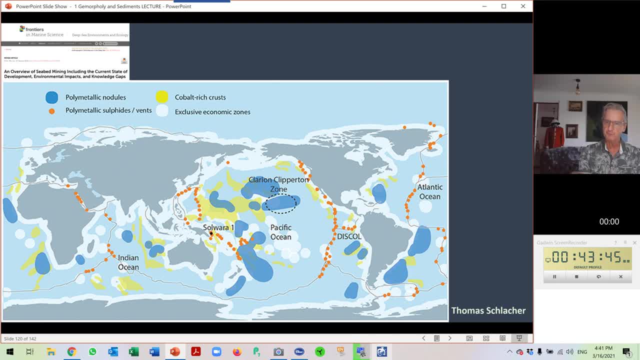 five years ago people said oh, yeah, yeah, one day, you know, we might actually go and mine some of those things. we might start, might we might mine some of those. you know vent chimneys and they are right in our neighborhood by Australian companies. or you might go off and basically do the cobalt which crusts right, or the 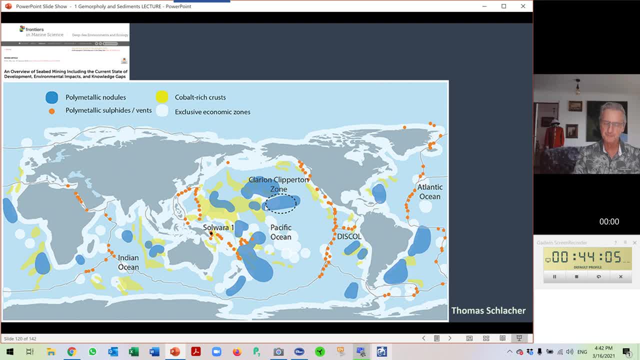 polymetallic noddles, whatever it may be, and technology is so rapidly advancing that now we actually are in a situation to having to decide who actually has the exploitation right and how can we have a little bit of an influence of actually making sure it is not complete wanton environmental destruction. and that's the 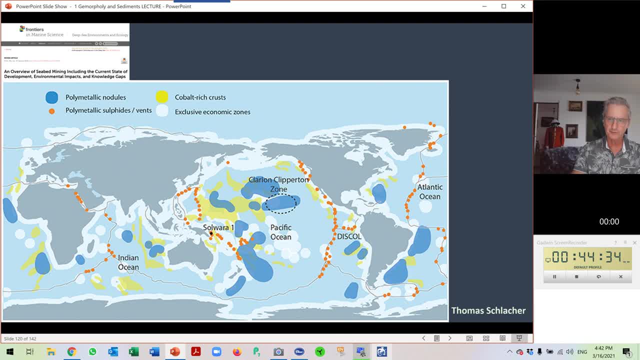 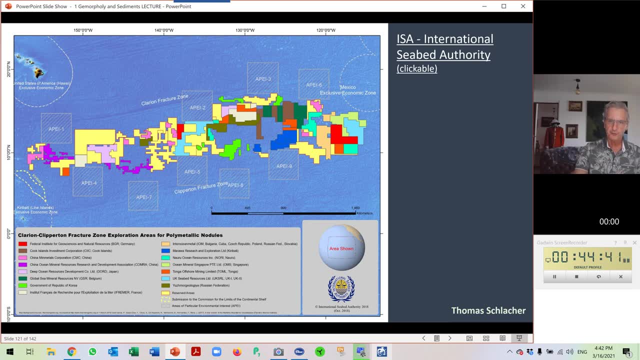 same problem we have actually on the land. this, you know- terrestrial dry mining. Now, and this is actually no secret, you can actually go on the website of the International International Seabed Authority and this map comes straight from there, and it is astonishing that we, as a global society, have already started. 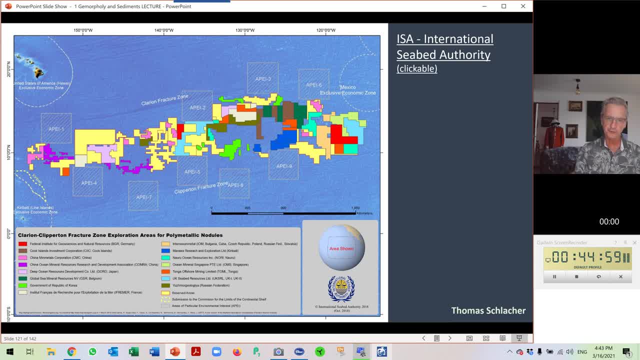 to hand out mining leases right to countries in what is called the Claring Clipperton Fracture Zone. This is where most of the mining is done. This is where most of the mining is done. This is where most of the polymetallic noddles sit, and what is really really amazing is: you can see. 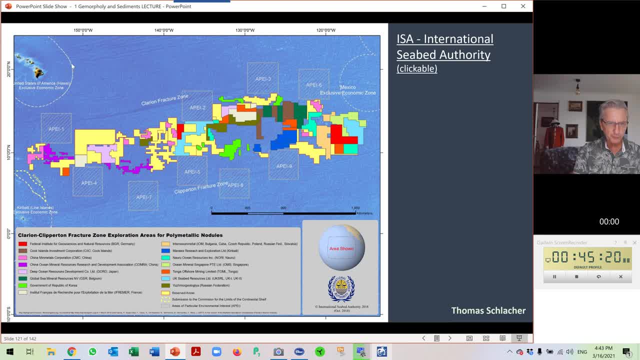 it sits completely in international waters. This belongs to the US, This is Hawaii, This is Kiribati, This is Mexico and basically, it is the United Nations task, particularly the international, more specifically the international Seabed Authority, to regulate the use of natural resources on what we call the 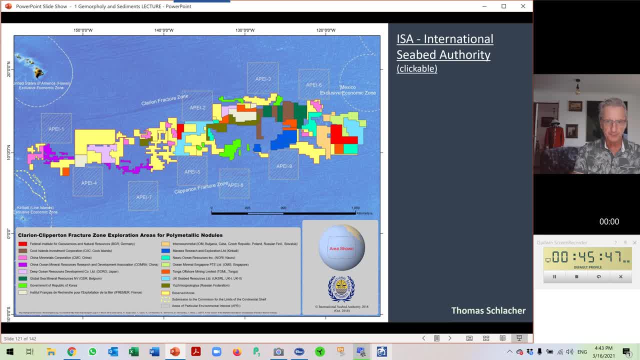 high seas. Now, the high seas happen to be, you know, everything which lies outside the exclusive economic zone. Now, what is quite curious here is that the environmental areas all sit outside the prime mining area and of course it is a bit like saying you, I make a national park somewhere. 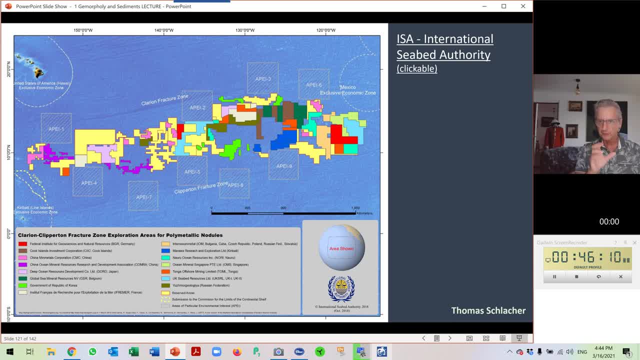 But you know not quite really where it actually should be. ie, every conservation area should have as one of its criterion the need to be representative right And if I actually talk about you know, things being thousands of kilometers on either side, it is probably fair to say, and this is what I was. 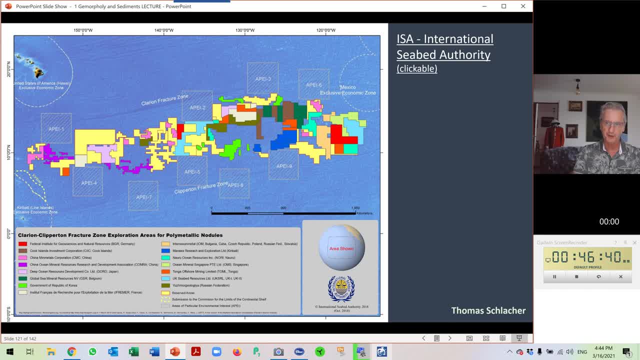 trying to say: So what is also interesting is this: this was sort of the images you saw of the sea mount, So this is actually very, very curious. It is actually saying, yeah, where are we actually putting spatial conservation zones in? But they are all outside the mining. 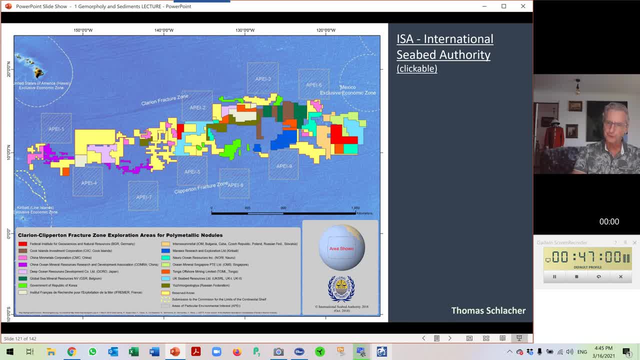 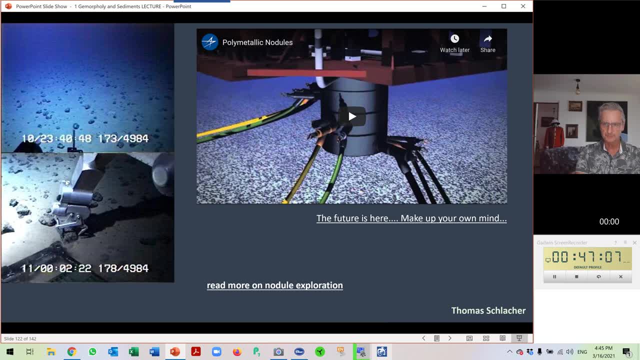 places. So what is also interesting is this: this was sort of the images you saw of the marine resources. So this was sort of the images you saw of the marine resources And these are all sort of the ones that you see now in Richard in your mind. so 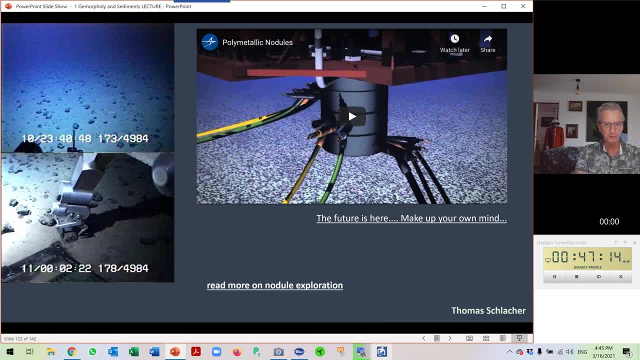 And I hope I get that- you give it a risk and simply given it a more technical answer À la het zou ki en listing be hell. I want to try this again. So this is how what I was talking about. So as to the team I was talking about, 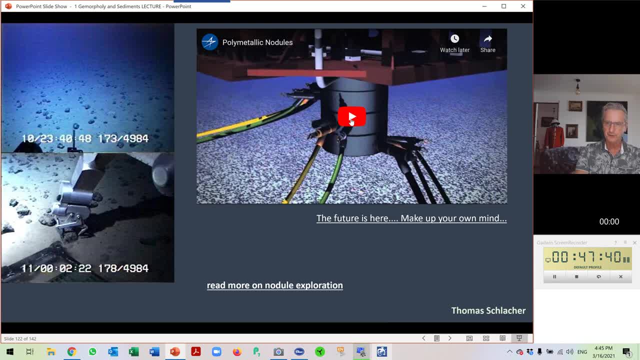 13. fight striker, basically working for the UK government or under, I think, the permission of the UK government, so like, oh look, this is what we're going to do, so watch this. I leave this really to you before we move on, to basically make up your own mind. of course it's. it's a promotional 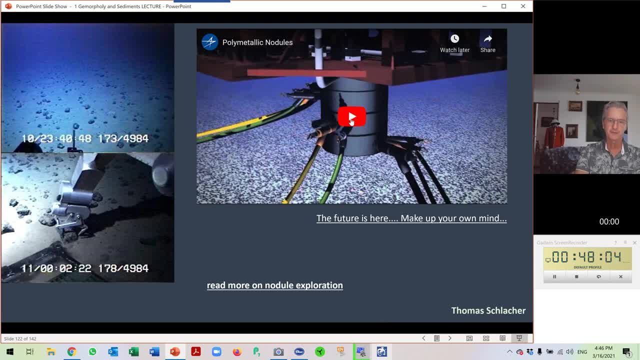 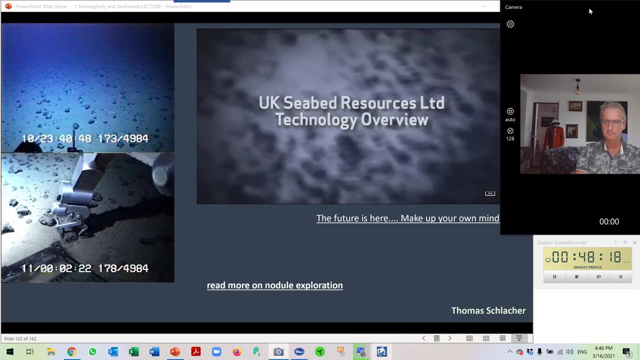 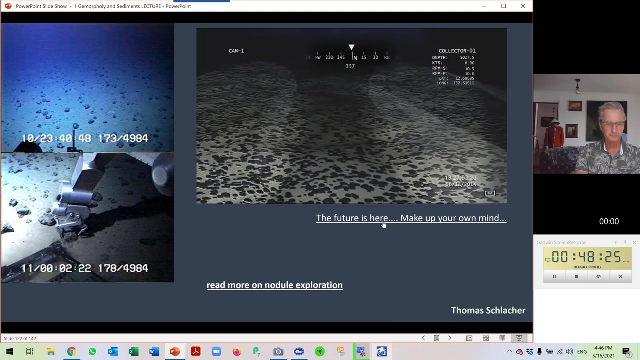 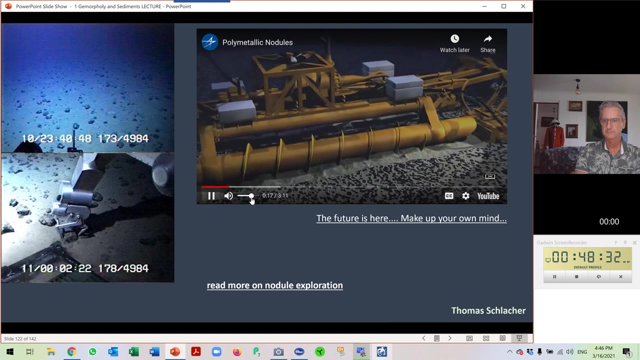 video, but what actually is important, that it is something most people don't know and yet it's actually publicly and presently out there. UK seabed resources, a wholly owned subsidiary of Lockheed Martin UK, will assemble a deep seabed manganese nodule recovery and processing system using low-risk, commercially available equipment and technology. the company 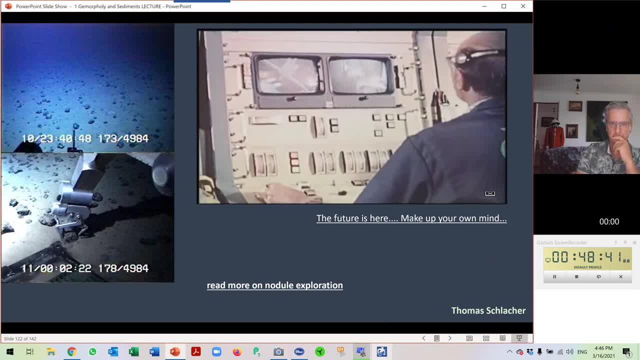 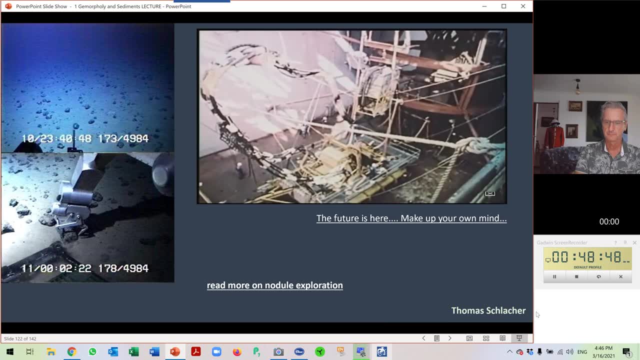 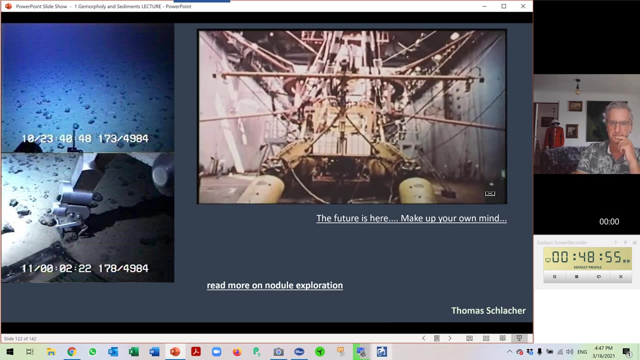 will draw on its parent company, Lockheed Martin, to leverage the system architecture from the 1980s. this was in part developed and proven by a Lockheed led consortium in the 1970s, which invested five hundred million dollars in addition to operational seabed experience. the 1970s work. 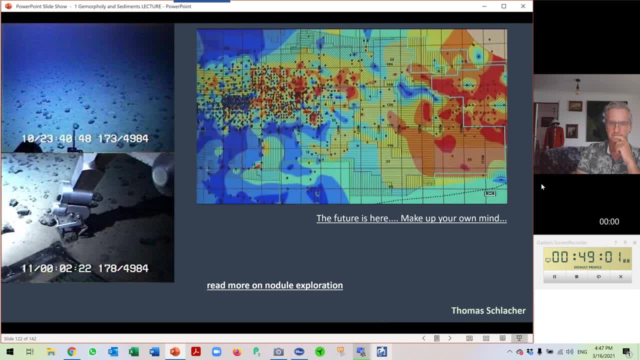 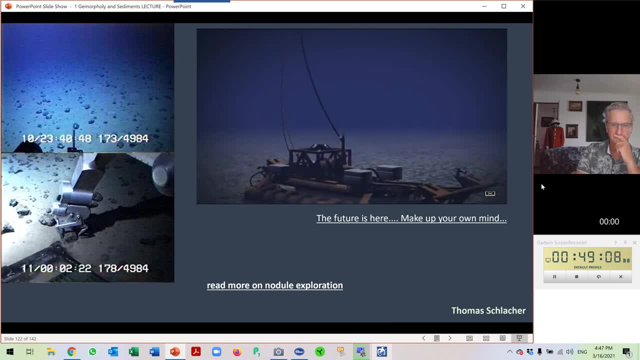 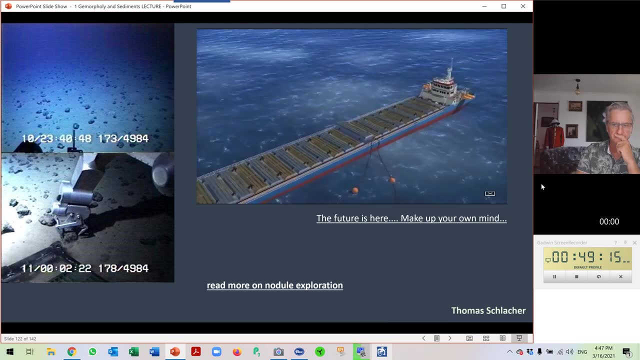 also resulted in the discovery of thousands of geolocal located nodule mineral samples. here we see a potential scenario based on applying modern technology to bring forward the legacy Lockheed Martin system. other alternatives will be evaluated in line with exploration results and environmental considerations, which are paramount. efficient sea 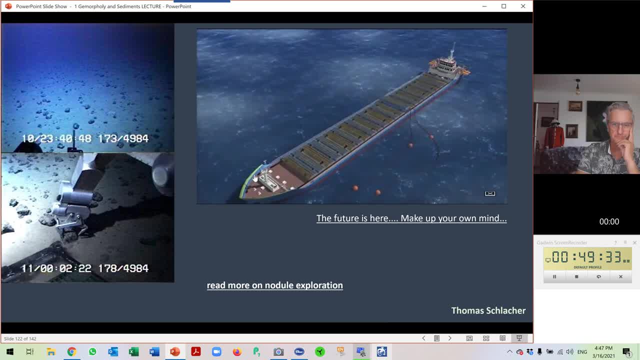 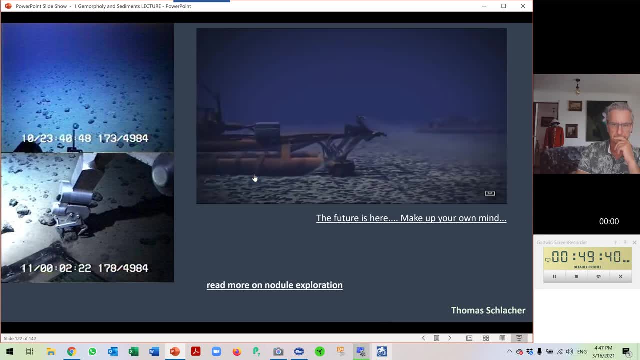 bed to surface nodule recovery could be achieved by multiple deep sea nodule collectors, slurry transfer lines and pump and state-of-the-art laser pipes. this process would deliver nodules to a surface ship, from where they will be transported to a metallurgical processing plant. multiple module collectors scooping the nodules from the 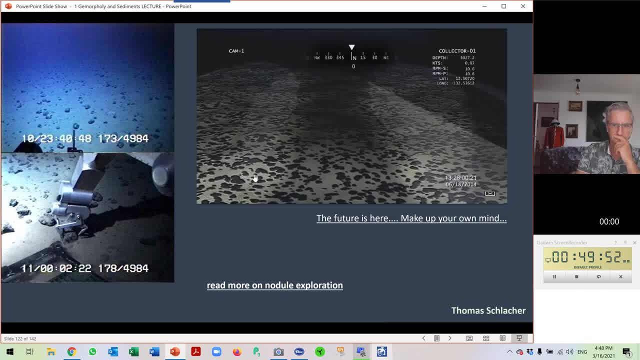 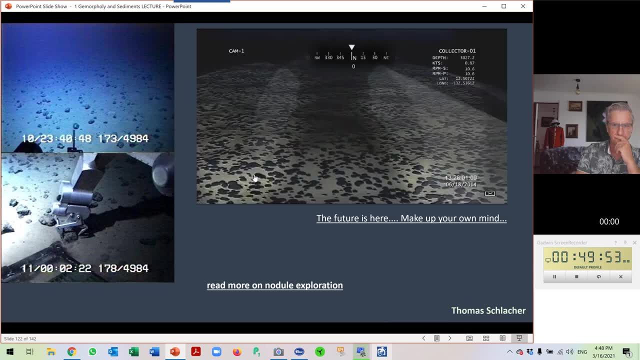 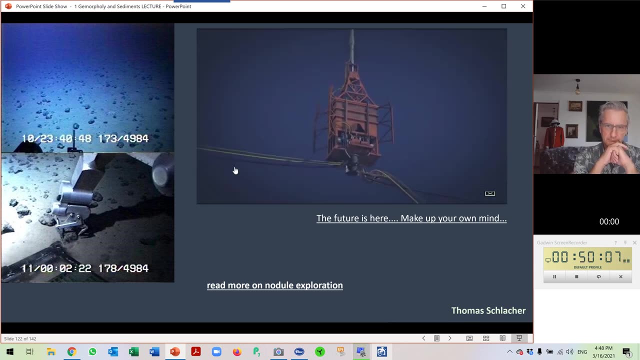 sea floor and transferring them as slurry to the central pump will be at the heart of the system. equipment of similar 100 ton size is already operational today for deep sea cable trenching and pipe lading deep sea vehicles already available can also be employed to connect. 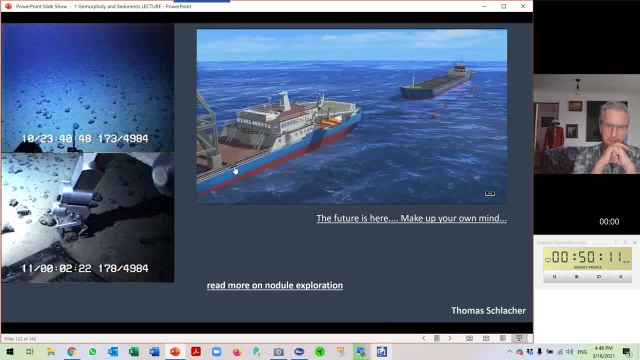 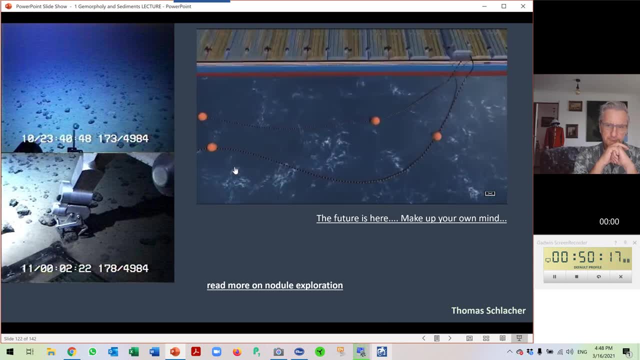 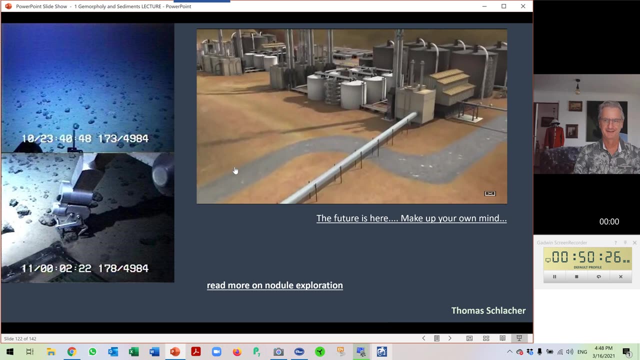 to the central pump. the multiple collectors and central slurry pump together provide a constant flow of nodules through the riser pipe to the surface. on board the surface ship, the nodule slurry is pumped to dynamically position bulk carriers for shipment to shore. the nodule slurry. 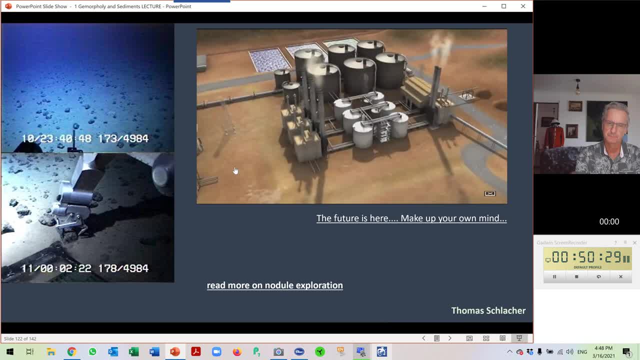 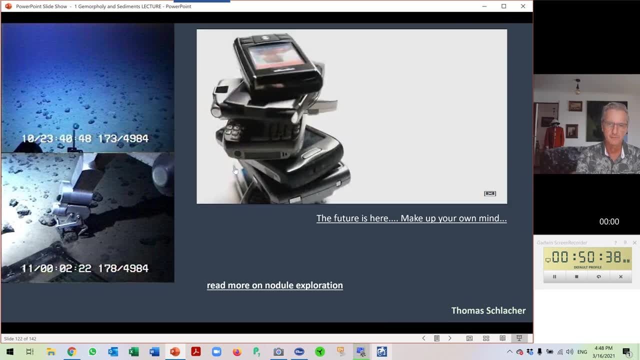 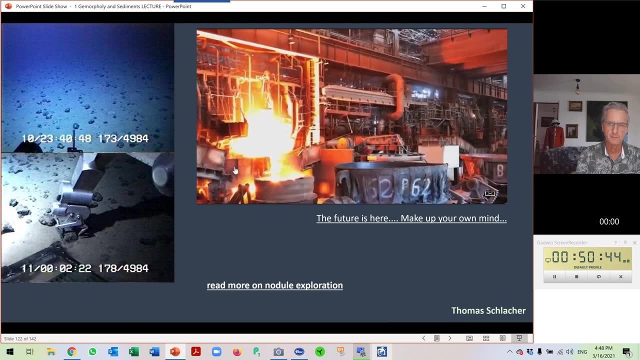 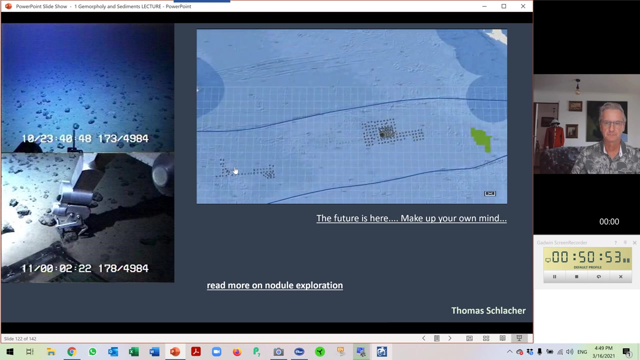 is pumped from the ore carrier into temporary storage ponds in the processing plant. well established metallurgical processing techniques are used to recover the valuable metals from the ground tools. the byproduct is rich in rare earths, which are in demand for high-tech applications, and also in manganese, a key component in steel production. UK seabed resources holds rights giving. 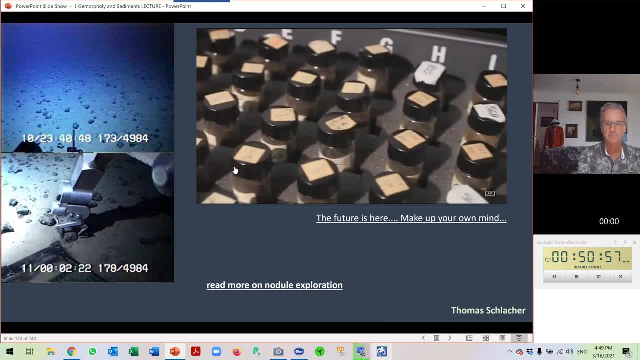 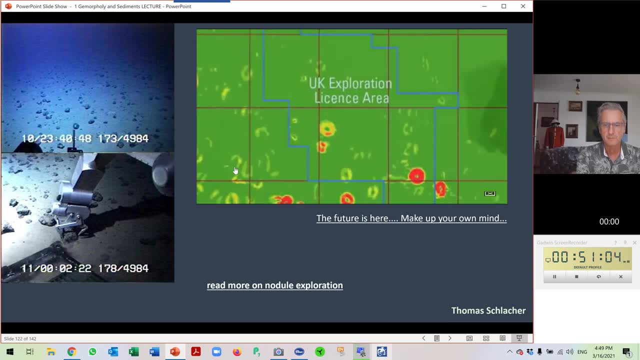 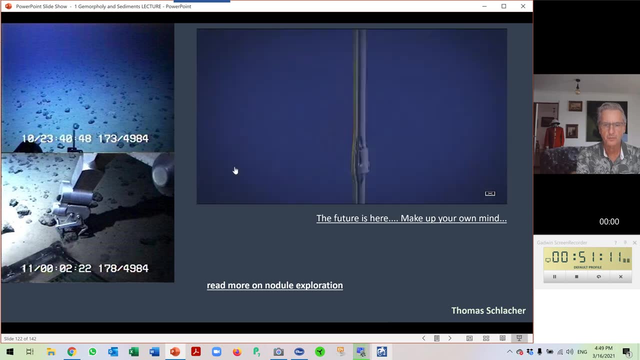 it access to parts of Lockheed Martin's collection of geolocated nodule samples and library of exploration data. this has been gained from across the clarion clipperton zone and provides a unique understanding of the manganese module resource. modern technology and processing methods enable UK seabed resources to implement environmentally responsible commercially. 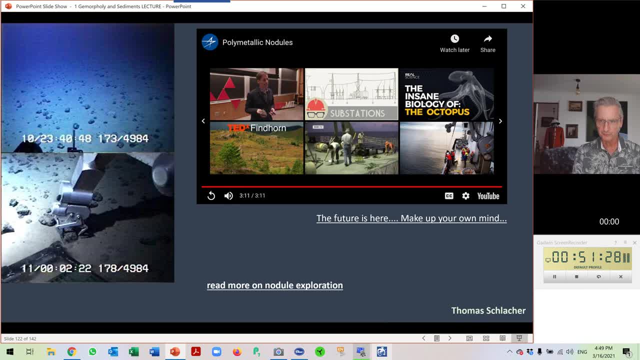 viable solutions which have the potential to benefit the UK economy for the next 30 years. so I should say nothing against the UK. well, it's not rugby or cricket time yet, but otherwise, you know you always have to sort of beat the pumps, but never mind. many, many countries actually have exploration rights and will actually have very, very similar. 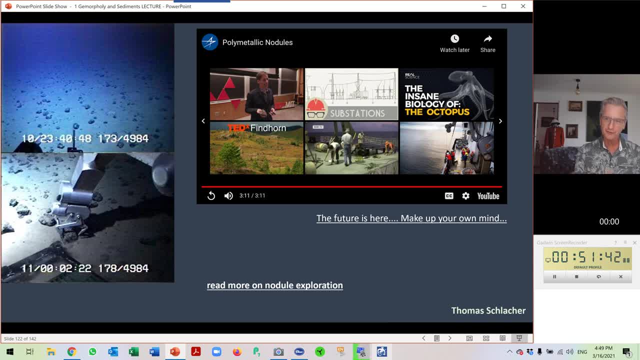 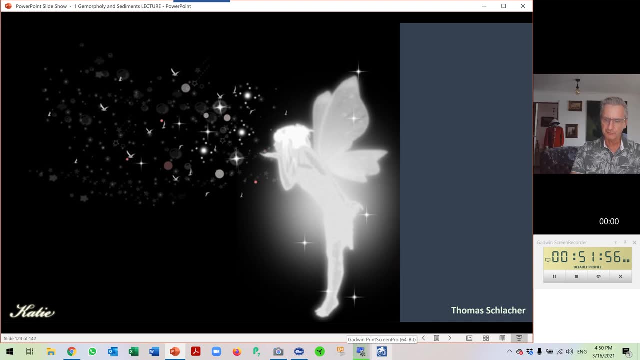 you know plans afoot. so this is actually just like a reminder for you, to poke you in the side and actually, you know, illustrate an issue which unfortunately not terribly many people know about. right, uh, here we go to the fairy dust, you know. if you have uh children, you know all about it. but 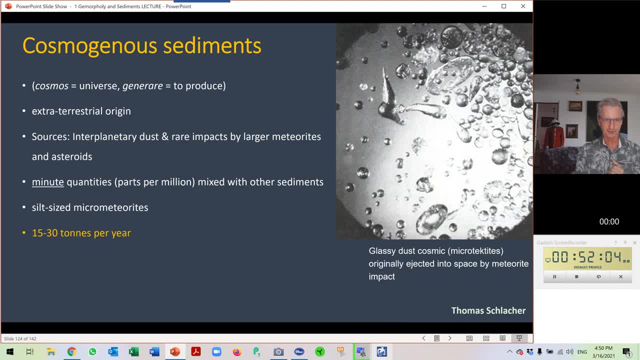 also it's real, but it really is quite cool. I actually think to have between 15 and 30 tons of fairy dust per year laying on Earth is actually a figure. I thought, uh well, I I didn't really think it was actually that much before I actually researched it. 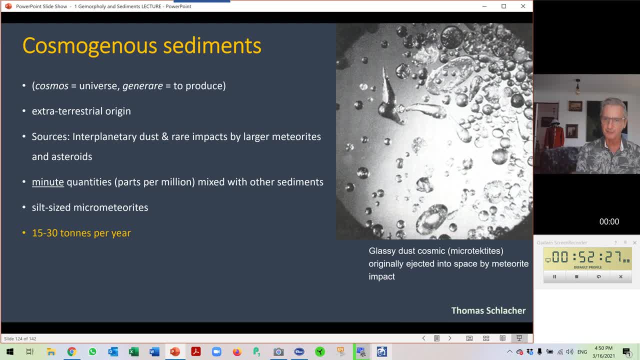 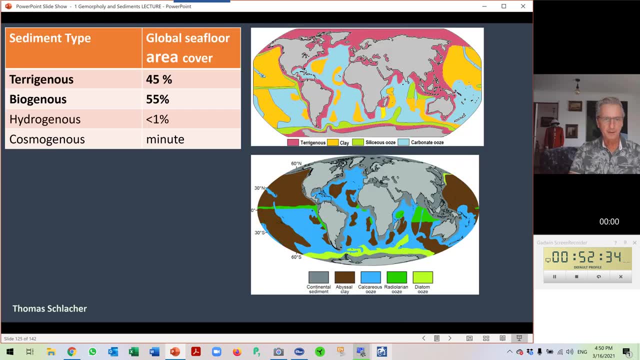 and days in every basically cubic meter of deep ocean sediment. there will be a little bit of that in it, right? you might say, okay, uh, which sediment type is you know the most? well, if you measure it, it depends how you measure it, if you do when. if you measure it by the area of sea floor covered. 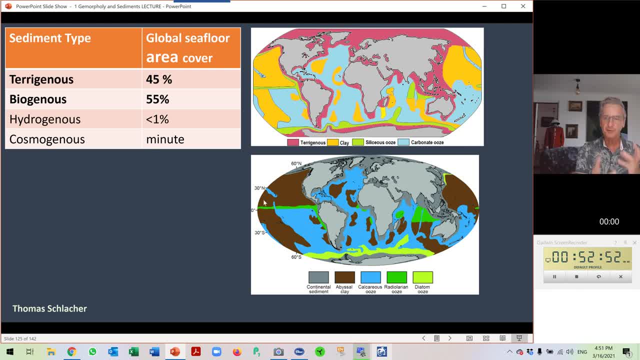 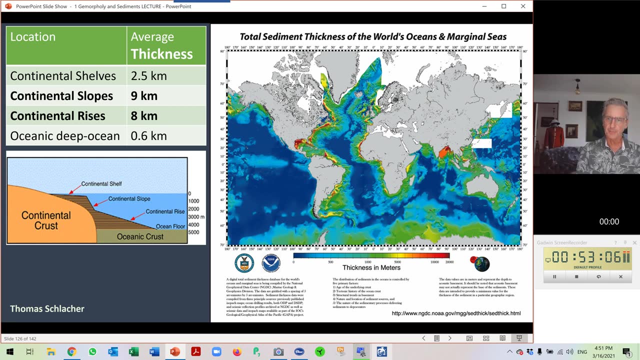 and you can actually come up with a map, something like that. it's about half half between the ones from the land and the ones made from organisms. the other ones are really just very minute quantities. um, if you, however, ask yourself: oh you know, how sick is sediment? how much is there? how high is? 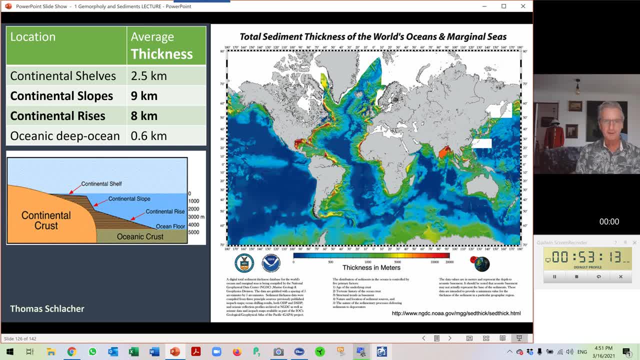 it tied up at the bottom of the sea floor. I think the uh, the answer is truly astonishing. it's kilometers, kilometers, kilometers of deep mud. you can actually download this in an incredible high resolution format: the total settlement sickness of the world's oceans and sea map. it's. it's fantastic. I mean, Noah the beginner. under Trump it became a sport really. 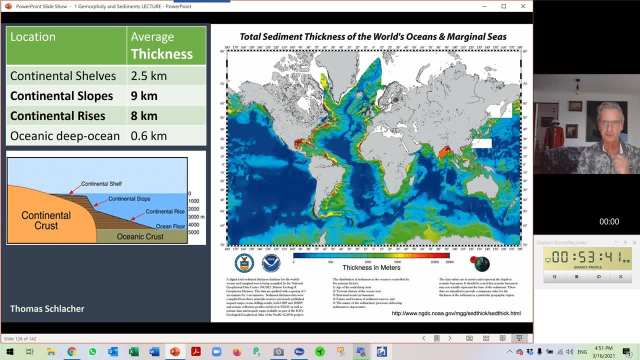 for everybody. it was a cheap sport and it was a justified sport to make fun of the United States, but the government agencies of the United States to do some really, really, really, really, really, really super wonderful work, and one of them is, uh, how they make publicly available some of the you. 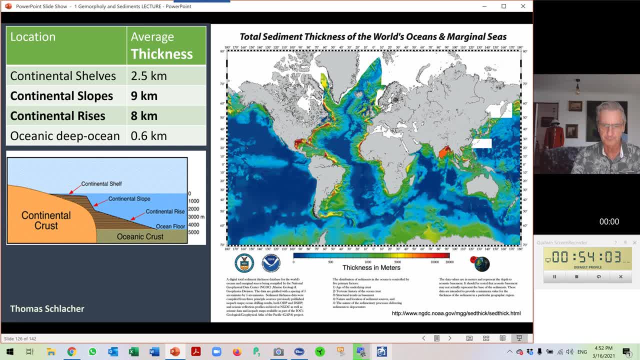 know, uh, ocean, um, exploration products. I can, I kind of love it. so you know you have to give credit where credit is to you and we can spend hours literally just talking about this map. but what really, you know, astounds me is look at the scale here at the bottom right, sickness in meter and it goes up to 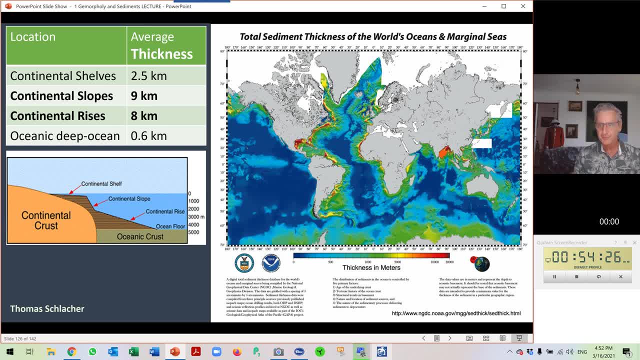 what? 20 kilometers, that's 20 000 meters of mud high, right so, and essentially the Gulf of Mexico and here the Bay of Bengal, receiving all the sediment coming down from the Himalaya Mountains, and, of course, you know, the Mississippi drains half of, uh, the watershed of the USA and Canada. actually, that was my, was supposed to be my road trip this. 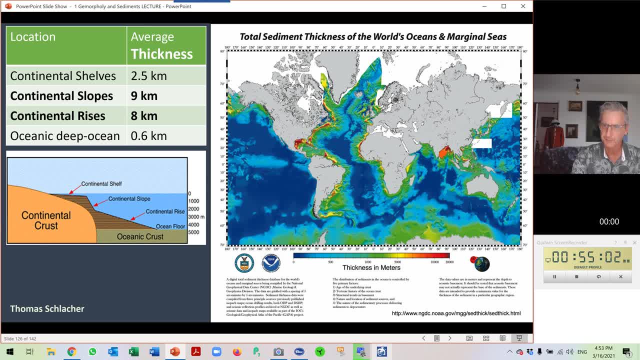 year driving in Ford F-250 from the headwaters down to New Orleans. but let's do it next year. we do two or three, can't wait anyways. and essentially over millions of years it just filled those basins up. they used to be quite deep and now it's a muddy pool. now, if you actually cast your mind back when we talked about the topography, 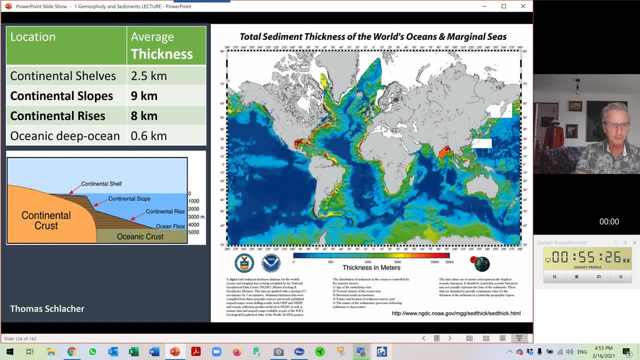 of the oceans, the ABC of geological features. we said, well, the continental crust sticks a little bit into the ocean and then it actually drops down deeply and that slope environment is called the continental shelf. and then the slope and the rise. now, not surprisingly, most ocean sediments. 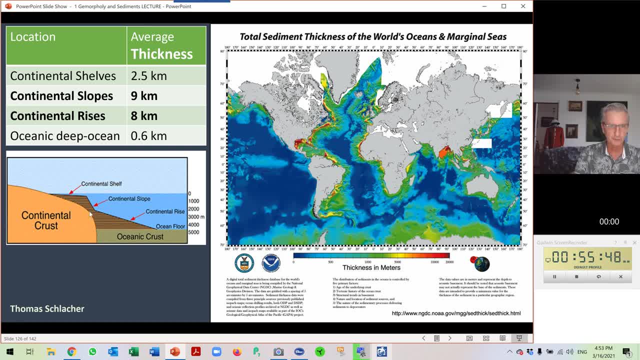 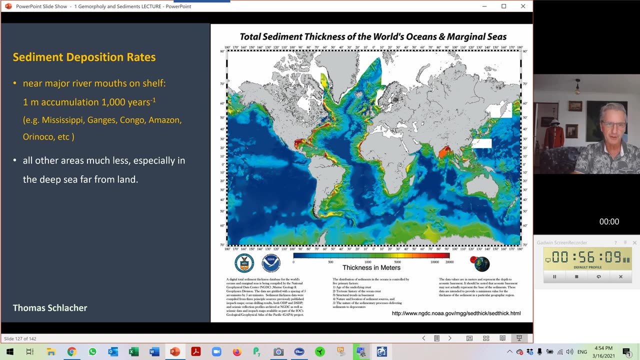 you know that came from the land- start to accumulate here. some of them- actually the clay particles that go all the way out to the middle of the Pacific but basically down here. they're talking about eight to nine kilometers on average average of mud. I think that is just astonishing. so the accumulation rate can be up to a meter of mud per thousand years. 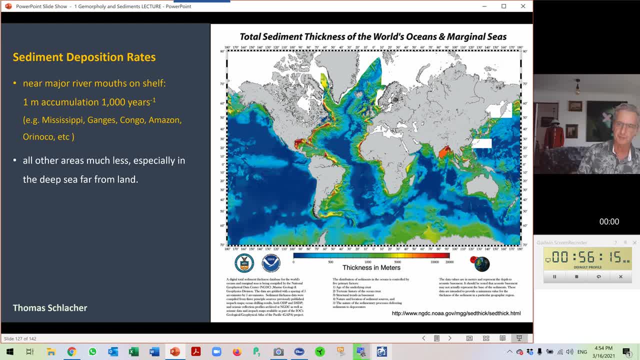 which, basically you might say this is not terribly much, but in geological times that's just massive, it's just extraordinary. and of course, if you look around this chart of the oceans, you can actually see well where does it come from. it's the major rivers: the Mississippi, the Orinoco. 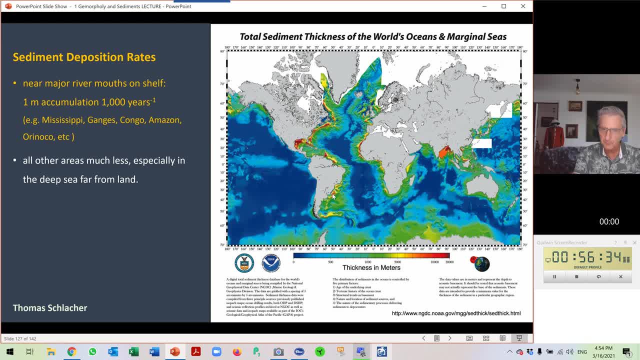 the Amazon, the Mar del Plata, the Del Plata, the Ganges, Brahmaputra and, of course, a little bit here in Europe. this is actually stuff which came off from the Sahara. you can actually see it right here. it actually comes out from the Niger River. that is comes out actually from the 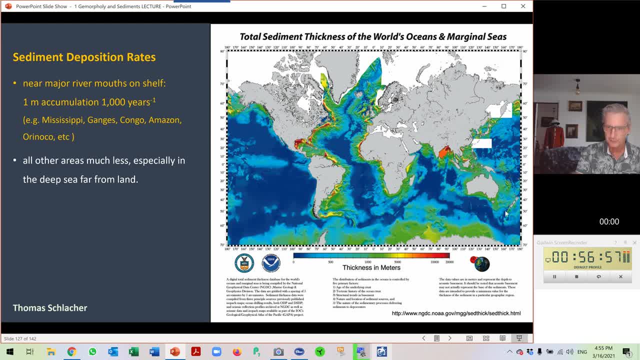 Nami Desert, and that's the Congo. hey, Australia, uh, has anybody ever- oops, has anybody ever- noticed that we seem to be in a permanent drought and hence our contribution to sediment around is nothing red, okay, fair enough. so, essentially, if you go very deep, uh, very far. 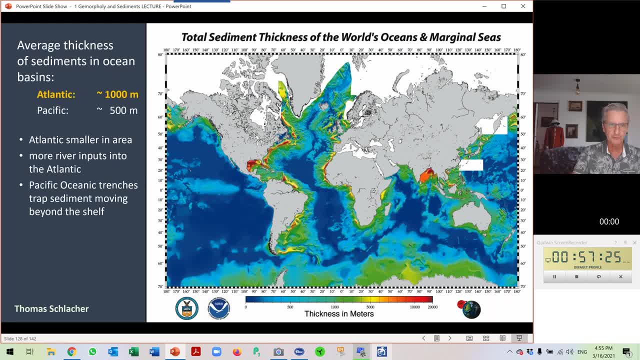 away from land. of course it gets less and less. the Atlantic has about double as much on average, simply because it's surrounded by more land in close proximity and there's more rivers flowing into it. also in the Pacific, if you recall, you've got this big Ocean Trenches sitting just basically offshore from Japan then 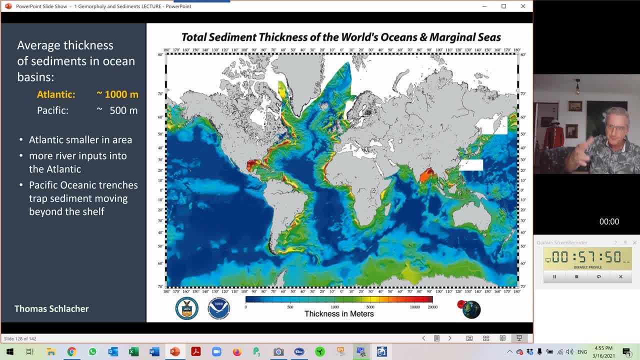 going on an island arc over Fiji, Tonga, coming down uh, towards New Zealand, the Tonga Kermadec Trench, and then we got the big Chile Trench just off Chile. so all of those actually, you know, act as a gigantic sediment trap before it actually has a chance to move out into the middle of the Pacific. 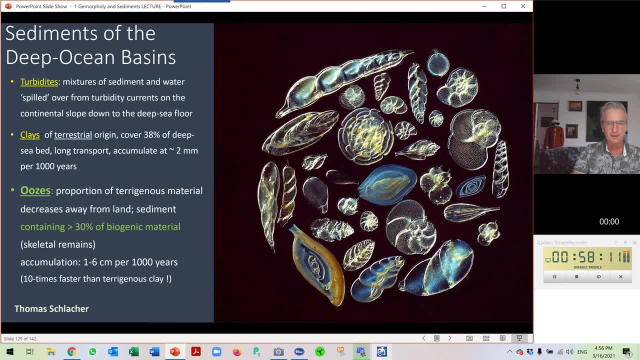 still. there is quite a lot out there. now let's have a quick look at some of those ocean biogenic uh sediments. there's a little bit of very fine clay which can travel thousands of kilometers and that covers a big area. but it's often not very sick, but still, you know. 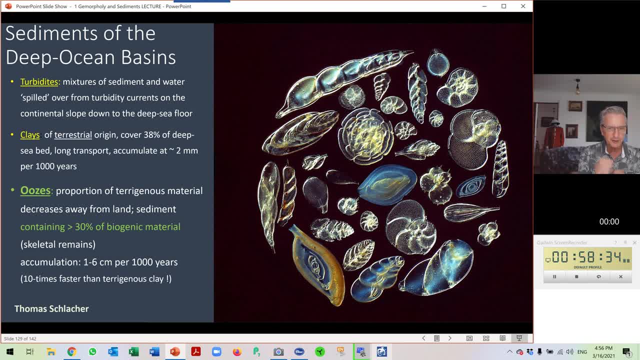 no part of the ocean is ever, ever isolated from the influence of land. let's just be clear about that. so when people say, oh, it's in the middle of the Pacific, no, no, no, you know, everything is actually ultimately connected in one biosphere. but what really is the cruising are the oozes and it's. 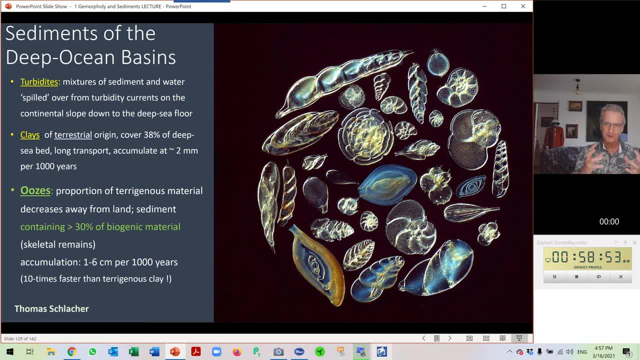 very, very hard to explain what the feeling is when you first get your hands into Deep Sea Melt, which is made from oozes. It really is oozy, uh. it's also very cold, usually like four degrees, you know, or even colder, but it really is. 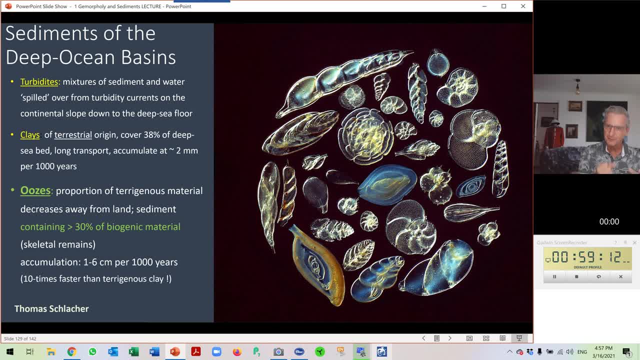 this kind of oozy material. it's kind of slushy but it feels kind of nice at the same time, although it's very, very sharp when your fingers swell up because all the little skeletal material goes in and it accumulates at a great rate of up to six centimeters per thousand years. 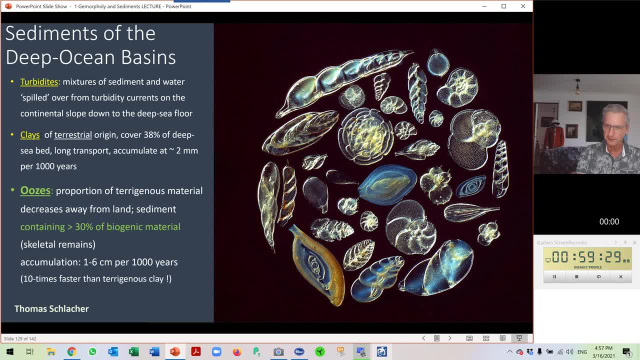 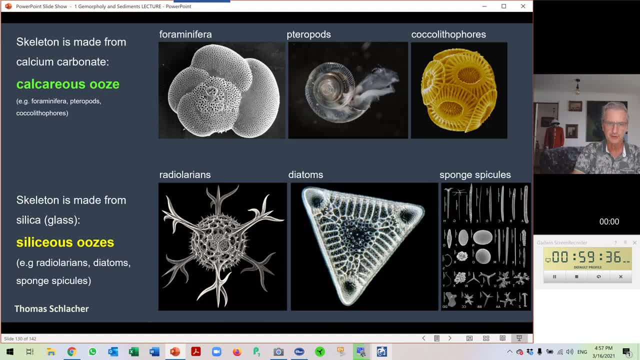 that is actually an astonishing rate, and it's all dead organisms in the grass cilia and falling down from the sunlit areas. now you might come across, you know, those kind of dirbs, whether it's a calcerous ooze or a silica reviews, and it basically just means ooh. 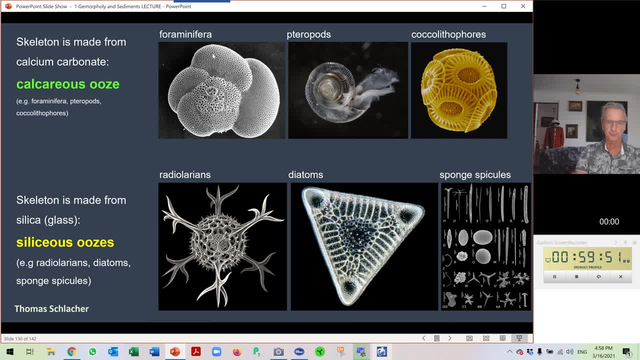 easier. skeleton made from limestone, then you're one of those culprits here. always it made fun glass, then you're one of those carpets. here Now, forams can be very large. We talk about pterobots in a second and coccolithophores Radiolarians are. 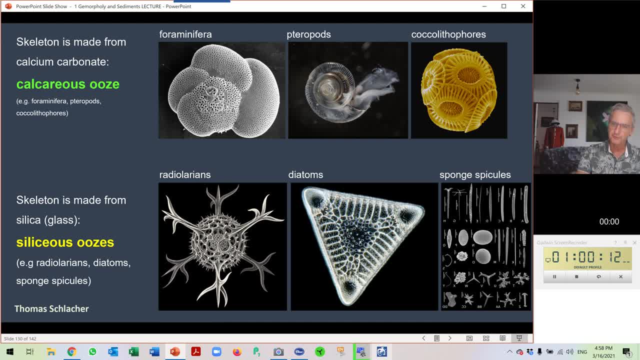 basically tiny little phytoplankton cells of sorts, I have to say, made from glass, and so are diatoms, And here those are the skeletal structures of sponges, But it's mostly radiolarians and diatoms when it comes to the glass-like you know. 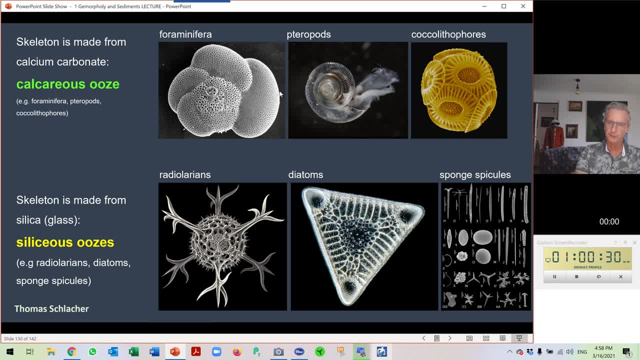 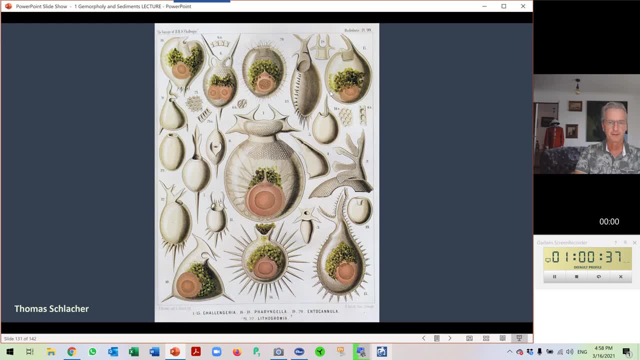 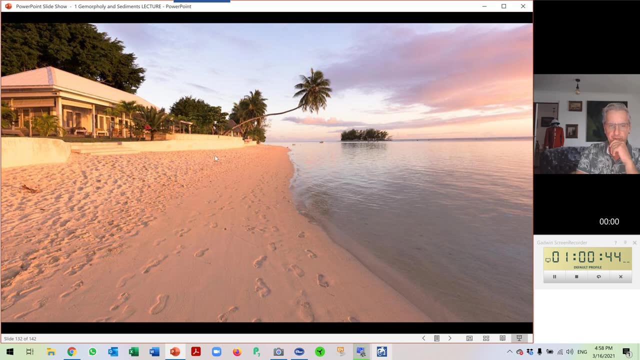 oozes and forams, pterobots and coccolithophores. when it comes to the limestone ones, Now, what are those strange animals here? Hmm, Now here's radiolarians. and before we get to one of my favorite animals, next time you have a chance and you go to a. 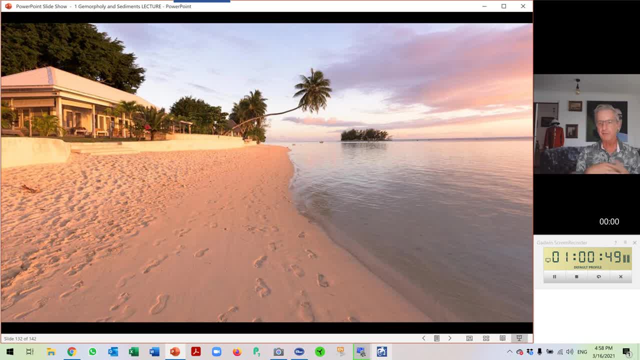 Pacific island and go there. I mean it's the most loveliest of people and they really need every single tourist dollar, Don't? I mean I shouldn't really say don't go to Bali or don't go? 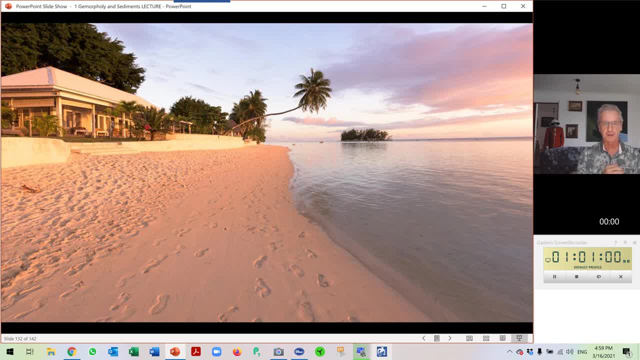 to France. but I think if you really want to make a difference- I think you know- to people's real livelihoods, go to some of the Pacific islands. You know I lived for two years in Fiji. It's quite astonishing and you do not actually. 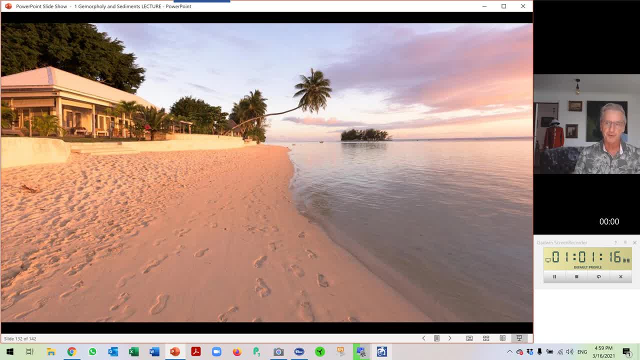 realize how far, if you spend it wisely on some of the smaller islands, in these Davis locals, how far every tourist dollar goes into in terms of educating their kids and buying medical supplies, that kind of stuff, Just when the, when the borders open again go And then buy as many cocktails from the. 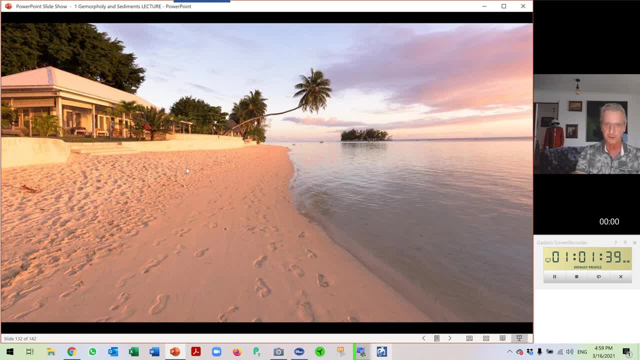 locals, as you possibly can basically wet behind your gills And what would be as orange juice or mineral water. Don't buy coconut water unless you know it comes from a small grove, but never mind, And as you actually put your hand in. 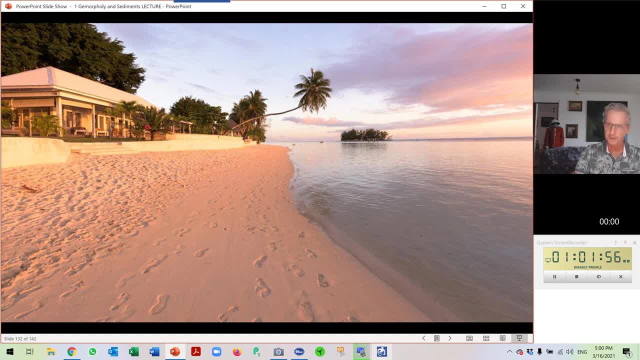 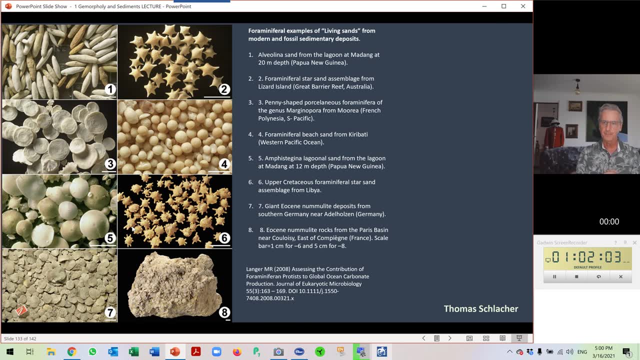 to the sand here. you might actually notice it's actually a lot coarser than is on our beaches here, And have a close look. Often it is coarse because it's made up of gigantic one-celled organisms. Those are some of the largest cells you 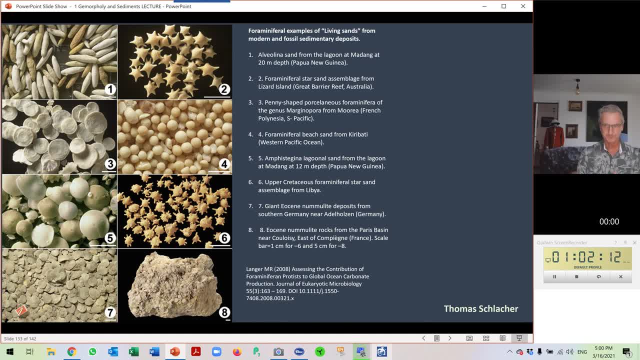 can find in the blonde and animal kingdom. It's a bit of a debate where those you know unicellular organisms should go, but I think that's irrelevant really. And there can be stars, so they can be those little you know, almost like a rice, but quite often actually you find these big. 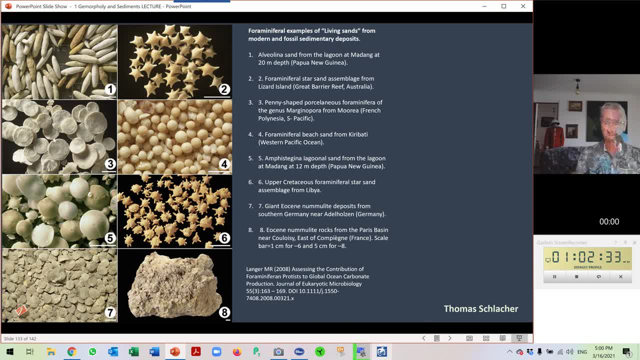 big discs and it's a single organism and they make up the sediments on those cells. specifically. guys, just something to do. you know, if you have no romantic date on the speech, you might as well study for a minifera. you know that's quite sad, being a marine biologist, you know. so the date: 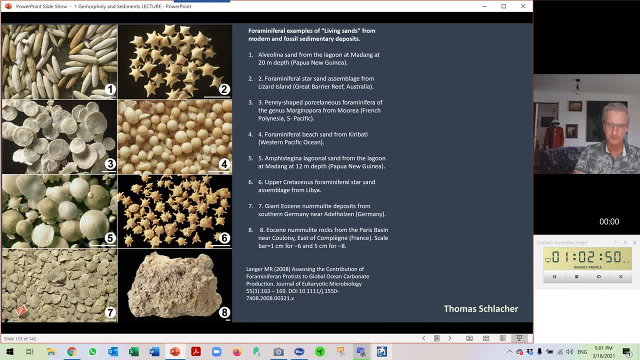 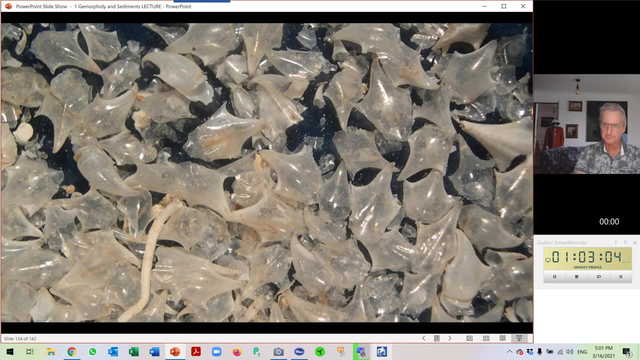 you can always look at for a minifera. yes, here we go right on that set note and look how big they are. this is actually a matchstick here. i think it's fantastic and it can have stars and blah, blah, blah. but uh, my very first deep sea sample. i put my hands into- oops, into, uh, the mud. 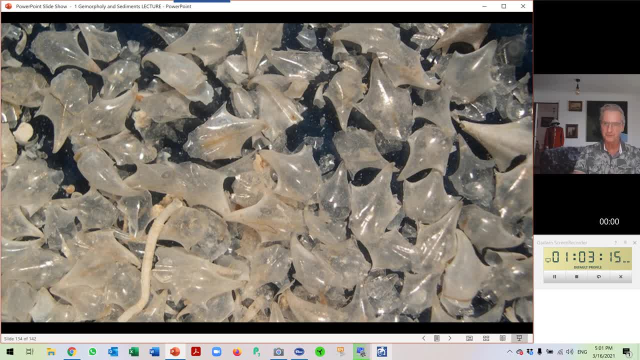 and then the next morning i could hardly move my finger. they were like big german sausages and millions of little, basically spines, buried themselves because they all broke off as i handled the mud. like those things broke off and you get little inflammations and stuff. 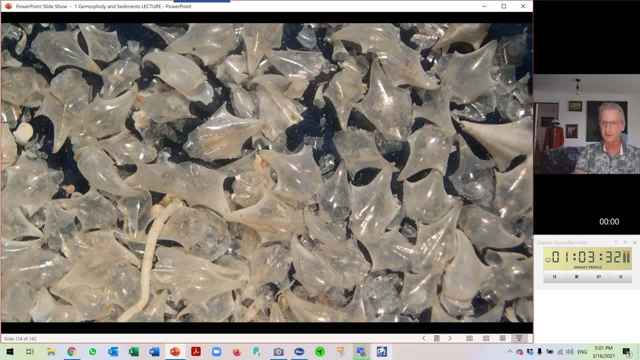 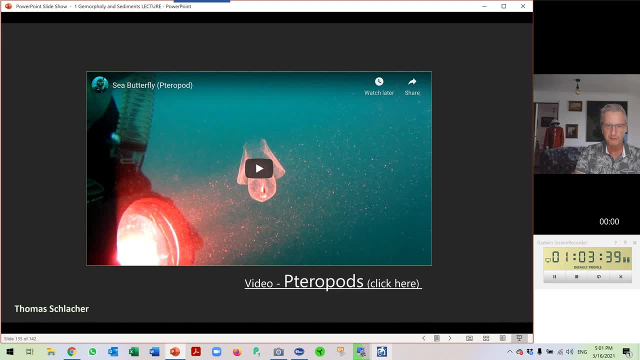 like this, which is lovely on it, both in the middle of the pacific, but never mind. and i thought: where the hell does this come from? and they come from what i think must be my favorite animals. they're called the sea butterflies or the sea angels, um. 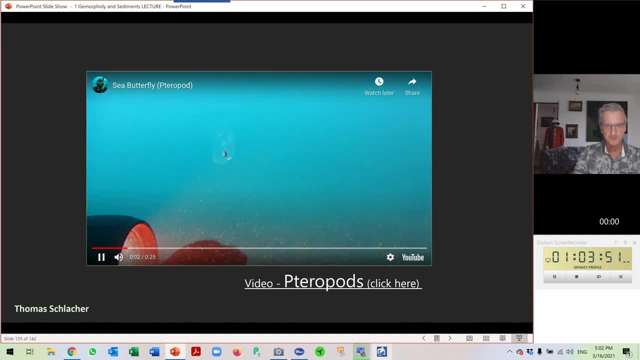 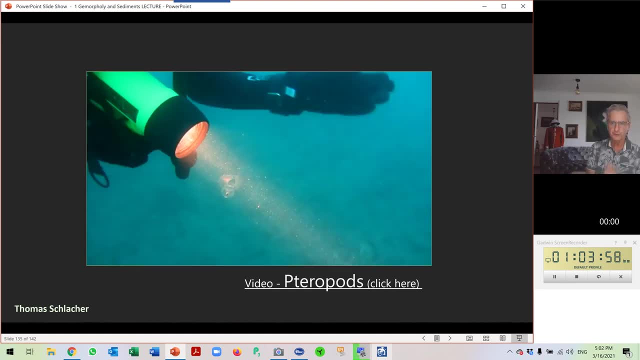 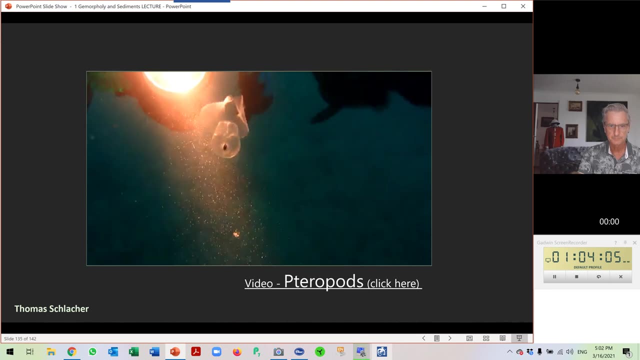 now, the sea butterflies are like this and it's actually this translucent animal. it's quite large and you think, like what the hell could it possibly be? uh, you see them occasionally and you see there's a little bit of dark structure. it's probably the stomach of the animal, so they 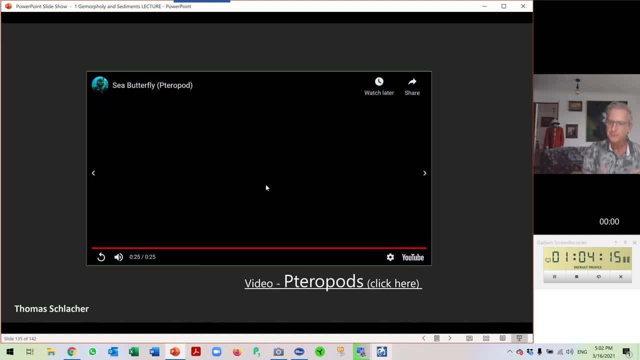 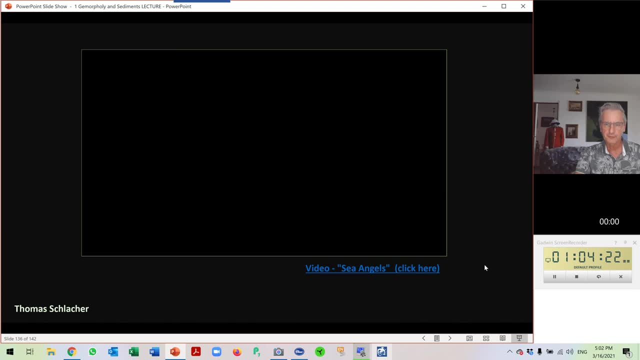 just ate something. but all of that is just like this floating, and it's not a jellyfish kind of thing. i mean, it's probably like a jellyfish and they're moving on the other side. so this is very interesting. so what could it possibly be? now i'm not clicking on this one. 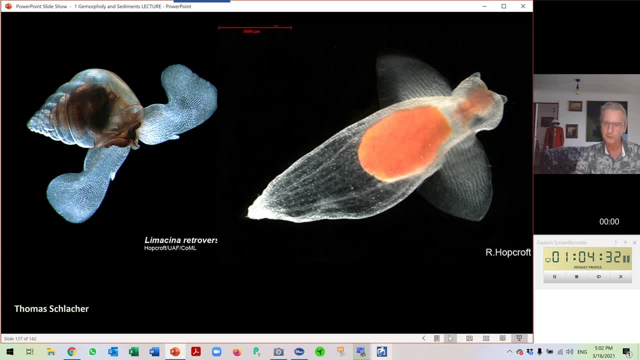 it is simply because of copyright reasons, so it doesn't upload onto youtube. you got the link in your lecture notes or just just google sea angels. it's fantastic. now what actually happened is you can actually see it from this particular fellow. here you can see the. It's a very small, very translucent, very fine, very delicate shell, because it has to. 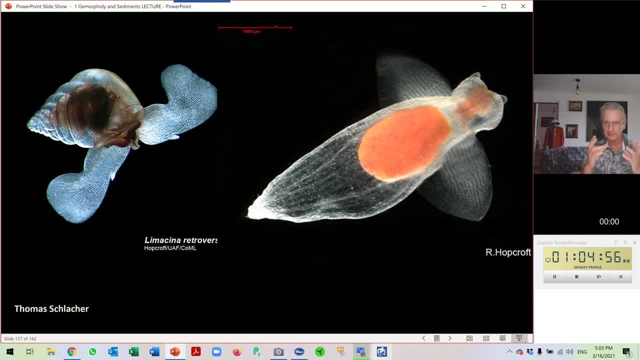 be very light Because there's a group of snails who decided I completely hate it just being this kind of snail thing. I'm kind of slimy. I've got a bit of a shell at the top which is quite heavy. 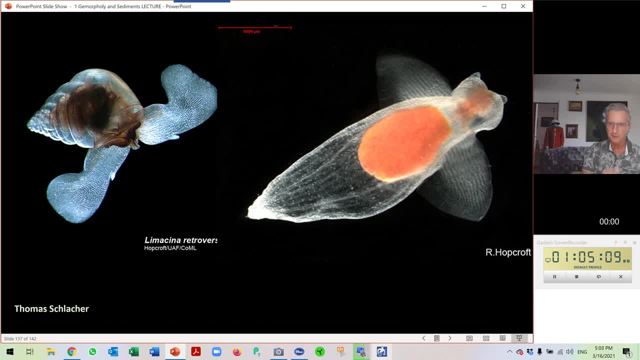 Sometimes the French come along and they stuff me with some garlic behind their gills and drink red wine and eat baguettes with it. But this whole snail business is just really, really mundane. It's very pedestrian. So I want to actually be free. I want to be like a bird in the ocean. I want to be like 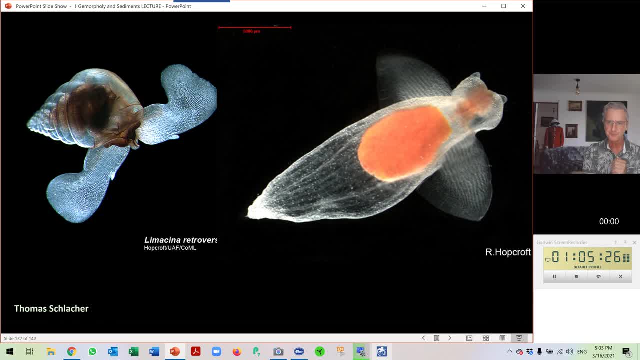 a fish. I want to be like you know something beautiful. So evolution has kind of- you know, the evolution theory has kind of listened to their beliefs for being a little bit more glamorous or a lot more glamorous, And what actually happened was they transformed their foot into rings. 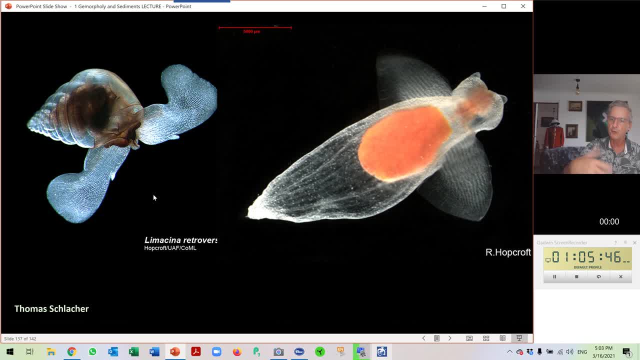 Here we go. That's why they're called pteropodes. They're ringed feet, so to speak. They reduced the shell, but that little bit of shell which remained is the skeletal remains which sink to the bottom of the ocean and make those oozes which can be very, very. 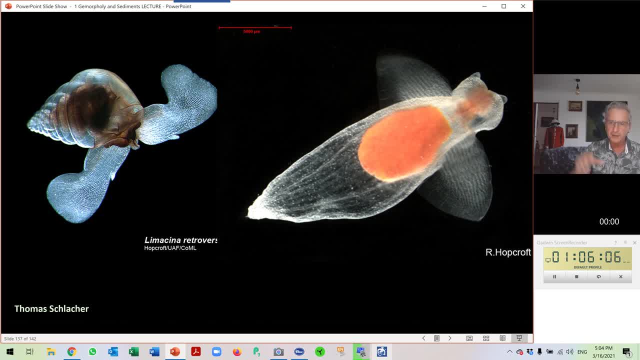 prickly. But the really cool thing is it's actually snails flying through the water. I mean you can't get any cooler in zoology. I think they are the number one cool invertebrate. And go and Google on YouTube pteropodes or sea angels or sea butterflies. 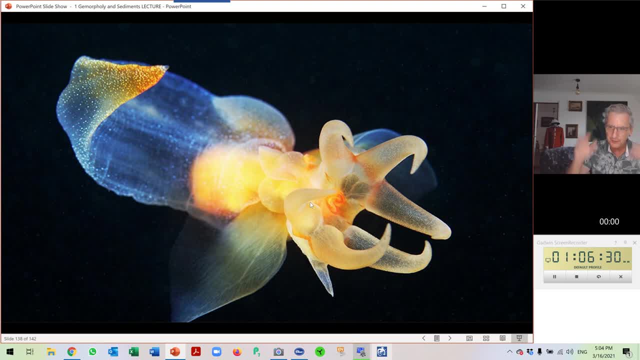 I think it's fantastic. And look at this guy. I mean the colors. and then he developed these little arms and there's a little jaw. I mean, compared to you know, any other marine snail, this is like cool stuff. 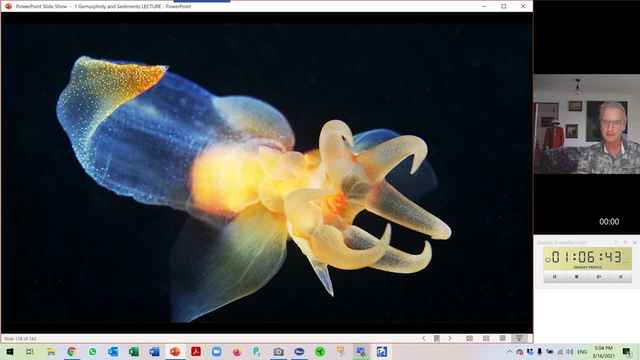 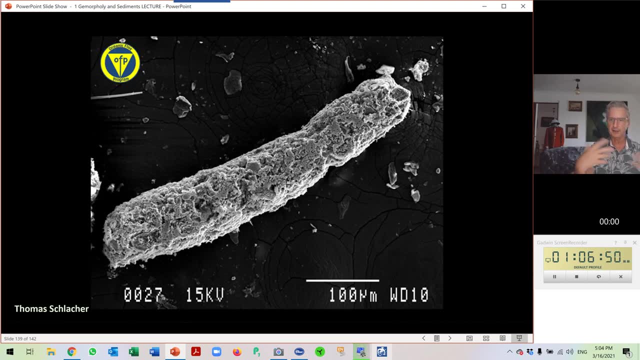 Now going from the really, you know, aesthetically Incredibly pleasing stuff to that now, when we still could lecture in big lecture theatres, I said, well, what is that? I'm not quite sure, And there would always be one or two kids who are not all that polite. 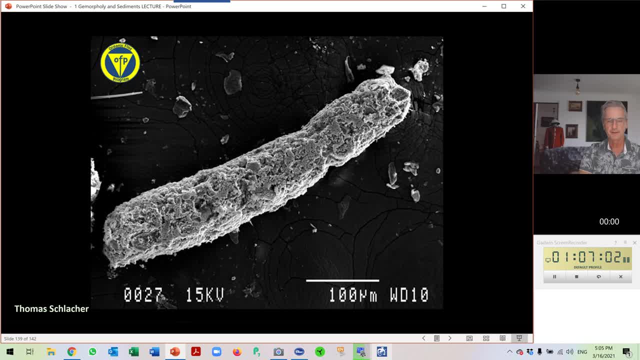 And I would say that's a turd. And yes it is. It's actually named a faecal pellet, which is a very curious term, And it's called a faecal pellet. It's called a faecal pellet. I'm trying to make a faecal pellet, but it's basically a turd. 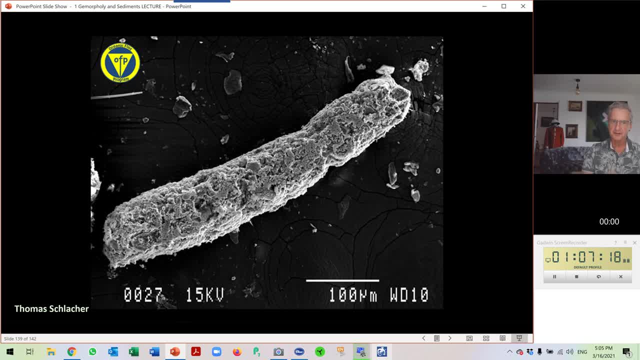 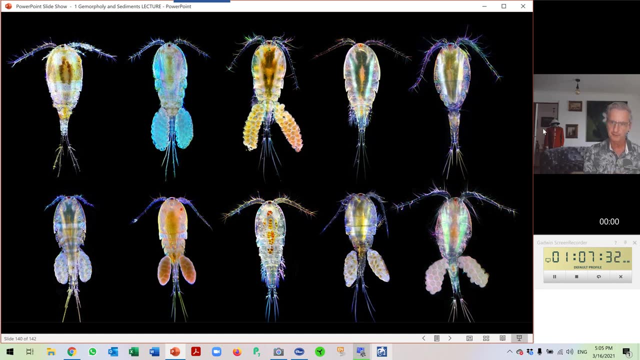 And it's about 300 micrometers long, So it's a lot bigger than really the little tiny fragments of phytoplankton which it contains, And it's a turd from those kind of animals called copybirds. Now, they really actually are that colorful, you know, if you put them under the microscope. 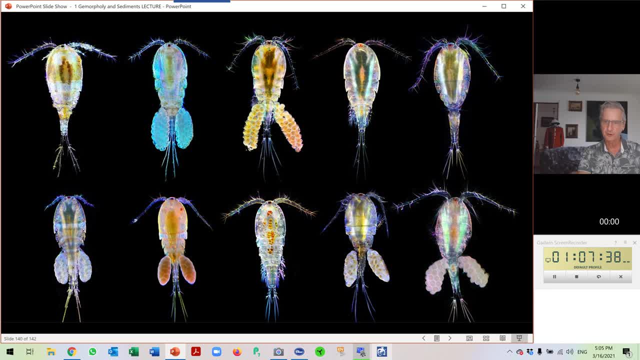 And it is said there's something like Jamie Clarkson would say on top girl. it is said that you know that Tyler Lama only has one pair of underpants, or something like this, Something ridiculous. He always says on Top Gear, or what is it now? 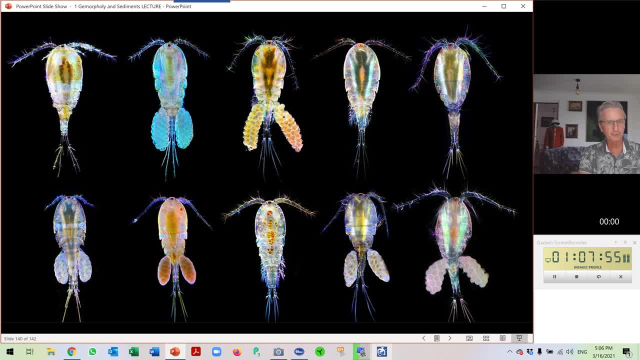 The Grand Voyage, That one particular species of copybird, that tiny little crustaceans in the plankton floating in the top layers of the ocean, is the most numerous species of multi-cellular animals in the world. So that is a turd. 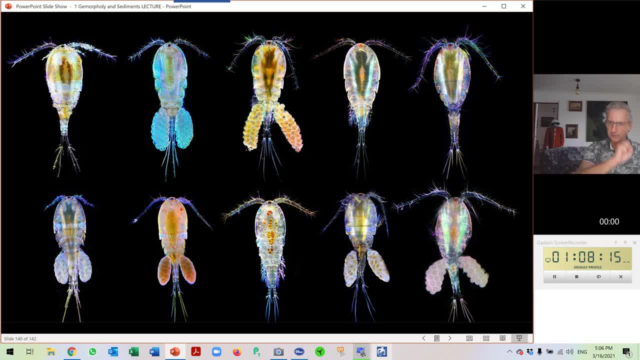 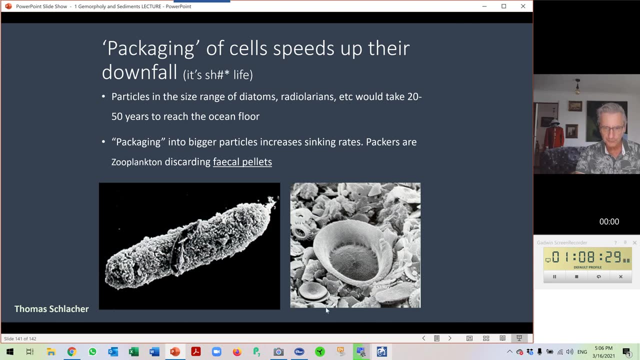 There's tons of them, And they're grazing on the phytoplankton cells, including those which have skeletons, which make sediments when they have died, And so what actually happens is we go from the skeletal remains like this: This is like a big, big circular diatom. 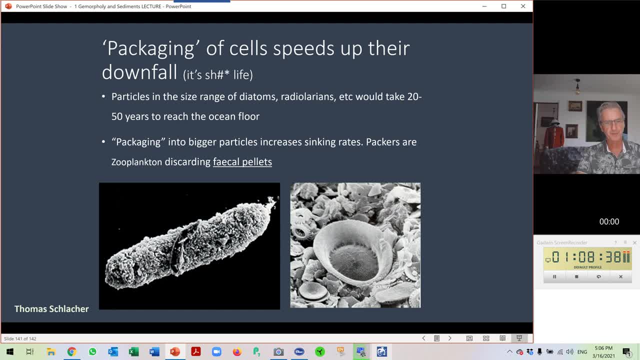 And that's actually magnified from one of those turds. And remember what I said: It would take 50 years for that surface carbon to go from the top to the bottom of the ocean. But if you have the copybirds packaging it into larger particles, ie this one politely. 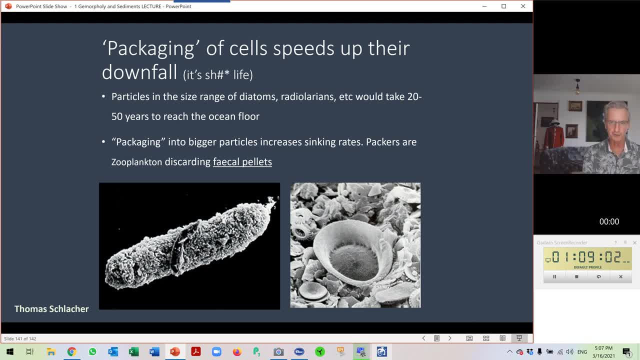 called faecal pellets. the whole process is actually sped up considerably, And this is a really cool mechanism: Tiny little crustaceans Feeding on phytoplankton- phytoplankton that absorbs carbon dioxide after it has been dissolved in the seawater, of course make organic molecules which feed the copybirds and then sink to. 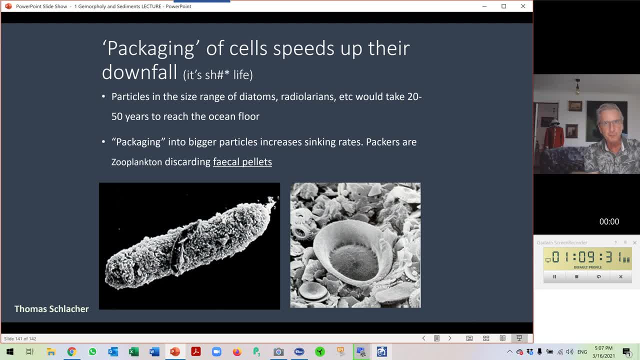 the bottom of the ocean, much of it, where it actually gets buried. This is the true carbon removal pump of the biosphere. It's not like planting forests and offsetting them And this is all. Of course, that doesn't work, because the trees rot again, just basically when they rot. 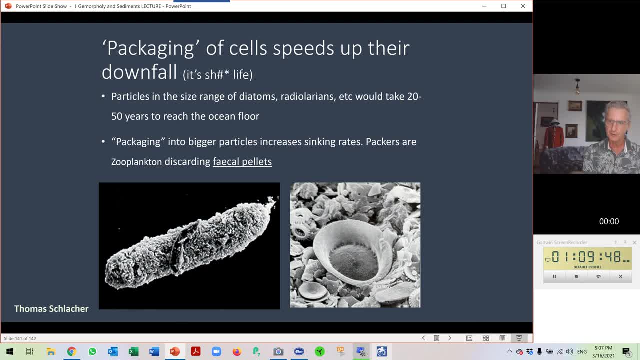 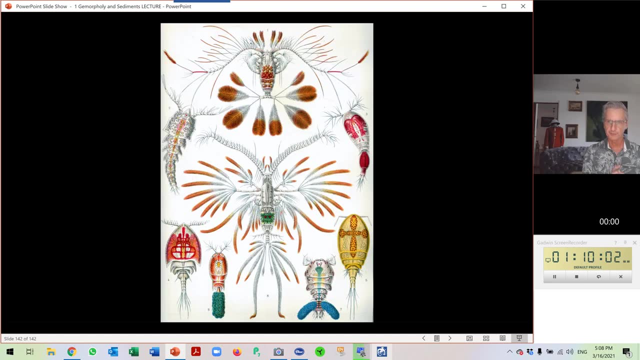 the bacteria give off CO2.. This is actually what does work And, oddly enough, a key process is a turdy one. However, I can't leave you with that kind of impression, So I leave you with a few drawings of those copybirds. 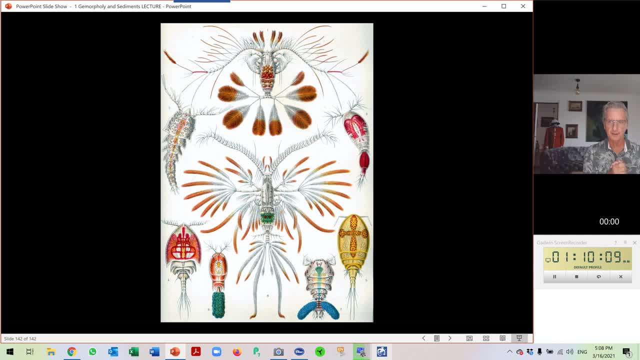 And this is not a guy who actually has you know this kind of thing. This is a guy who actually has you know this kind of thing. This is a guy who actually has you know this kind of thing. This is a guy who actually has you know this kind of thing. 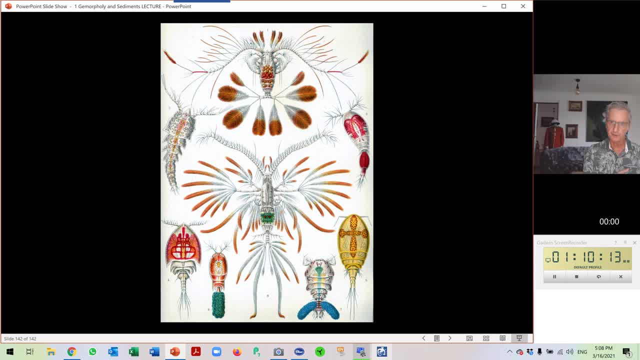 But this guy is actually covered in new drug supplier of some really, really cool stuff. This is a German illustrator at the turn of the last century And he really actually saw copybirds exquisitely like that. So there is beauty in turd producing crustaceans in the middle of the world's oceans, making